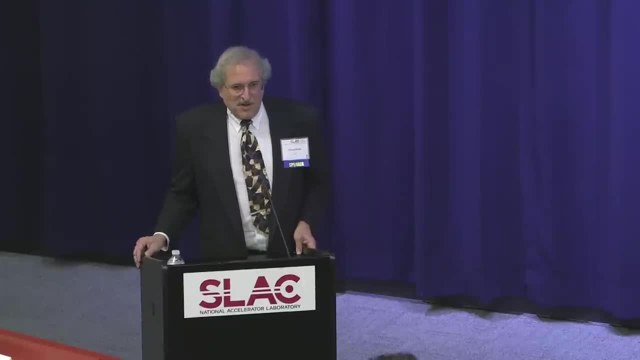 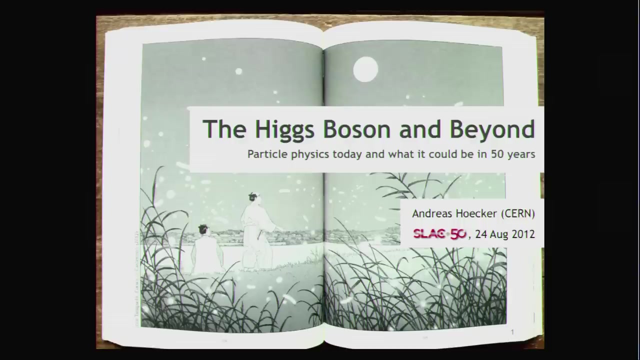 of the Orsay Laboratory and also he is now the convener of the supersymmetry searches group in Atlas place to survey what the terrain is now and what will happen in the next 50 years. So let's welcome, Andreas. Thank you very much, Michael, for this introduction. 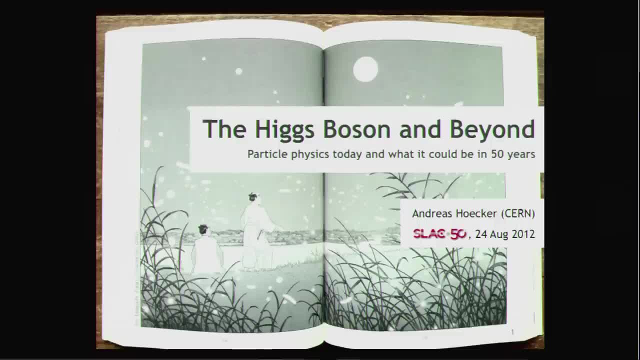 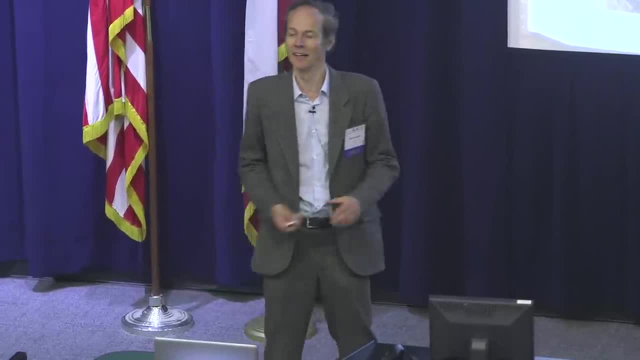 I'm really excited, a bit nervous, and I'm very honored to be able to talk to you here about this very particular moment for SLAC and also for particle physics, of course, As you know: the completion of the Standard Model and a model to which SLAC has so decisive. 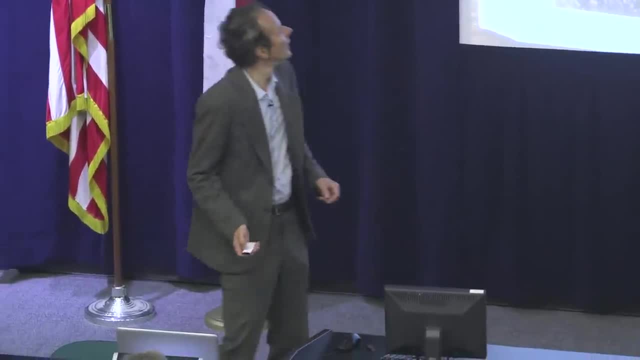 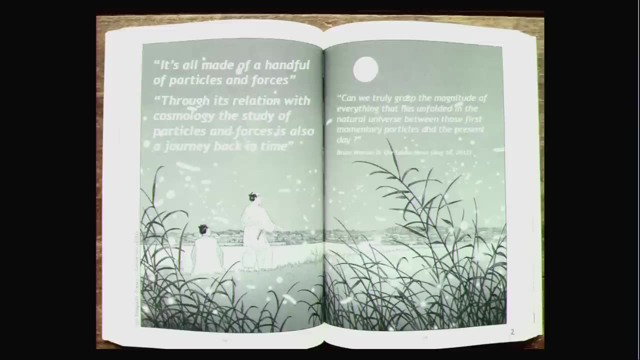 contributions throughout the many, many years, And so most particle physicists believe that it's all of us. everything is made out of a handful of particles and forces, And so we should really imagine the creativity of nature to create all this out of just particles. 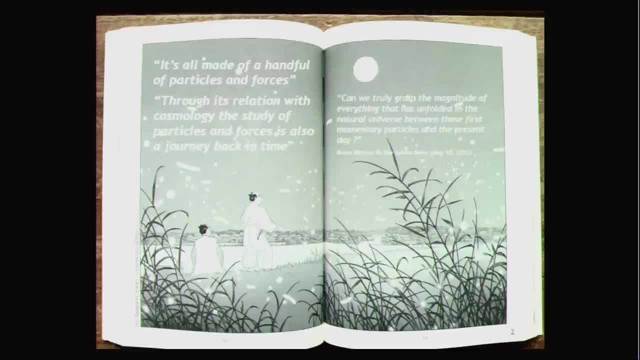 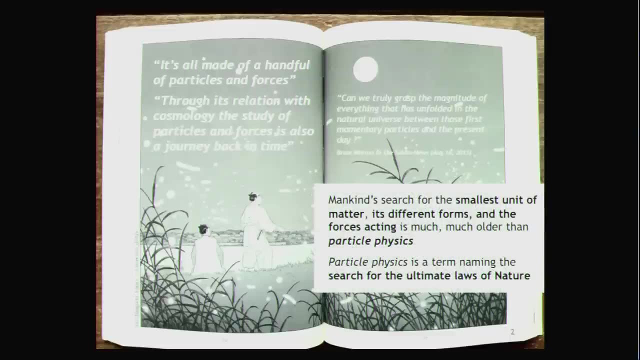 and forces, And through its relation with cosmology, the study of particle physics is also a very important part of, of course, the journey back in time. Now, mankind's search for the smallest unit of matter in its different form of the forces is much, much older than, of course, than particle physics itself. 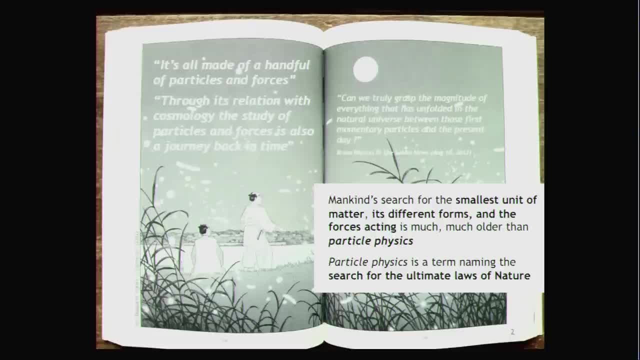 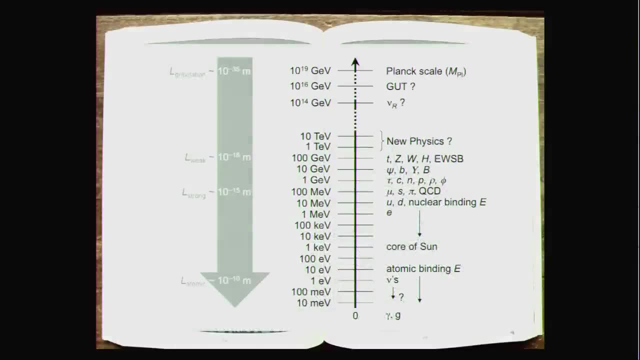 And particle physics is just a term for the search for the ultimate laws of nature. Now I would like to show you just quickly, as an introduction, the scales of particle physics. And so I don't have a stick, so I will try to make big movements. 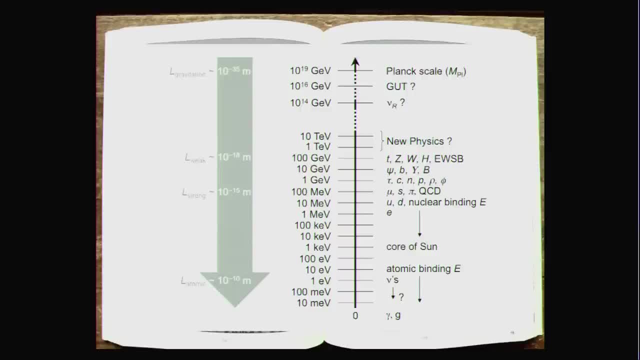 And so if we look Very big movements, we need to get to this high energy here And we see an antropoportionality between energy and distance. So in order to resolve very, very small distance, we need a lot of energy. 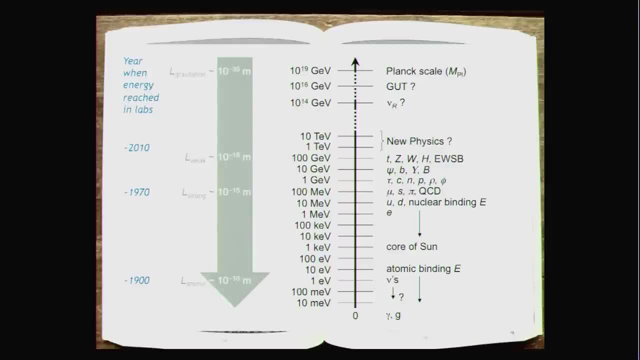 And throughout the time we see here. in 1900, we were able to resolve the atomic scale. At 1970, we were able to resolve the QCD scale And now we are really fully resolving the electroweak scale with the Higgs boson, with. 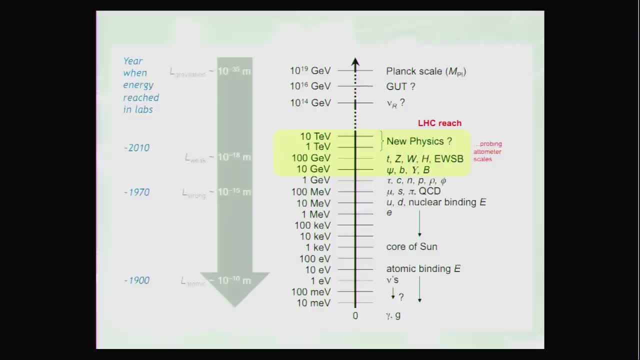 electroweak symmetry breaking And we hope then, of course, additional particles coming up And if you just look at the pattern, there is a good reason to have additional particles coming up just beyond the electroweak symmetry breaking scale. 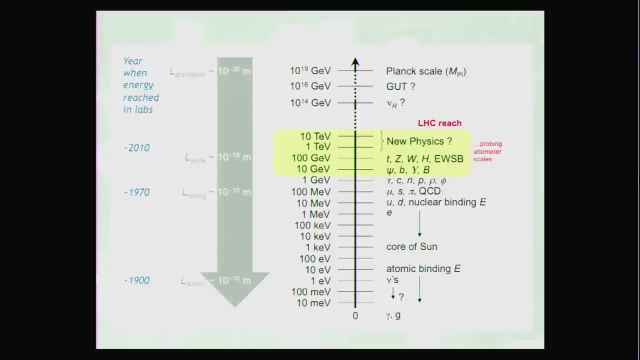 And then we don't know what is happening. We have a few hints. what should happen, For example, at very high energy, gravitation becomes strong, And so we expect certainly new physics to come in there. We expect also there is grand unification of the forces of the order of 10 to 16 GV. 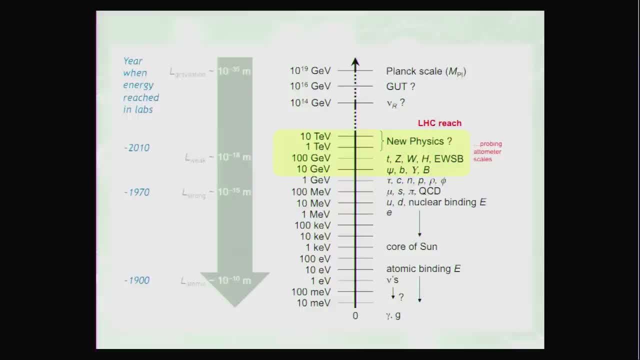 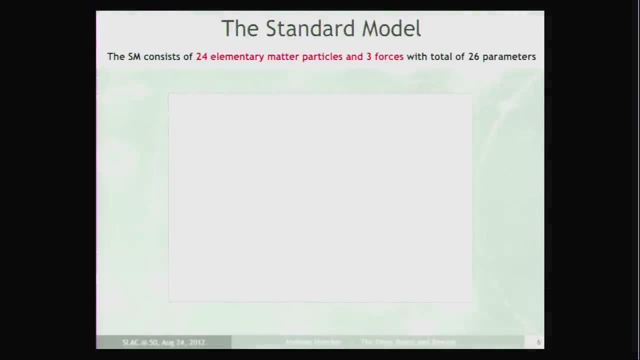 But what we are now really concerned about is this: 10 to minus 10 seconds after the Big Bang, the TEV scale. So if you've got, Yes, So we want to compare nanoscience, of course. oops, sorry, very, very small. we have seen. 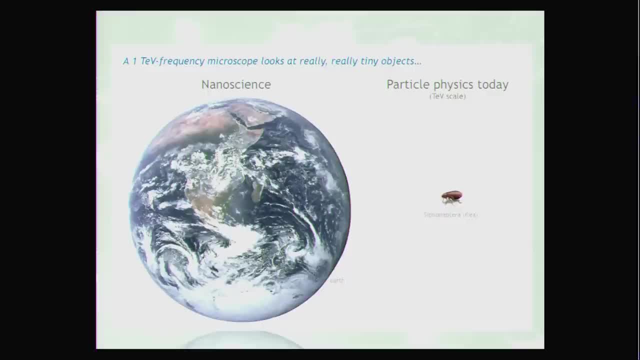 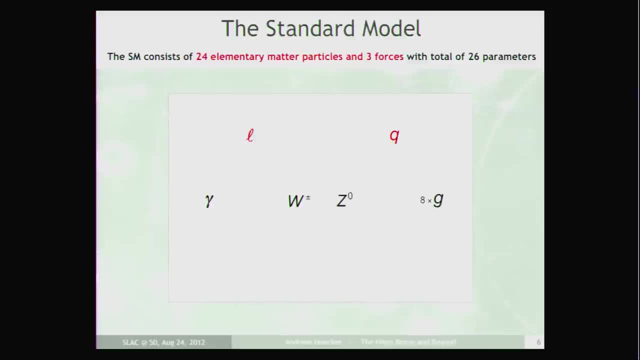 And if you compare the TEV scale with nanoscience, we compare a flea with the size of the Earth. The standard model consists of 24 elementary matter particles and three forces and a total of 26 parameters. at least it could be 28,, including the nocelo masses here. 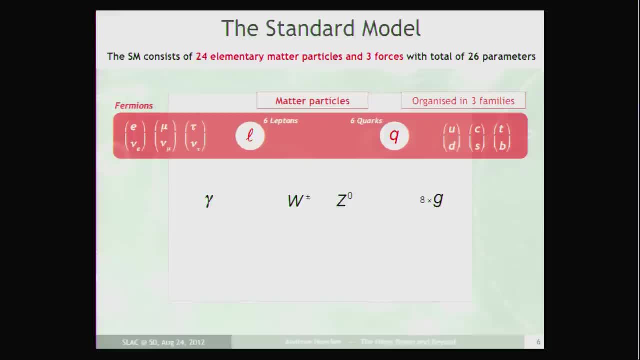 We are organized in matter particles, organized in three generations of leptons, And then we have the force quanta, where we have the photon for the electromagnetic force, the W and Z bosons for the weak force and the gluons for the strong force. 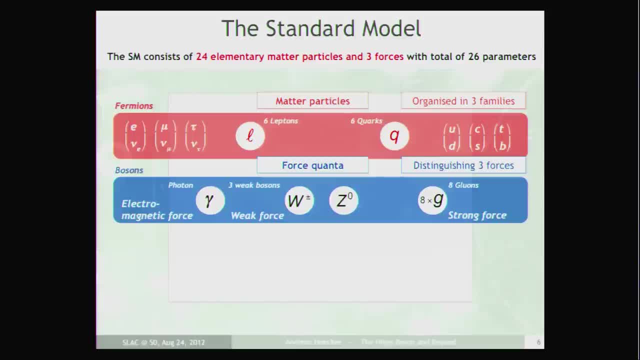 And the electromagnetic and weak force are actually unified in an electroweak symmetry, an electroweak interaction, And at the vacuum, at our energy. the symmetry is broken by the Higgs particle, which also generates the boson and the fermion masses. 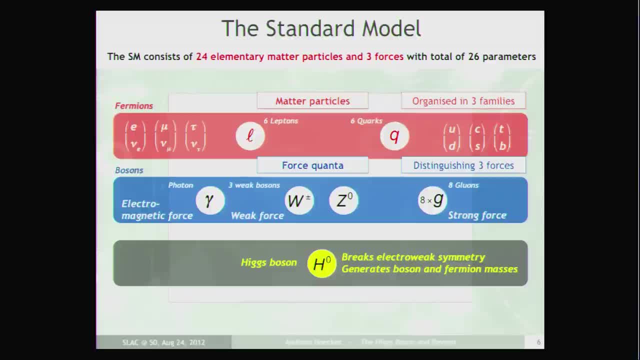 And this is a very important problem. It's a very important particularity because of gauge invariance. In fact, gauge invariance is a very fundamental principle, a geometrical principle, which means the invariance and the local space-time transformation, which is very important to 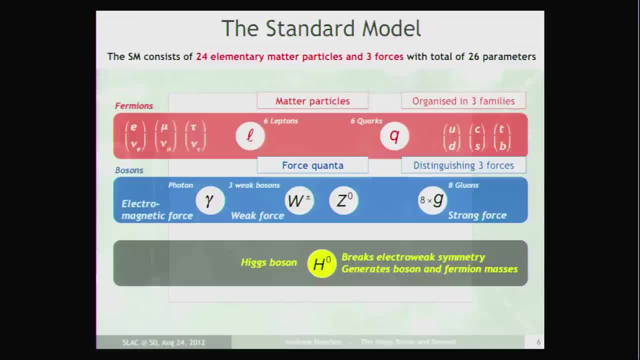 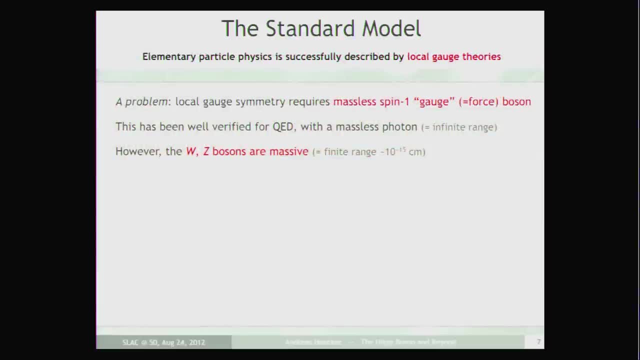 because from this principle we can derive all the forces in the standard model, and even gravitation from this geometric principle. So we don't want to give it up. but in fact there's a particularity in gauge invariance. It means that all the bosons and the fermions should be massless, and this certainly is. 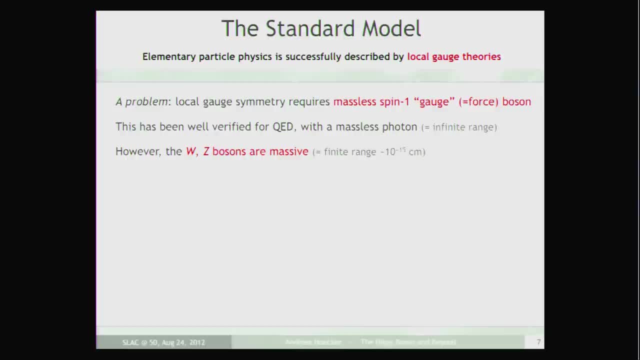 not the case. So we need a trick to give them masses without breaking gauge invariance, and the trick is spontaneous symmetry breaking. This is something which nature has done already in other areas, For example. you look at superconductivity, for example, where the Cooper pairs in the 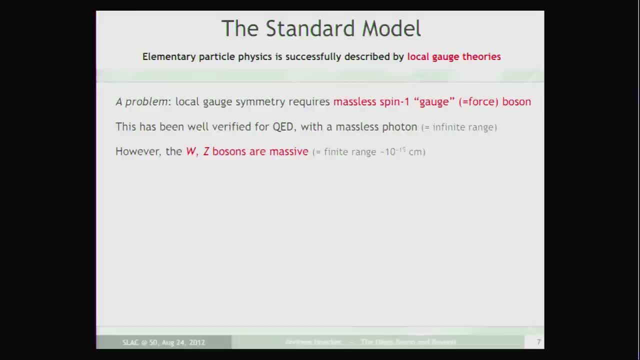 superconducting phase give mass to a photon, So this is quite similar to the Higgs mechanism here, And so, in order to break symmetry consistently, we need to introduce a new field, which is a doublet, in fact a doublet complex field with four parameters. 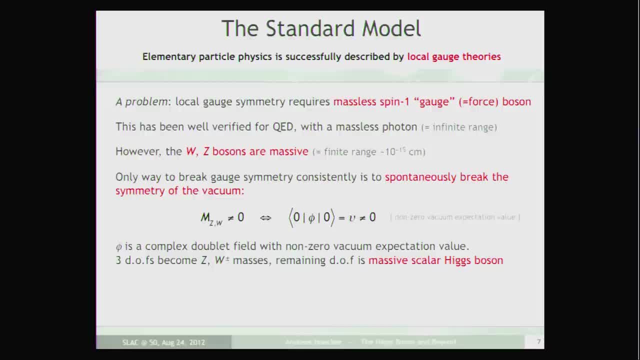 And we need a potential For this field. So the four parameters after: if you use judiciously the potential, the four parameters will be eaten up by the masses of the W and the Z boson and a single parameter is left, which 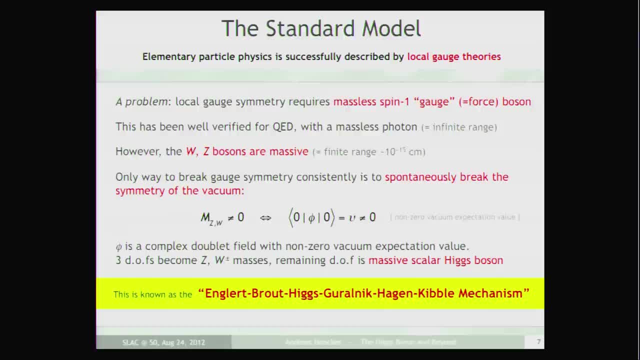 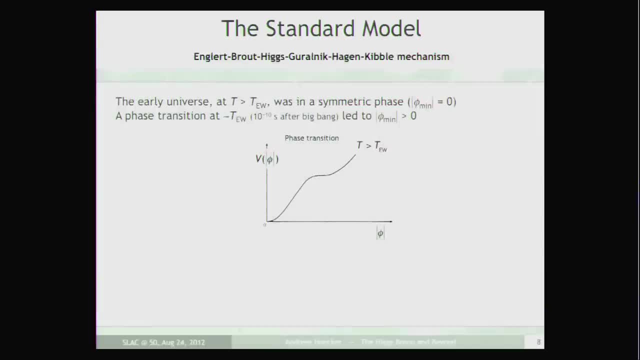 is the so-called Higgs boson, And all this together is the Englert-Brute-Higgs-Guralnik-Hagen-Kibble mechanism. We will short-term this Higgs mechanism, And so we should look back In the early universe. we have very high energy. 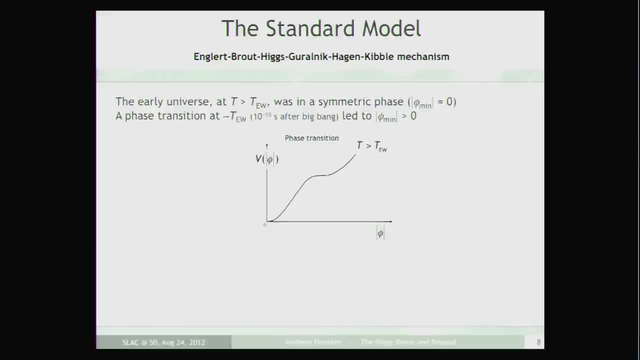 We are above the electroweak symmetry breaking scale. The electroweak interaction is unbroken And we have a potential of this phi which has a zero value at the origin. So we don't have any breaking of the symmetry. 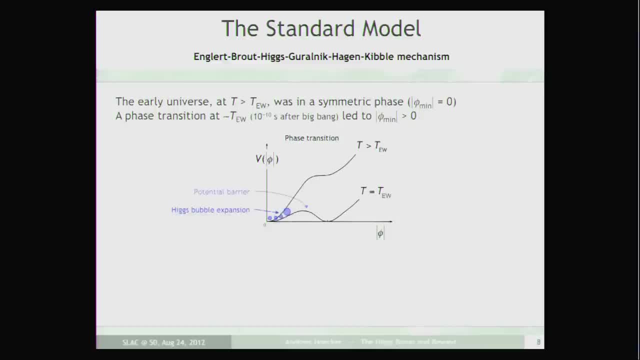 Now the universe expands, It cools down And we pass through the electroweak phase transition, which is actually very fast: Higgs percolates and bubbles, And then finally it comes up and builds a vacuum expectation value. so a non-negative value. 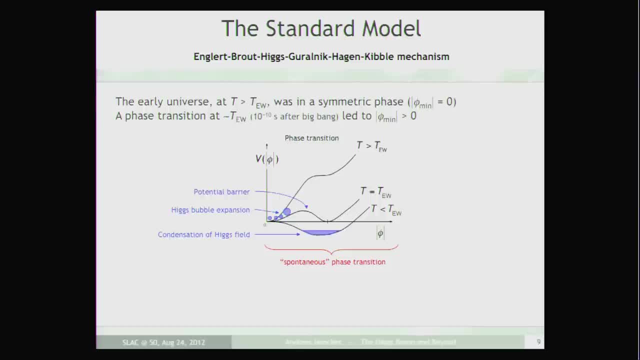 at the vacuum, at the zero, It's the zeroest energy And the potential to describe this could be, for example, this term: It's the simplest term for a scalar potential of this type, with a mu squared term, a lambda. 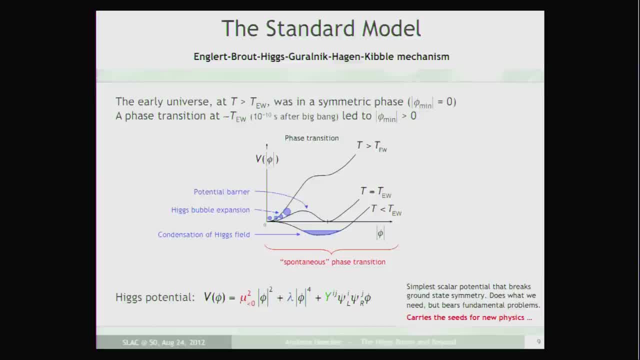 term to the order of fourth and then some term which gives the Fermian masses, And this term has to be negative. This is an important feature, So this gives this feature here. Then lambda has to be positive. Goes up here And in fact we want that. 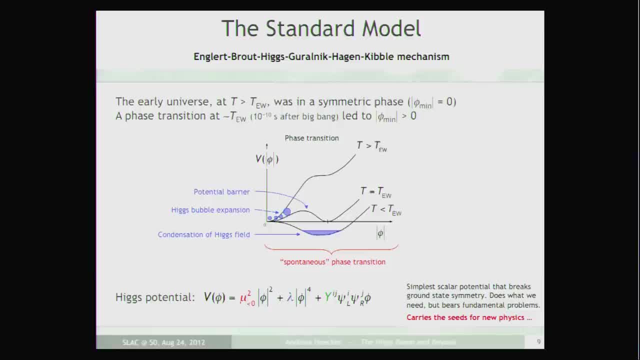 Yeah, so in the standard model this term gives the mass of the Higgs- and this is directly then also described proportional to the mass. So if the mass is too large, lambda will be too strong. This is a self-interacting term. 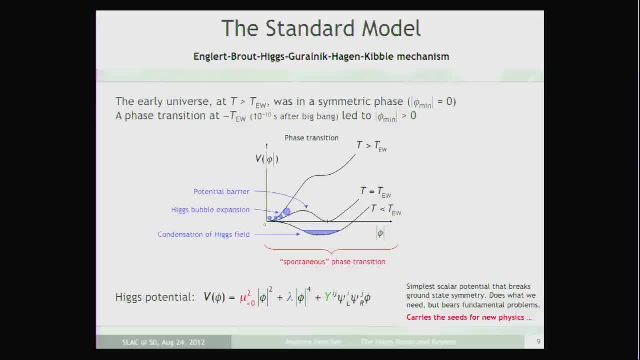 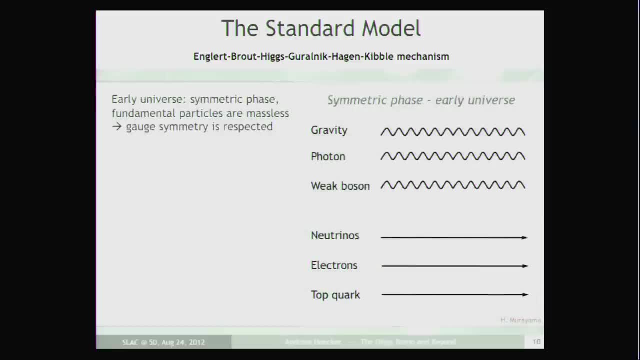 If the mass is too small. in fact, this potential might have another minimum and might be unstable. So this would be an unstable electroweak minimum. So this is a very, very important feature. So we need to- I mean, these parameters have to have the right values. 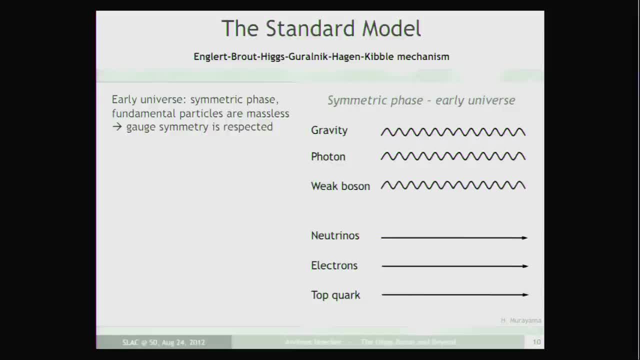 So now a little bit more imaginative. We are again at the Big Bang. We are in the symmetric phase. No electroweak symmetry breaking. All particles are massless and travel with speed of light through the early soup. Now a Higgs field displaces the ground state, breaks gauge symmetry. 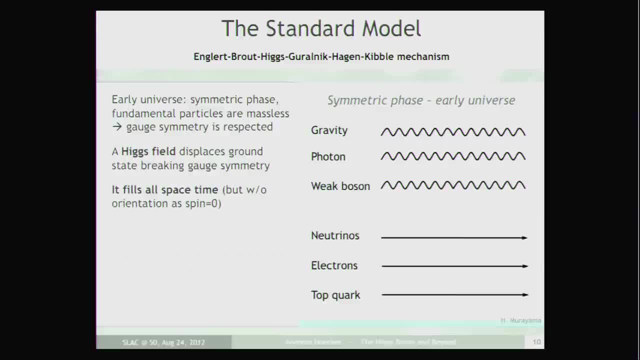 It fills all space and time, but no orientation. It doesn't have any spin And you see, that's actually very fast what's happening here. But you see, the particles start to interact with the condensed Higgs field And the stronger the interactions, the slower they become and the bigger is their mass. 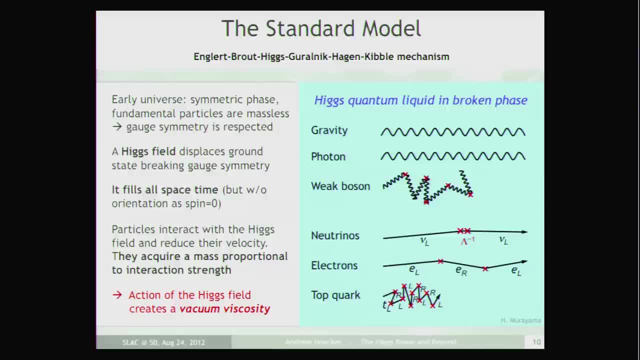 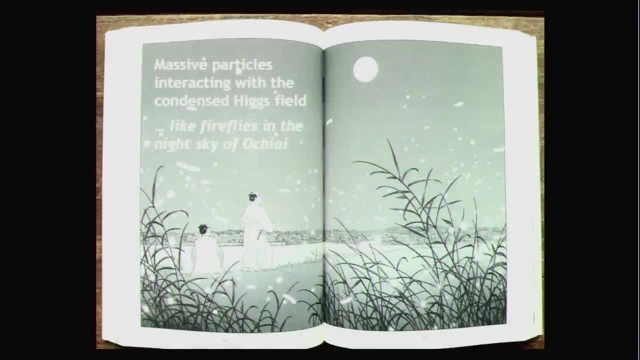 So this is the mass generation mechanism And it's really the action of the Higgs field creates here a vacuum viscosity. OK, So to introduce this picture: massive particles interacting with the condensed Higgs field like fireflies in the night sky of Oceania. this is a place close to Tokyo where you can. 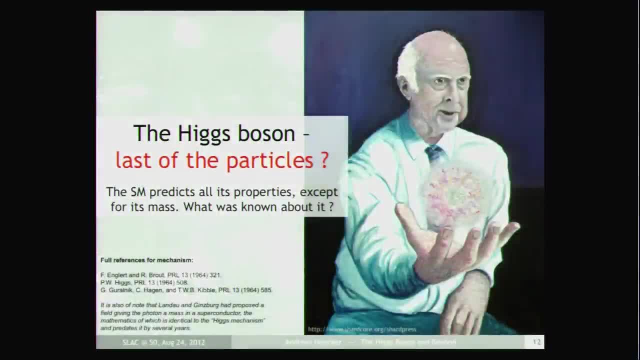 see many, many fireflies. So the Higgs one, is it the last of the particles? We actually did know quite a number of things already before it, And the only parameter which was not known was the mass And all of the couplings. everything else can be computed once we have the mass. 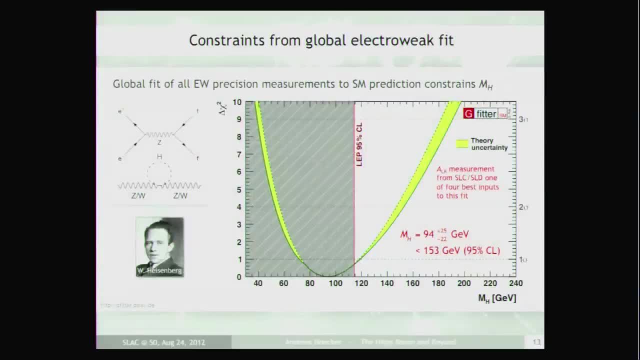 And even on the mass, from the- at that time- precision and intensity frontier, we already had quite interesting information, also delivered, of course, by the fantastic ALR measurement at. so a symmetry, thank you. a symmetry measurement at. oh great a symmetry measurement. 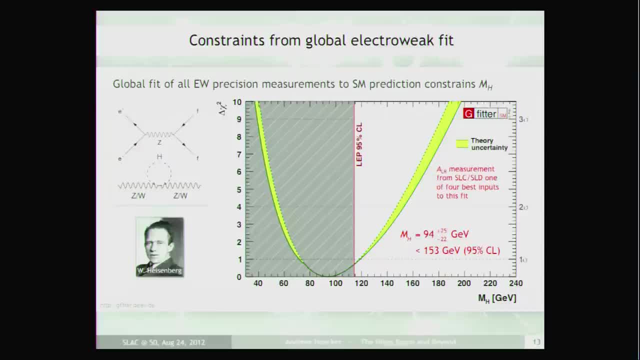 at the linear collider at SLAC, SLC, And so although these, like LEP also at CERN and the Teverton, could not produce the Higgs, in particular LEP of course and SLC could not produce the Higgs directly, they could. 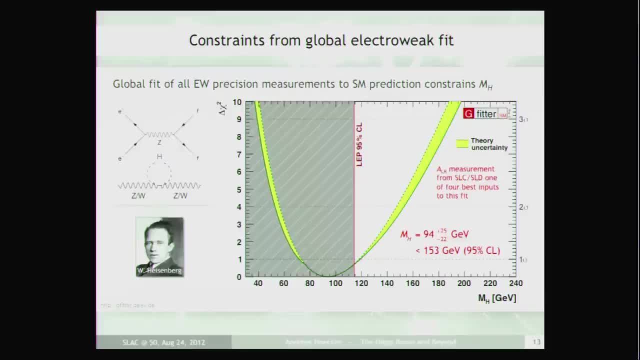 in fact see the Higgs through the uncertainty relation, through virtual production of Higgs, which does change the actual cross-sections, the asymmetries, variables, like also the W mass, which are measured, And so from a global fit of these data, it was possible to determine that the Higgs has. 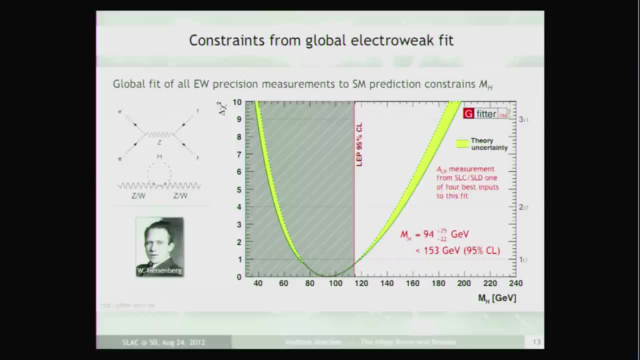 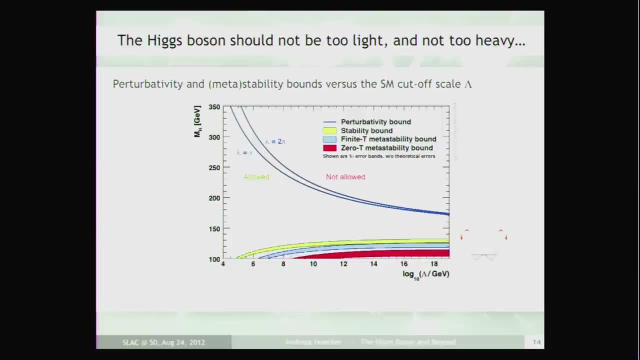 to be lighter than 153 GV. so that's of course, a very interesting information. There's another reason: Look again at this potential we have here, And the mass determines really the form of the potential. so if the Higgs is too heavy, 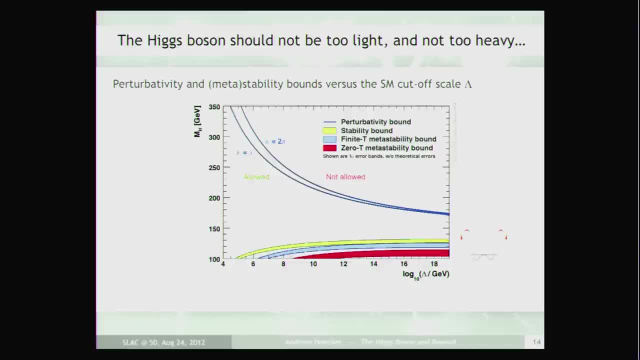 the Higgs self-interaction, We become non-perturbative. This is something we do not like. If the Higgs is too light, the potential will not be stable. There will be another minimum showing up and we might tunnel into this other minimum. 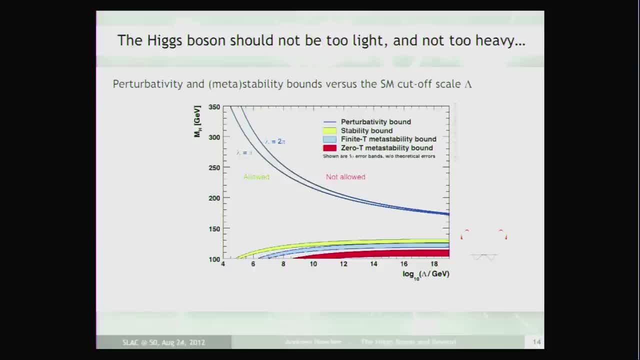 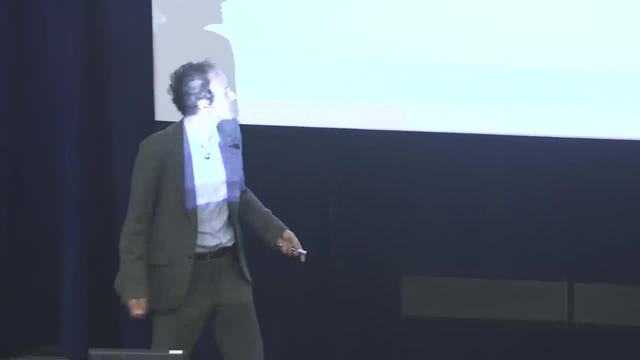 in our universe, And this is something we don't like either. And so these constraints become stronger and stronger if we go up in energy And if we go up to the Planck scale, assuming the standard model is valid up to the Planck. 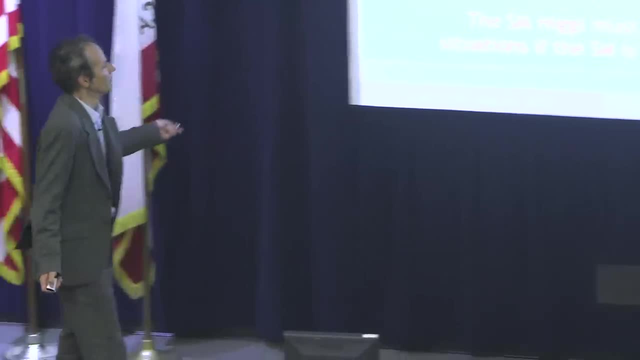 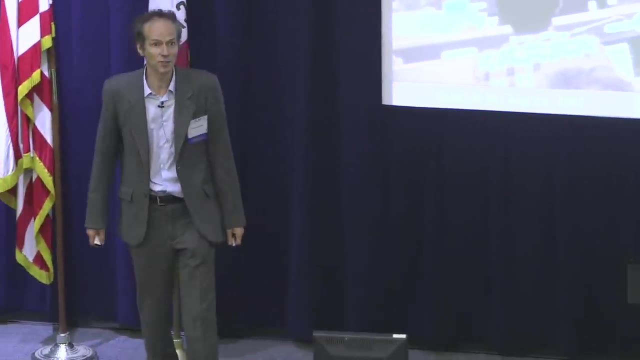 scale, then in fact we must steer a very narrow course between these two disastrous scenarios. So this was what he knew before July 4th. Since July 4th, we know much, much more. We have seen the Higgs. 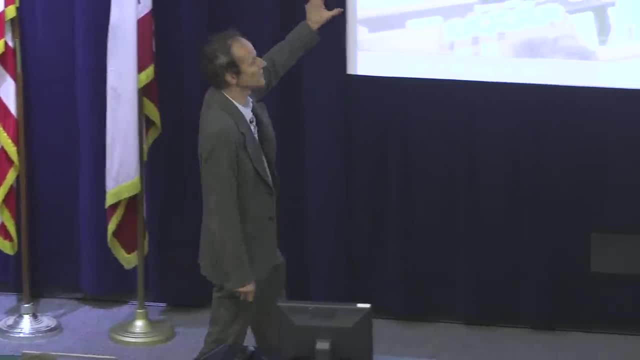 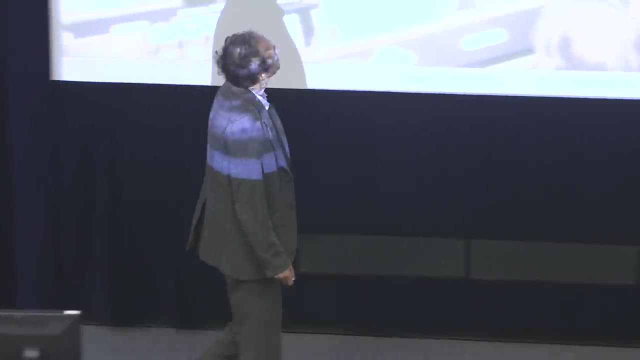 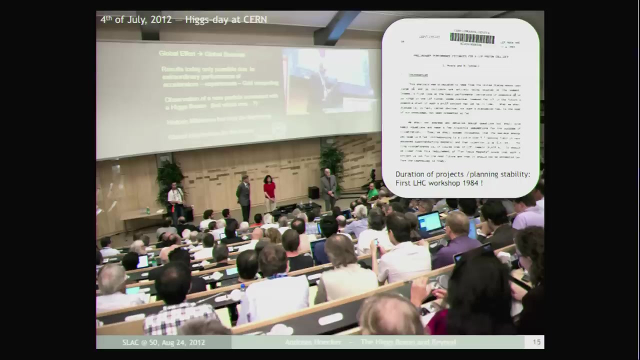 And to go this way to achieve this goal, to be at this day and to present these results was, of course, a very, very, very long endeavor, which started by a LEP node by Lynn Evans and Schnell on 83,, brainstorming the idea to have protons, proton collisions or proton-antiproton. 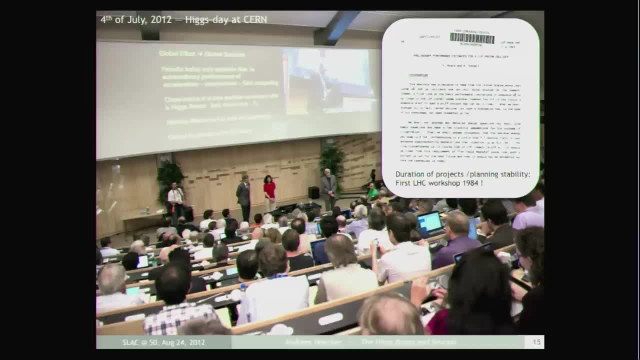 collisions in the LEP ring, And then the first workshop was in 84, so almost 30 years ago. OK, And so you assume what stability this needs and what incredible- yeah- what the people had to invest into this to make this possible. 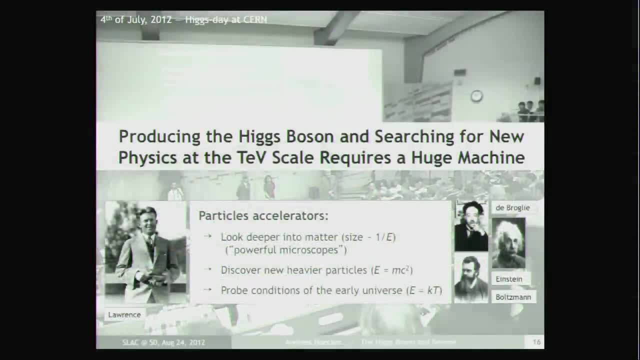 So producing the Higgs boson and searching for new physics at the TV scale requires a huge machine And we use the fact that looking deeper into matter we need a lot of energy, a powerful microscope, discover new heavy particles. We use Einstein's relation between energy and mass and probe the conditions of the early 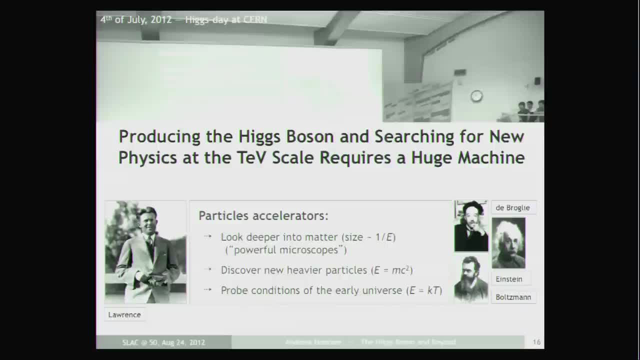 universe. We use the relation between energy and the Boltzmann relation. Then we use the trick which was introduced by Lawrence in the beginning of the 30s. That was a very, very small cyclotron. It became bigger with time. 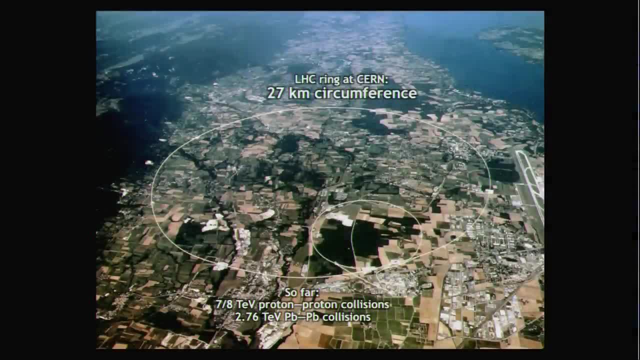 It became 27 kilometers huge, a proton-proton collider. here. This is the LHC ring. This is part of the injection chain here, CERN. There's another side of CERN here And so far last year we had a 7-TV proton-proton collision. 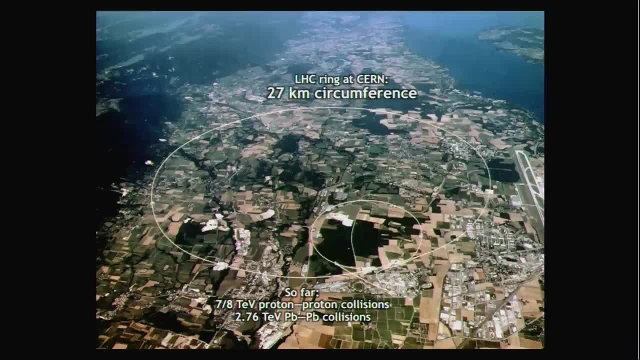 This year we had 8-TV proton-proton collision. Luminosity is in the detectors of five invertebrates. This is the LHC ring. This is the LHC ring. We have five inverse femto-1 last year. 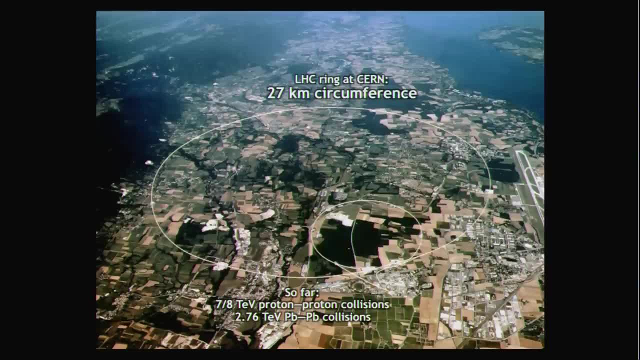 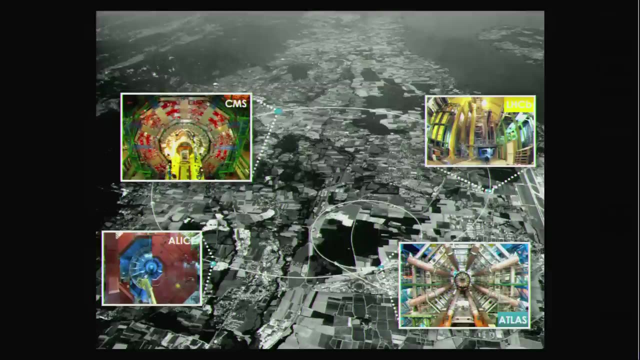 And now we have more than 10 inverse femto-1. this year The results on the Higgs were made of the order of almost six inverse femto-1 on 8-TV collisions this year. And so we have four experiments: two general-purpose detectors, ATLAS and CMS, and then LHCb for 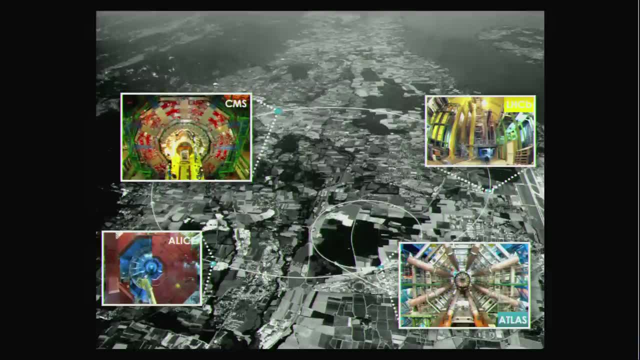 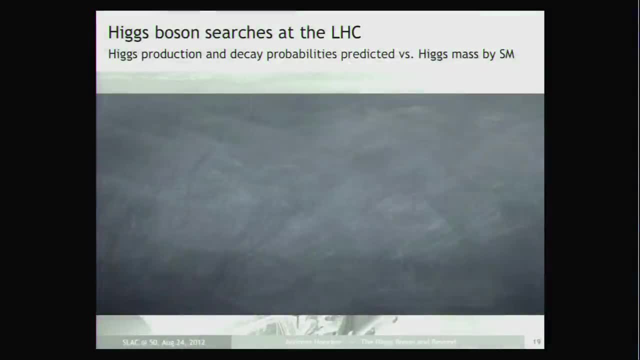 dedicated B-physics studies, flavor physics and ALIS for dedicated heavy-ion studies. I cannot go into the details of the detectors, but what we are looking at is proton-proton collisions, So we think protons, that's U and U and D quarks. 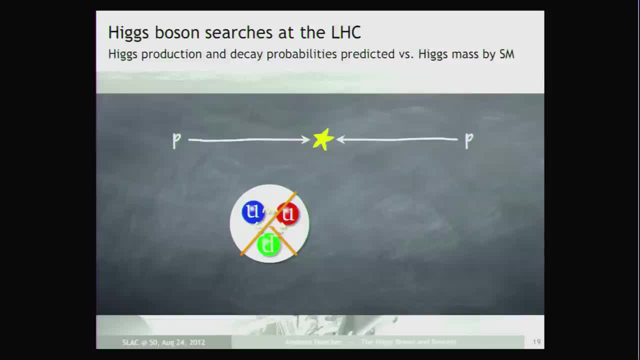 That's how protons are made, And so this is the picture we have, But in reality, of course, it is much more complicated. It's really a complicated compound wave out of protons, where we have all quarks and also gluons, and with different proton distribution. 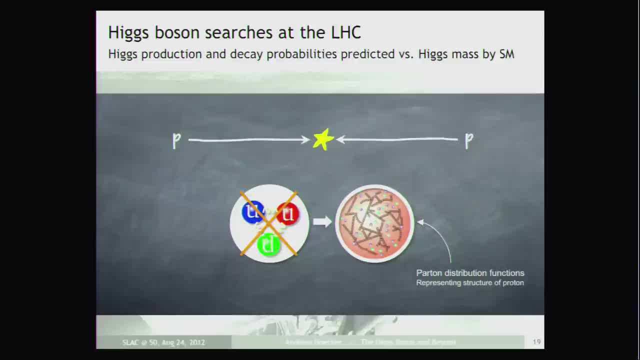 So corresponding to the momentum transfer of these proton-proton collisions you have. you have different quarks and different protons contributing to it, And the Higgs are actually very light compared to the center of mass energy We have. so in fact we are dominated by low X. 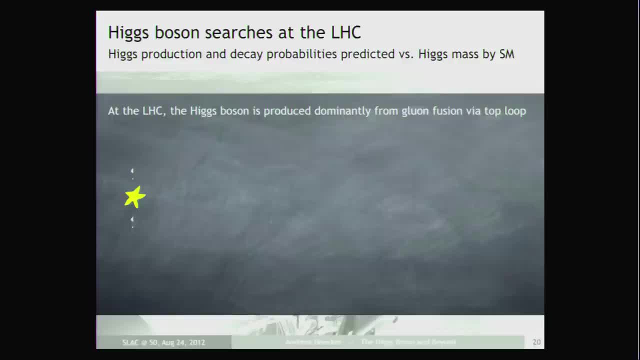 We saw a low X part in distribution function, which are completely dominated by gluons, And so, in fact, what we have is a gluon-gluon collider and not a proton-proton collider, Since the gluons don't interact directly with the Higgs, because the Higgs couples to mass. 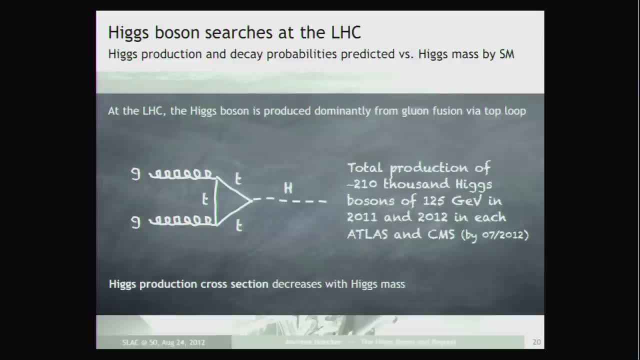 we have a loop here through top loops And in fact we have already 200,000 Higgs on tape each experiment. That's a lot And we think: why did we wait so long until showing that we have the Higgs? 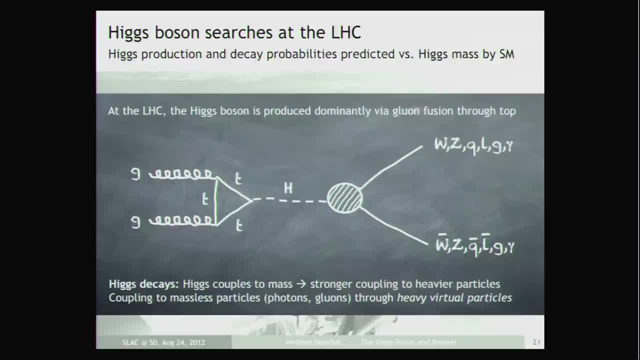 And in reality it is of course very complicated Because the the large majority of these Higgs we can't see because they are completely drowned by backgrounds. So what we really look at for low mass Higgs is the channels, two photons, the Z where 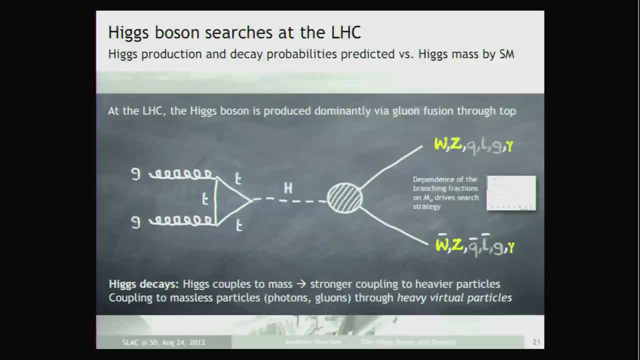 we for Z, we only look into four leptons. So each Z goes to two leptons And the W, where each W goes to a lepton and a neutrino. And this photon in particular is a very, very small channel, very, very low branching fraction. 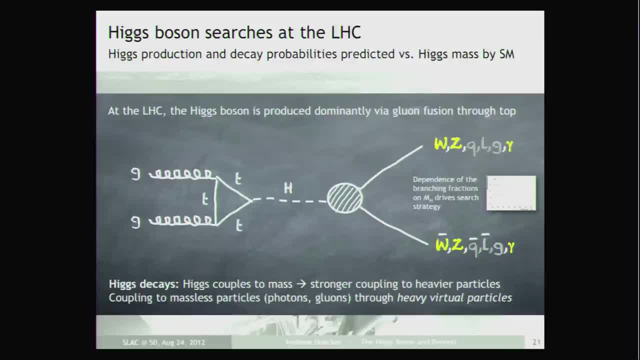 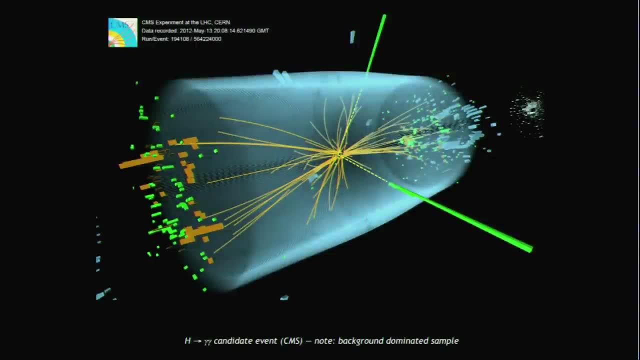 but it's very pure, So we can. we were able to to see this in our detector quite nicely, So I can show you a picture of the CMS detector. here You see the two photons. This is a Higgs candidate. We don't know whether it's a Higgs. 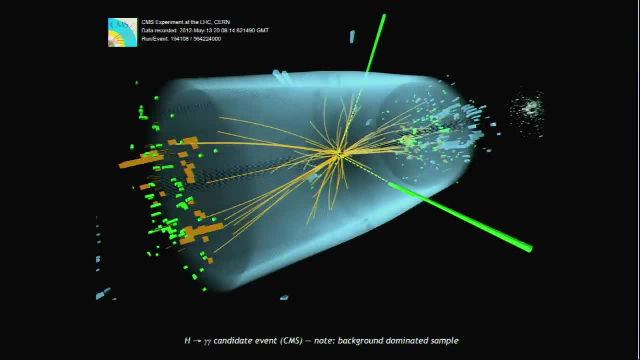 There's a lot of background for a given event. We can never say that's a Higgs in this case, here. So that's a Higgs candidate. What we do is we compute the energies. here. We measure the energies, We measure the angle and compute the invariant mass from this. 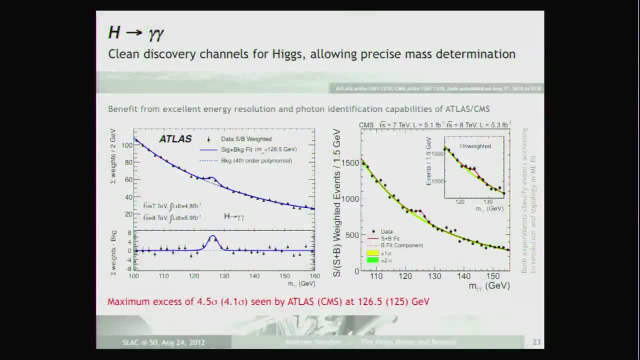 We plot the invariant mass and look for bumps. And you see here, Atlas has seen a bump here at around 126 GV. CMS also has seen a bump here around 125 GV, In very good agreement. both see, in fact, more than a four sigma deviation from the background. 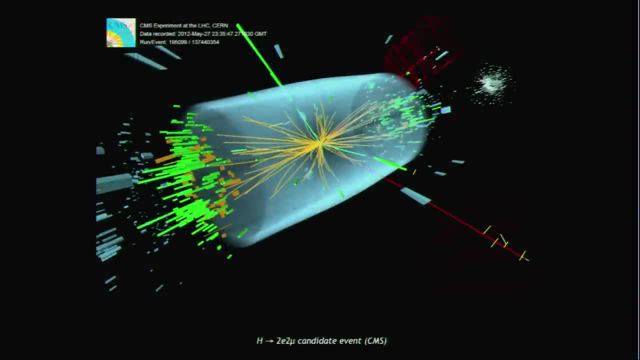 only hypothesis. in this channel We can also look into ZZ production. So in Z this can every Z can go to two leptons with actually a small branching fraction of three percent only. So we can have four muons, four electrons, or two muons and two electrons. 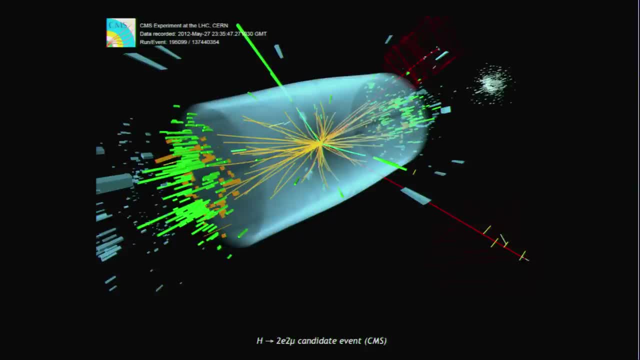 In the event. in this case it's an event in CMS where we have two electrons here and two muons. The muons are minimum ionizing particles. They penetrate the full detector And so we can also- again, we compute. 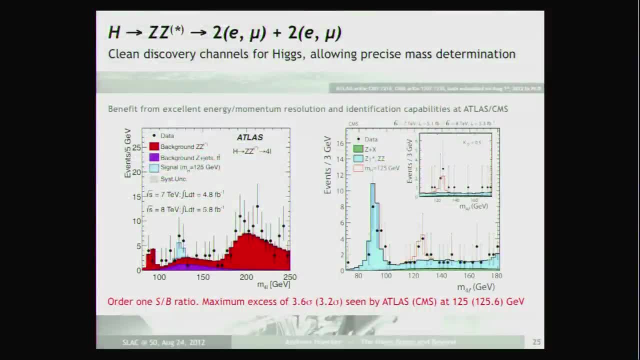 We compute the invariant mass of these particles and plot them and we see we have much less background here. That's nice. It's a very pure channel And we have a peak. That's the Z, It's not the Higgs. 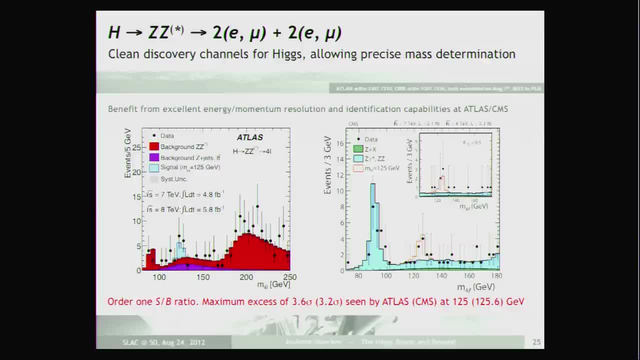 And also the Z can actually go to four leptons. We have a single. we have a small deviation here in both experiments actually, This gives us an excess of 3.6 sigma in Atlas and 3.2 sigma in CMS, again at the same mass. 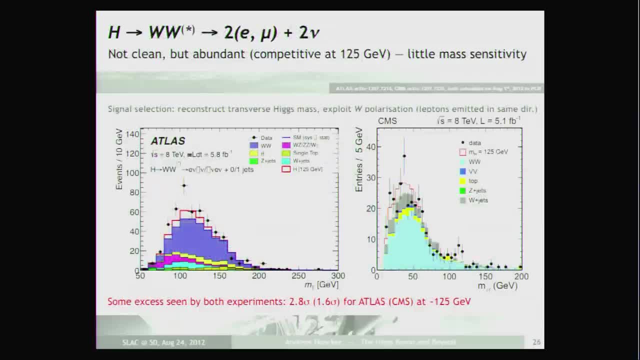 as we had for gamma-gamma. Then, finally, we have the mode in two leptons, in two Ws. So we have neutrinos. We cannot reconstruct the neutrinos, We can only reconstruct the transverse energy balance of these neutrinos. 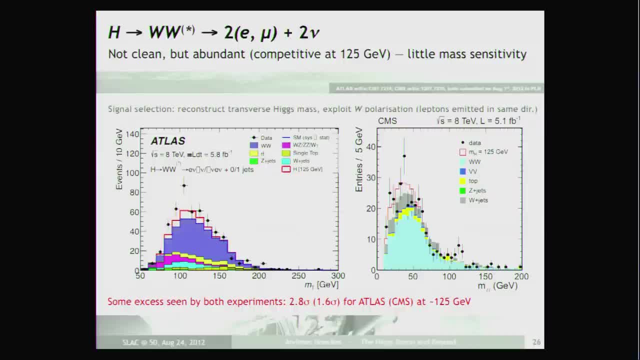 So we can do something like a transverse mass, so something like an invariant mass, which is not as good. It doesn't have very good resolution. You see in red here the resolution of this mass: two Higgs. But we can make a counting experiment. 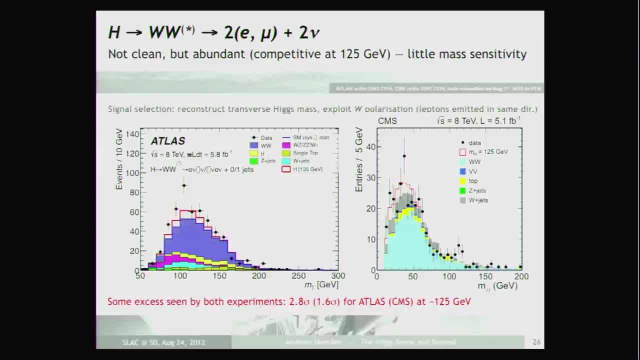 We can see if we have an excess of events, And we do have an excess in Atlas, and we do also have a small excess in CMS: 2.8 sigma in Atlas, 1.6 sigma in CMS. Now we can put all this together. 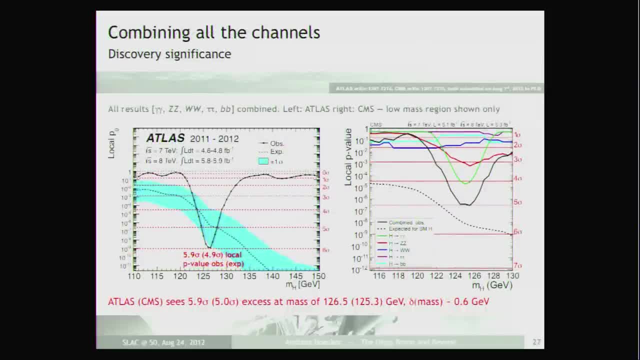 And we can ask ourselves, For each mass we have, what is the probability to observe what we've seen if there's no Higgs? So then we see, the probability is quite high everywhere. but here And so we have here a deviation of 5.9 sigma in Atlas and 5 sigma in CMS at a mass which 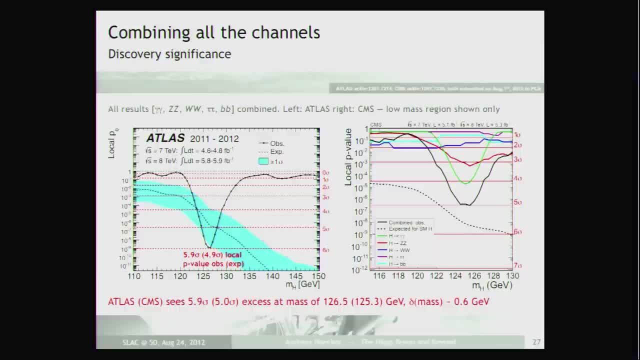 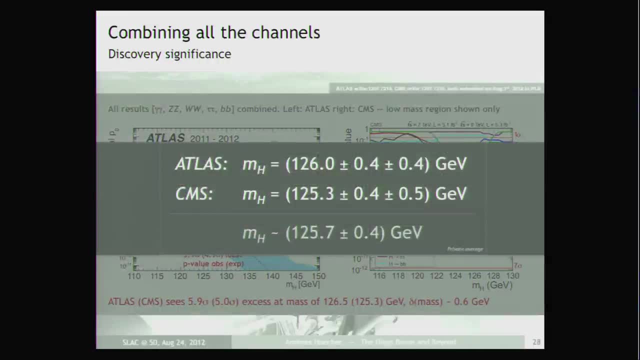 is compatible. So clearly, this is the observation of a new boson, a new particle, And the mass of this is of the order 125.7 plus or minus 0.4.. This is a poor man's average here, but it is probably pretty much that. 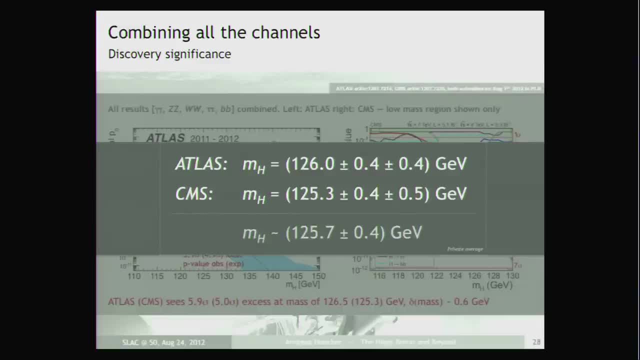 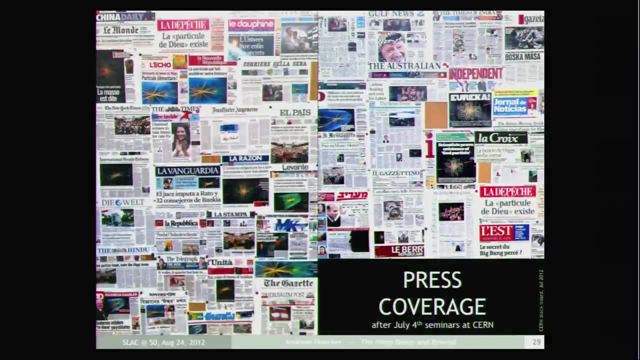 So the mass is actually already very well known. We just discovered it and already know the mass very well. OK, So there was a huge press coverage. I went the next day, of course, I went to the kiosk, into the news shop, to look. 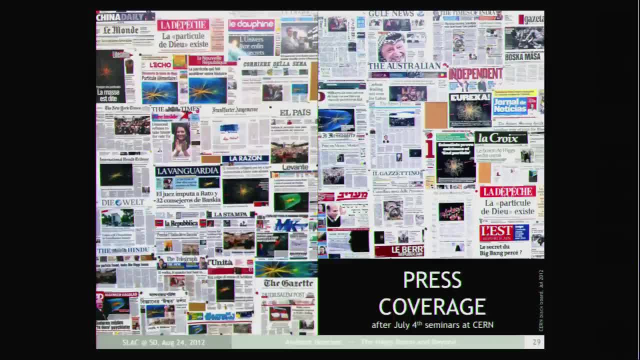 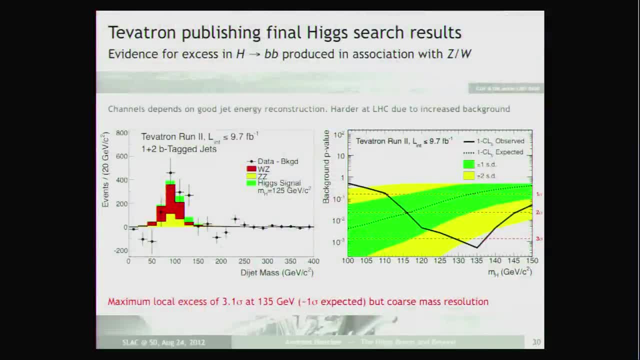 And every, every journal had the Higgs discovery on its first page. This is really a rare moment for particle physics, So we are really happy to have that Now. our, of course, has many, many years of excellent Higgs searches, And we many ideas were brought into the LHC experiment. 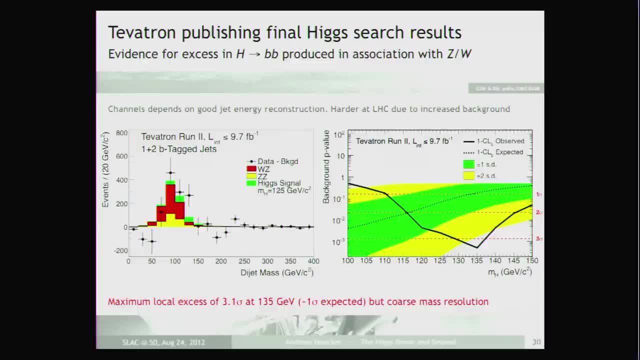 Actually also many ideas from the Bar-Bar experiment here at SLAC were brought into the LHC experiment. We used lots of, we reused lots of the fitting tools of the, the way to do analysis, as it was done in a very dramatically modern way, as it was done in Bar-Bar. 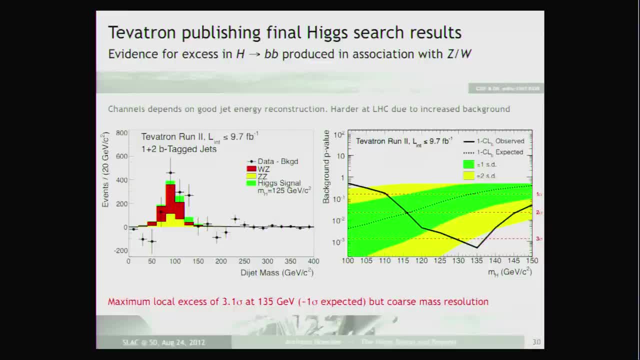 We do it also for Higgs searches, And so Tevatron has also an excess which is in the BB, in the BB channel, Higgs to BB-Bar, which is very, very hard for the LHC. So it's very nice to have this of three point, of approximately three sigma, a little bit. 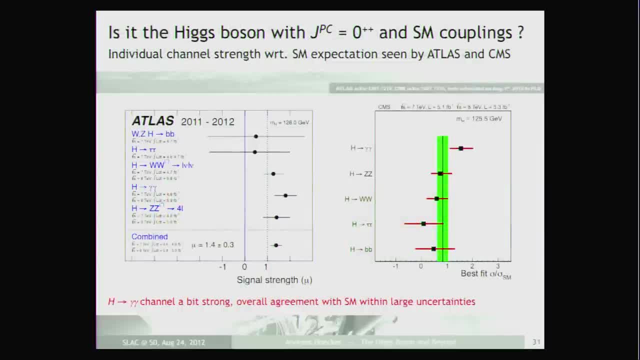 less than that. That's here at the actual Higgs energy. Now the ATLAS and CMS experiment. also, of course, right away start to look into the actual. So you compare each channel with the standard model prediction And so the signal strengths would be one in this case. 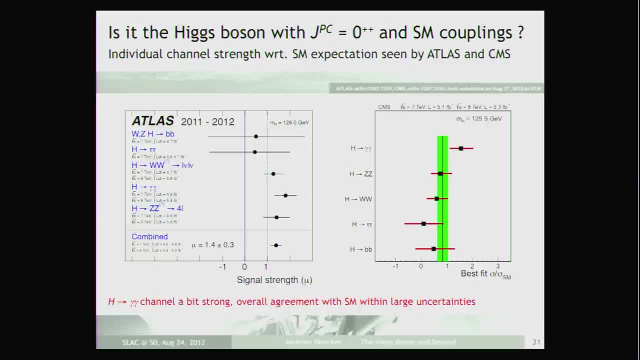 This is the standard model prediction And you see that ATLAS in these three channels- the most important channels- is a little bit above. CMS also is compatible with one here, And both experiments have a little bit of an excess in gamma-gamma which excites a. 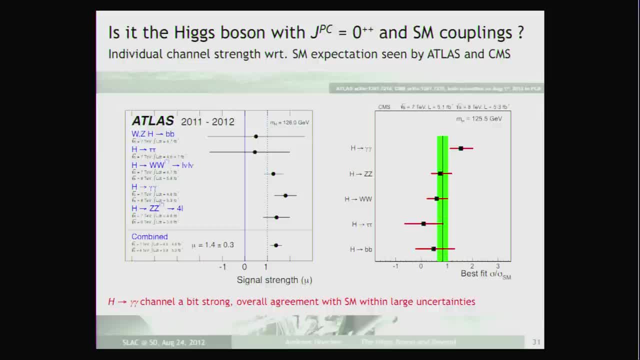 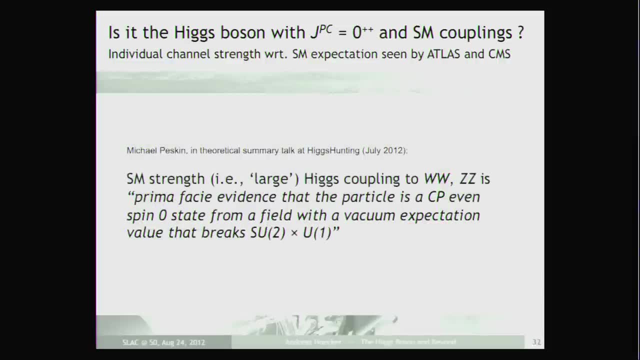 lot of theorists, of course, But we have to wait a long time until a bit more, a bit more- Not a long time, actually, a bit more- to see where this is going to. And I would like to cite here: there was the Higgs hunting workshop just after ICHEP. 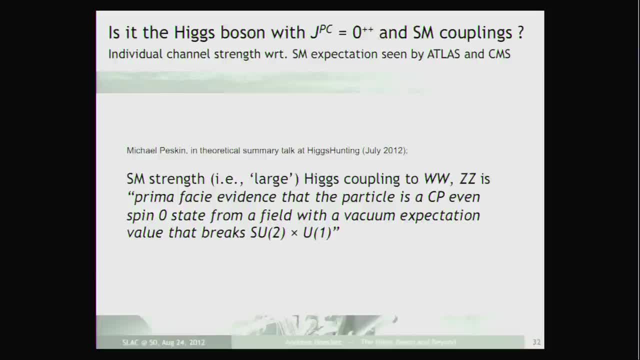 And this is, of course, a great opportunity to discuss all these results, And Michael Peskin was actually giving the theoretical summary talk- a very, very nice talk, And I would like to cite this here what he said: The standard model strength, the Higgs coupling to WWZZ, is prima facie evidence that the 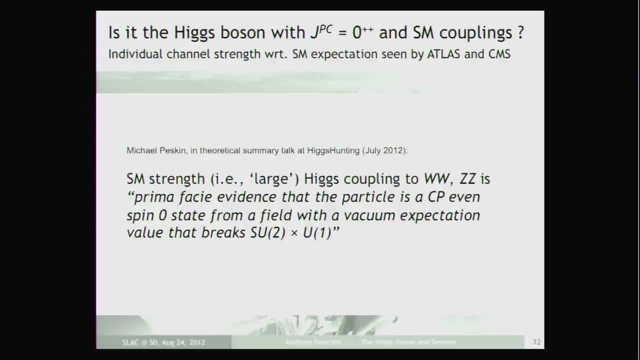 particle is a Cp-even spin zero state from a field with a vacuum expectation value that breaks SU2 and U1. And this is really A subtle comment, because the strength indeed to WWZZ is normally this would be a higher dimension operator and it would not couple if it didn't have a vacuum expectation value. 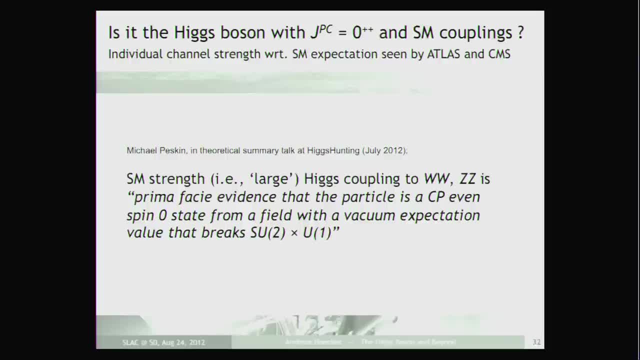 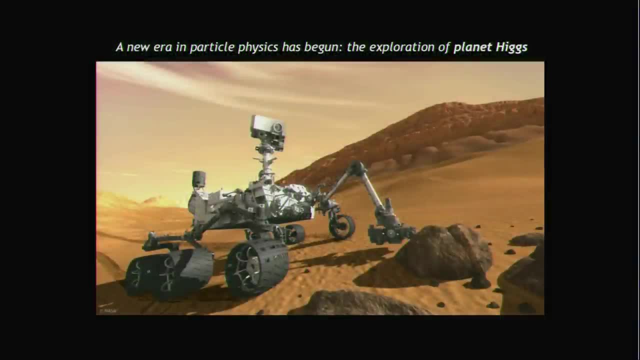 So the fact that we do see this is really indeed not only showing us we have a new particle, but also showing that it breaks electroweak symmetry, which is really interesting. So a new era in particle physics has begun, And the exploration of planet Higgs is starting. 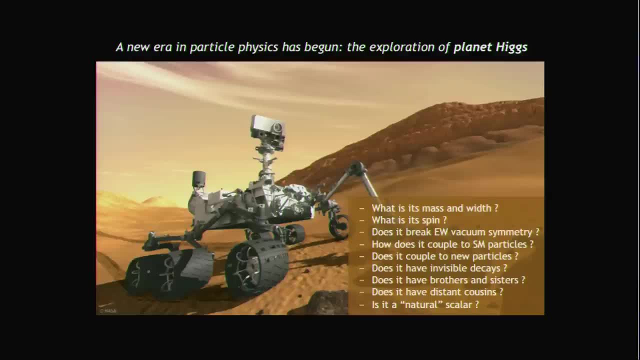 So we have many questions. We want to really precisely measure its mass, The spin, of course. Does it break electroweak symmetry? How does it couple to the standard model particles? Does it couple to new particles? Really interesting, Does it have any invisible decays? 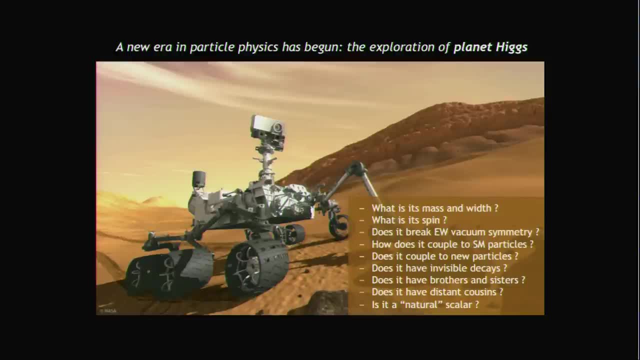 Does it have brothers and sisters? It could not be just a minimal Higgs scenario, but more Higgs's. Does it have distant cousins from higher symmetries, for example? Is it a natural scalar? I will come back to this natural question. 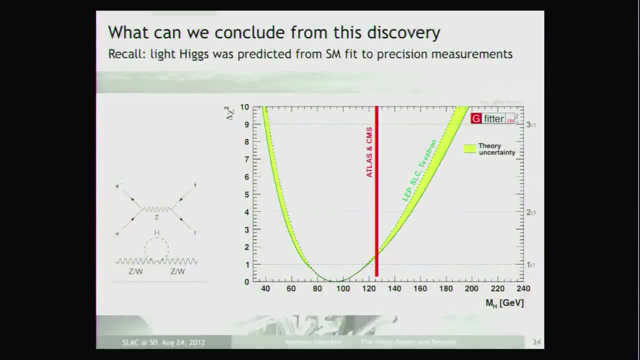 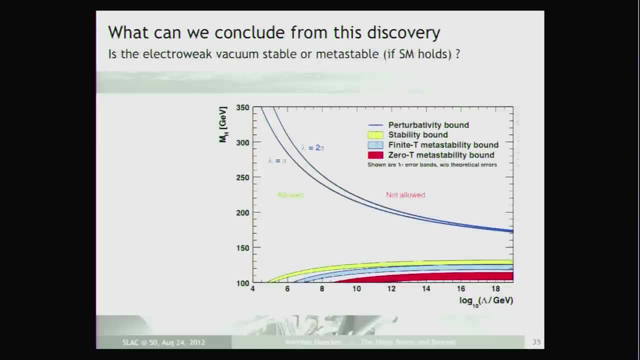 Now we can go back, we can compare to what we knew before and we see we have a fantastic agreement. of course We have a distinction of a like Higgs from the intensity and precision frontier. And we come back also to this plot and we see, actually the Higgs is just sitting at 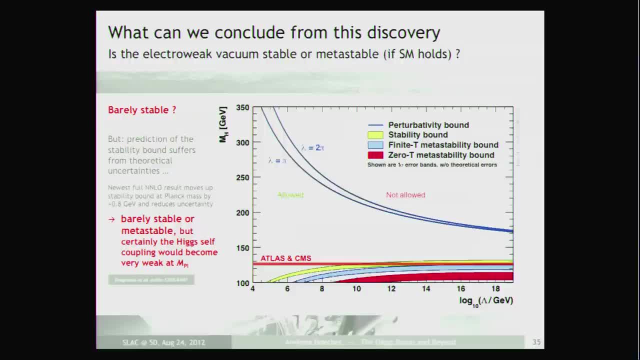 the meta-stability border, And that's quite interesting. I think many theorists are thinking about this. This means the Higgs. self-coupling at the Planck scale if you only have the standard model is very weak, Very, very weak. 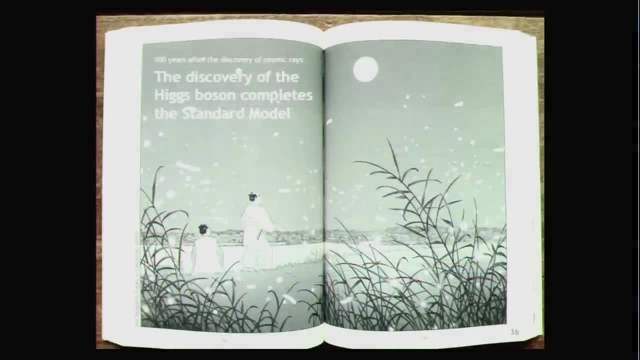 And that's interesting. It probably has consequences, But this is only true if the standard model doesn't have additional extensions in the TV scale. So the discovery of the Higgs boson completes the standard model And it's a triumph for the imagination and rigor of the human mind. 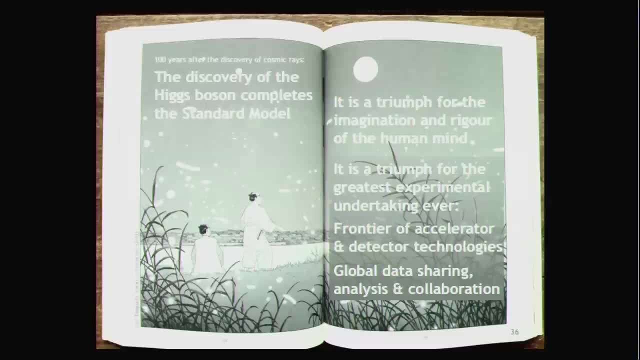 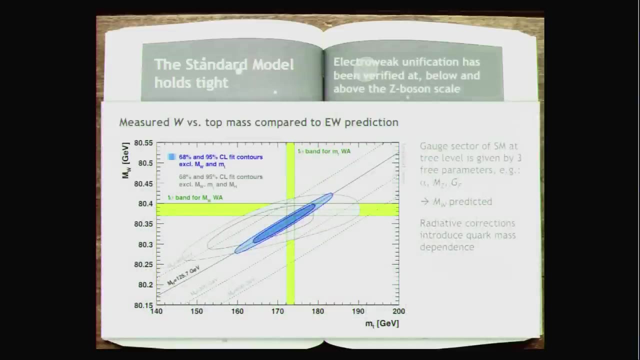 And it's a triumph also for the greatest experimental endeavor ever: the frontier of accelerator and detector technologies, global data sharing and analysis and global collaboration. Now the standard model is tight. I would like to give you a few examples. only, I had lots of them, but then I had to cut down my charts. 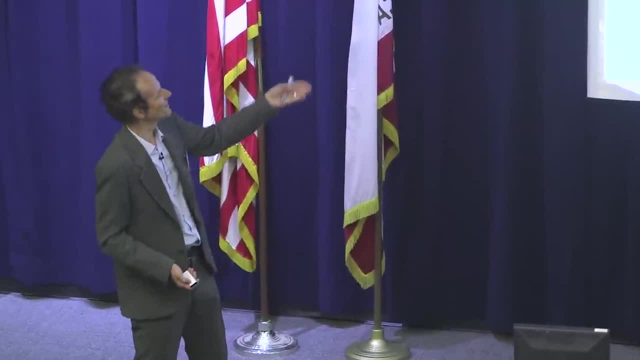 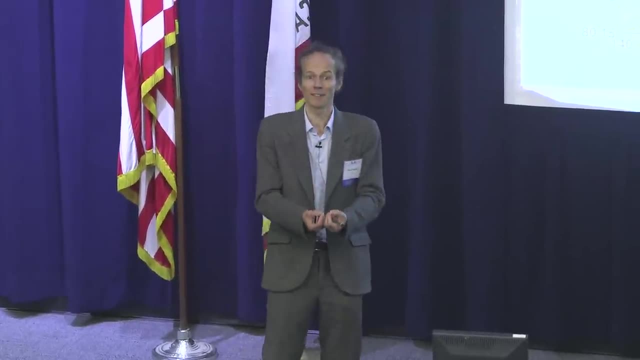 I had to stop, So I'll show you only very, very few. So we have here. this is a picture of electroweak unification Once again, so we can actually predict from electroweak theory, knowing the Higgs mass. 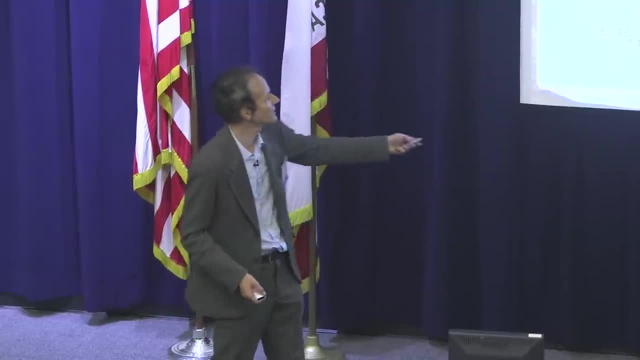 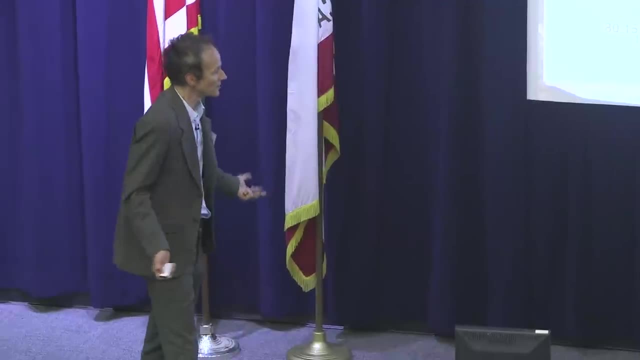 and knowing a few other parameters, the top mass and the W mass, And you see now with the Higgs, we have a very precise prediction here. Compare this to measurement and are in very good agreement. So this really is the proof of electroweak unification. 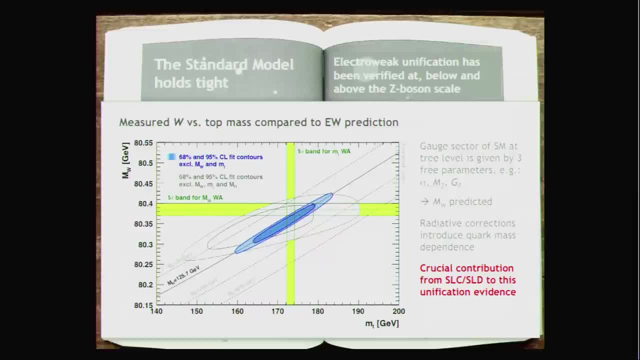 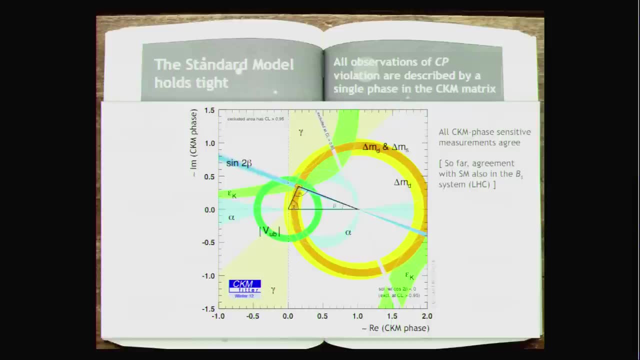 There's a crucial contribution. of course, One of the four most important measurements stem from SLC, from SLAC. Now this picture I have to show. I mean, I can't come here and not show this picture. So we have three generations. 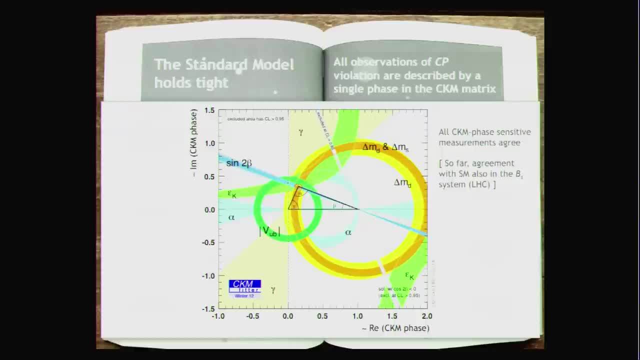 Three generations allow us meta-anti-meta symmetry violation. We must have meta-anti-meta symmetry violation to create the meta-universe we think we live in. So that's absolutely important And the standard model does provide this. It doesn't probably provide enough, but it does provide the feature of meta-anti-meta. 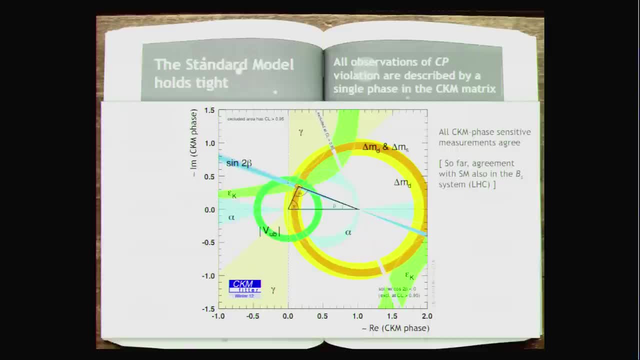 symmetry violation. There's a single parameter for this And it actually gives rise to a huge amount of different phenomena which one can measure. And there judicious people have built an accelerator which can measure this with unprecedented precision: This blue thing here, sine 2 beta, but also all the other measurements. 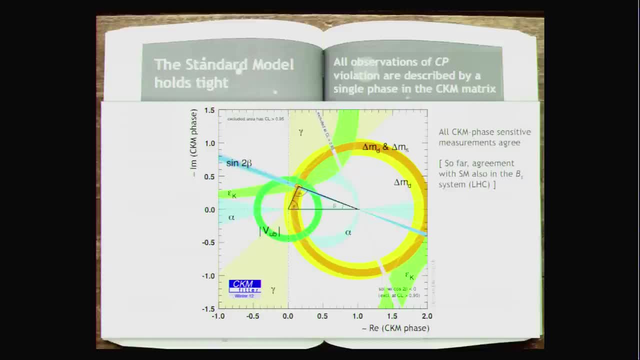 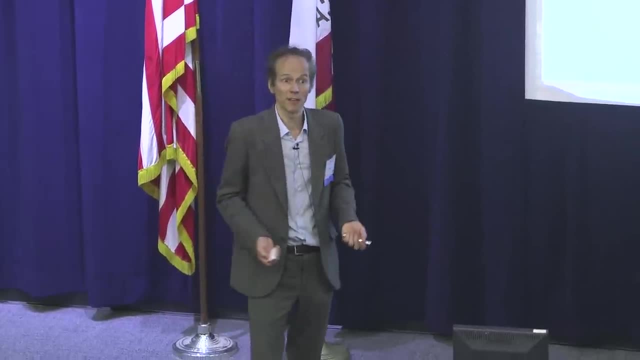 And all the measurements come together to a single point, which was, of course, the confirmation that indeed, the CKM phase, this CP violating phase, is the primary contributor to CP violation in the standard model, And it gave rise to a Nobel Prize for Kobayashi-Maskawa in 2008.. 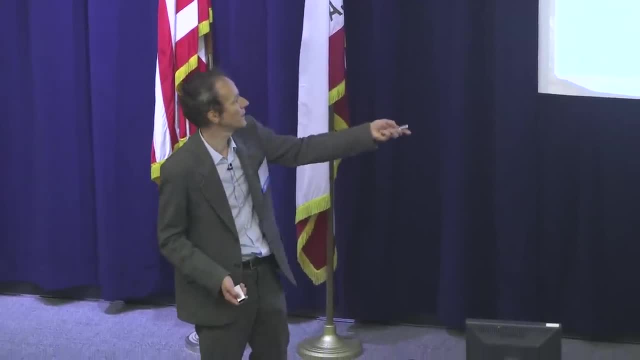 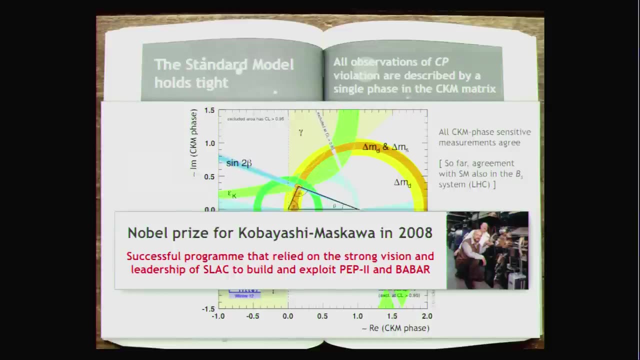 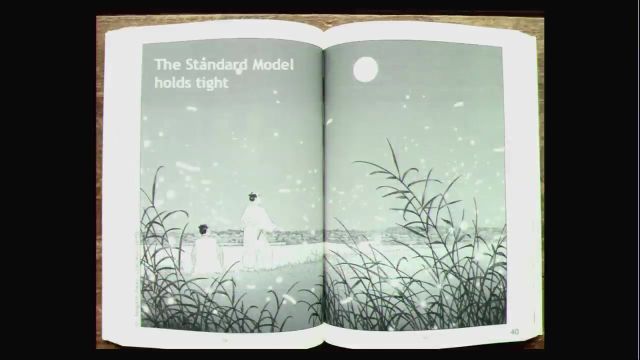 And certainly this successful program has relied completely on the strong vision and leadership of SLAC to build the PEP2 B factory and also the bar, And this went together, of course, with the corresponding experiment, which was running very successfully as well at Japan. 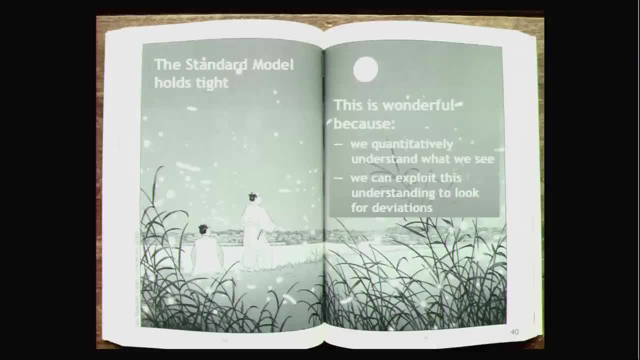 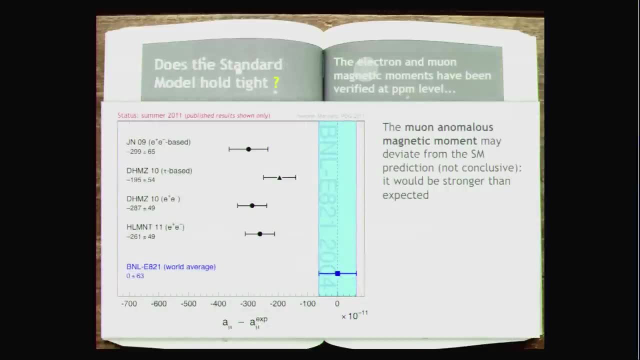 So the standard model holds tight. That's wonderful because we quantitatively understand what we see And we can exploit this understanding to look for deviations. Now I would like to show one example of a deviation, which is a very small deviation. 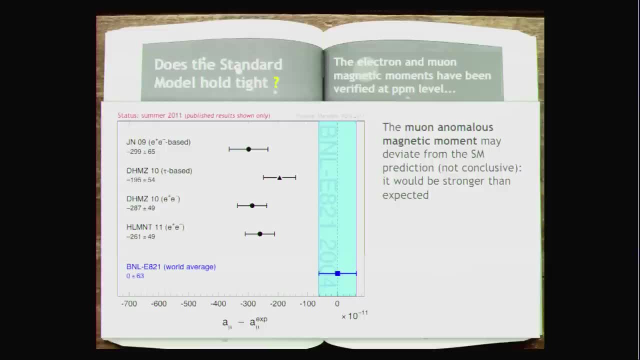 For example, the anomalous magnetic moment can be is: normally the magnetic moment of a muon or an electron is 2. We know this from the direct equation. Then through, virtually through Heisenberg, once again Heisenberg, we get a small offset. 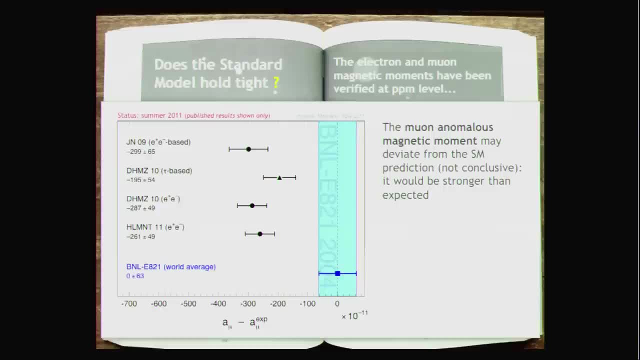 of this, which we can predict to parts per million in the standard model- an incredible precision. And we can measure this also to parts per million. A fantastic experiment at BNL measured this And we see, since about 10 years we have, we live with this deviation between 3 and 4 sigma. 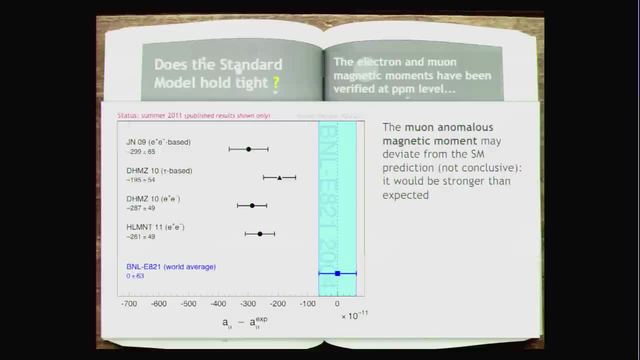 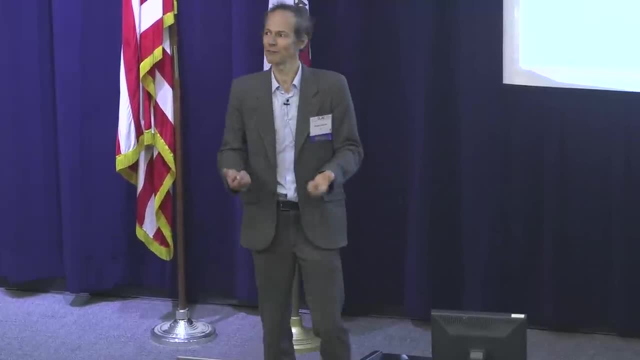 It's calculated by several groups and they all find similar results, And so this is, of course, interesting to follow up. Then there is another feature I wanted to mention in the standard model, which is the Cp. Actually, we should have Cp violation in strong interactions. 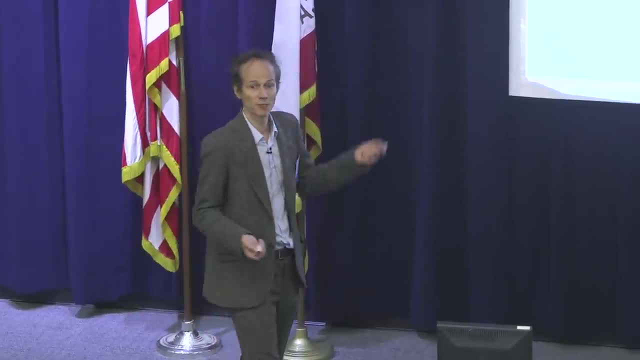 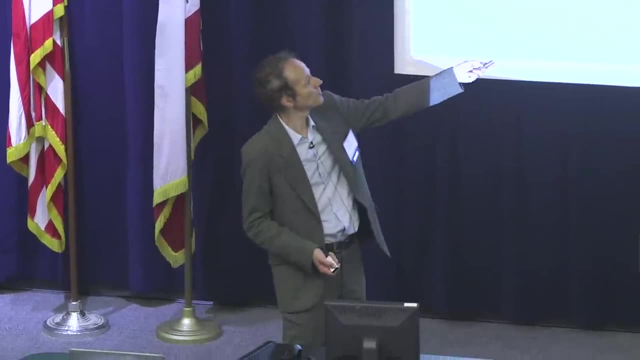 That's something people tend to forget, but we should have. We don't have. It should give rise to an electric dipole moment of neutrons, And we never see this. So we have actually very, very precise measurements here, smaller than 3, 10 to minus 26 e-centimeters. 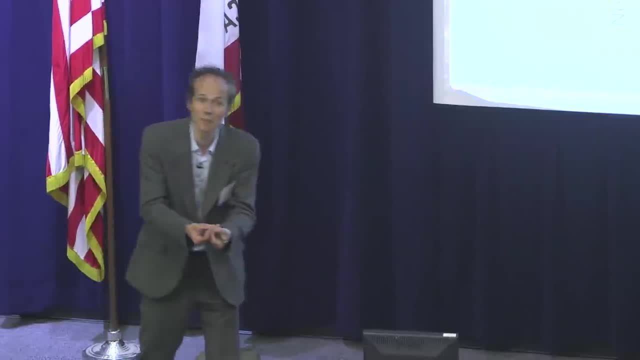 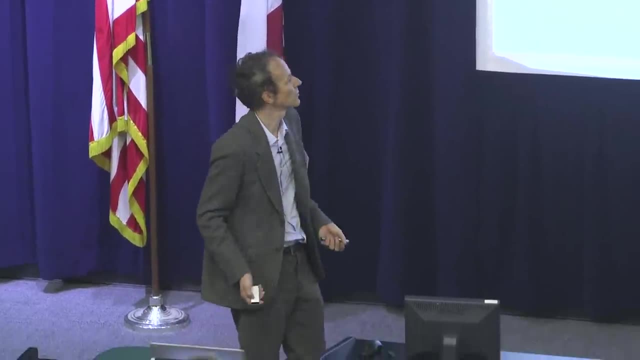 neutron electric dipole moment measurements which give rise to the Cp-variating parameter being smaller than 10 to minus 10.. That's completely ridiculous if there isn't any mechanism which makes it so small, And so this mechanism could be a new symmetry. 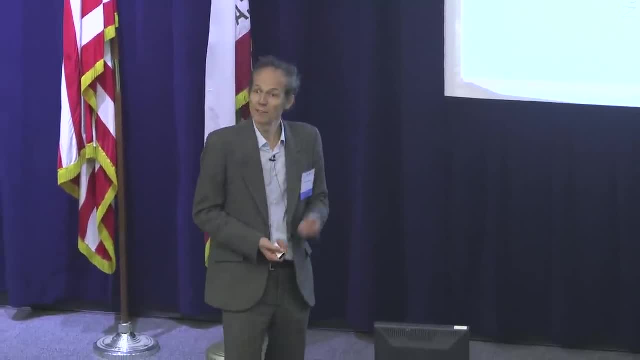 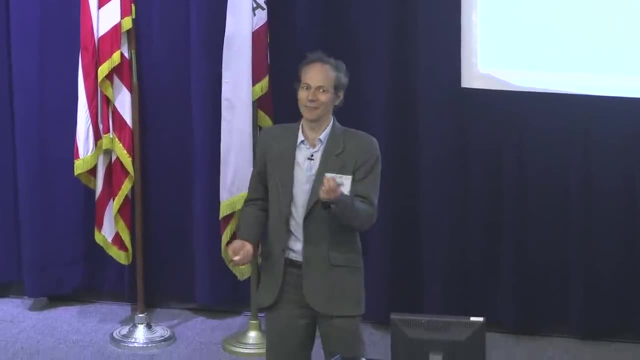 But it's not. It's a new symmetry, which is the so-called Pecet-Quinn U1 symmetry, which gives rise to a new pseudo-Nambu-Golston boson, a new particle which actually has the nice feature. 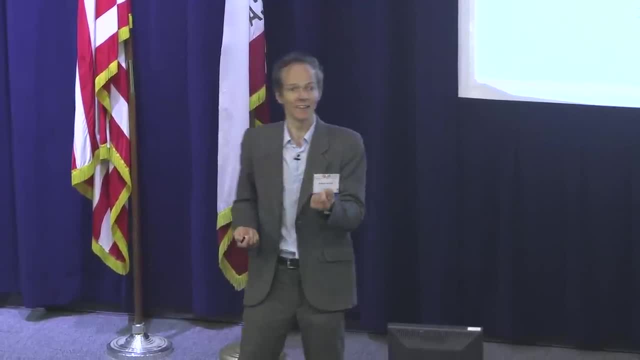 that it condenses in the universe and could be. although it's very, very light, it could give rise to the cold, dark matter we have. So we have two reasons to search for accents. It's something, I think, which is very, very important. 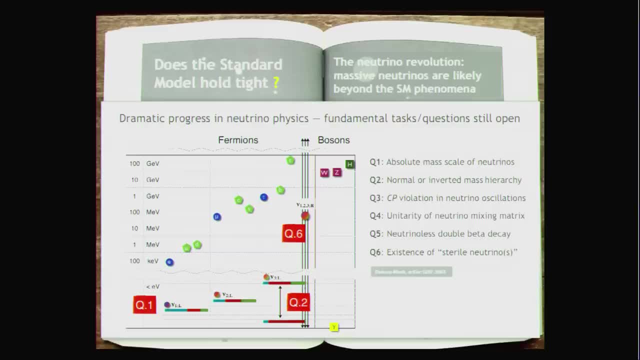 And finally, I must mention, of course, the Neutrino revolution. Since 15 years we are used to. at every conference we get new, very interesting results from the Neutrino sector, And now we know lots of things. 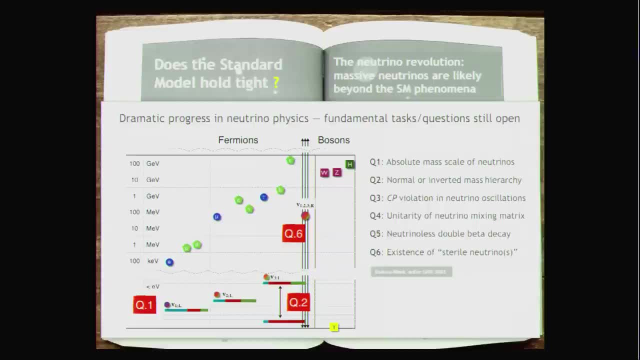 We know they are very, very, very light, much lighter than the rest of the fermions and bosons in the standard model. We don't quite know what the mass hierarchy is. We know they are lighter than of the order of an electron volt. 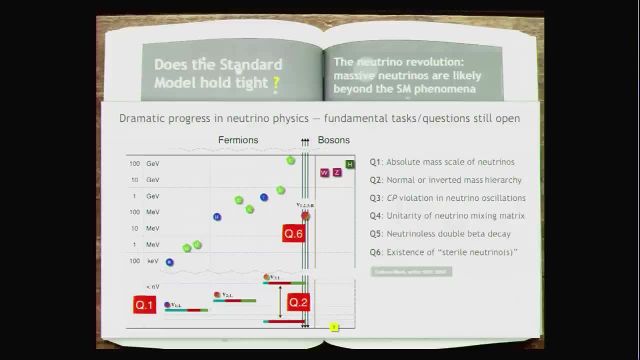 And now we also know their angles. So there are three angles, It's just like in the CKM matrix, And all three have been measured. now, In fact, the hardest one, theta 1,3, is now better known than the supposed to be less. 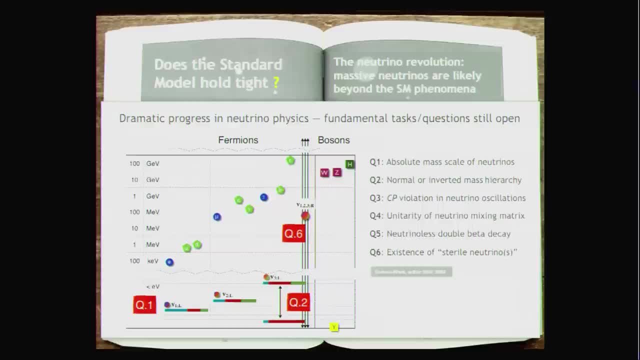 harder one, But this is, for the moment, what we know, Not more, And so there are many, many questions. We want to understand the absolute mass scale of neutrinos. We want to see whether we have a normal or an inverted mass hierarchy. 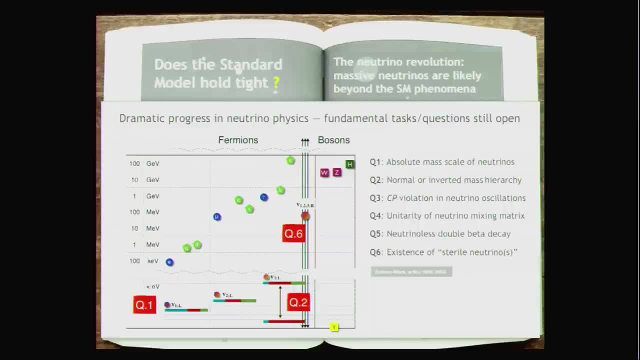 We want to measure, of course, CP violation in neutrino oscillations. We want to measure the unitarity of the neutrino mixing. So the same program as we did for the slack B factory: Neutrino less, double beta decay, to understand whether neutrinos are their own particles. 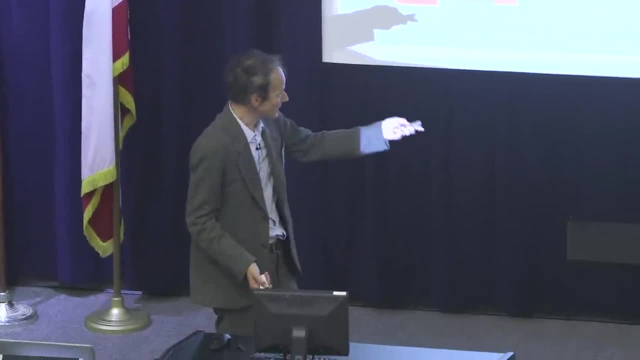 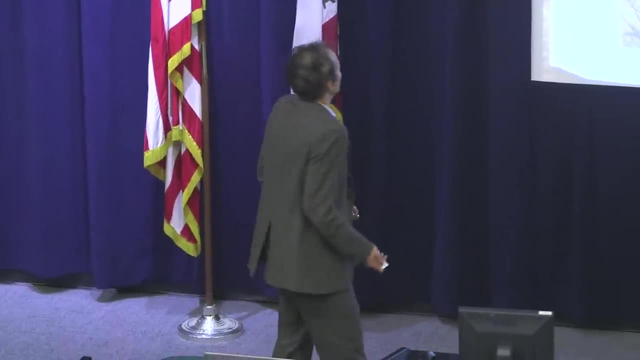 anti-particles or whether they are direct particles, And whether there is any existence of sterile neutrinos, neutrinos which do not obey weak interaction, But only gravitation. So can we conclude from the standard that the standard model is the theory of matter? 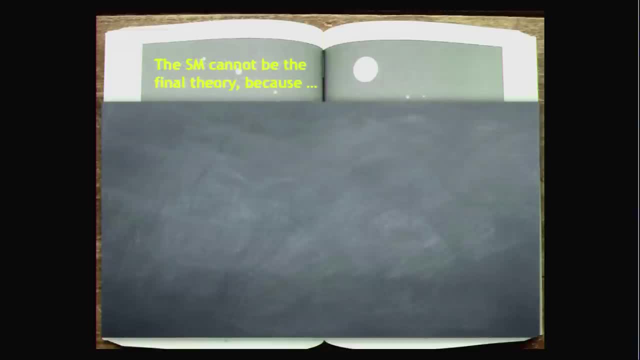 from what we know so far- And certainly we cannot- There's no way it could be. The Higgs is the only fundamental scalar. All other scalars we have are composite particles, So it's very strange to have a single fundamental scalar. 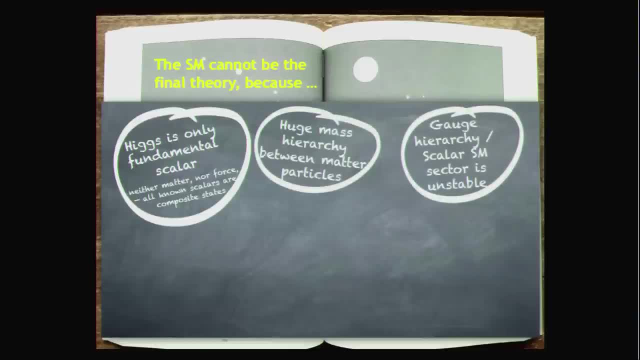 There's a huge mass hierarchy between the matter particles, a gauge hierarchy problem. I will come back to this problem in particular. There's dark matter and dark energy, of course, not contained in the standard model. There's inflation: It's also not contained. 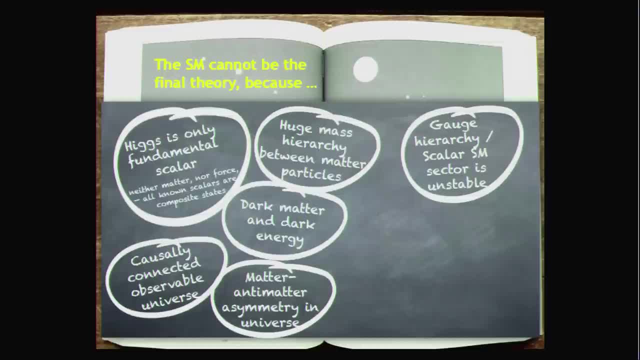 The material antimatter symmetry. the CKM mechanism is nine orders of magnitude too small to create the material antimatter symmetry we observe in the universe. Grand unification of the forces is not generated by the standard model. The strong CP problem, I've said massive neutrinos and finally gravitation. 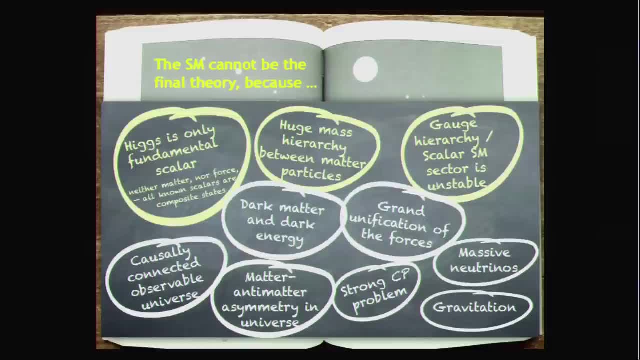 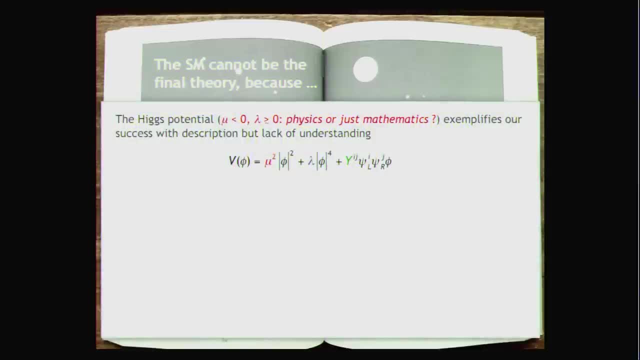 Gravitation is not at all included in the standard model. We cannot be happy with such a model at the moment, So I will come back to these ones, because these problems here are directly related to the potential I've shown you already from the Higgs. 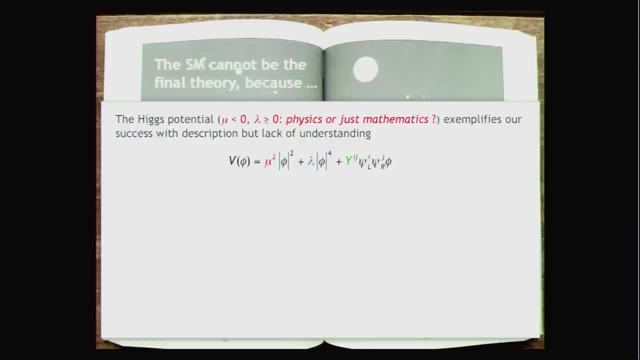 So this is the Higgs potential And actually I like also Michael's reaction at the Higgs hunting workshop. In some way this exemplifies our successful description, but lack of understanding. Is this what we just postulate, the potential we want? 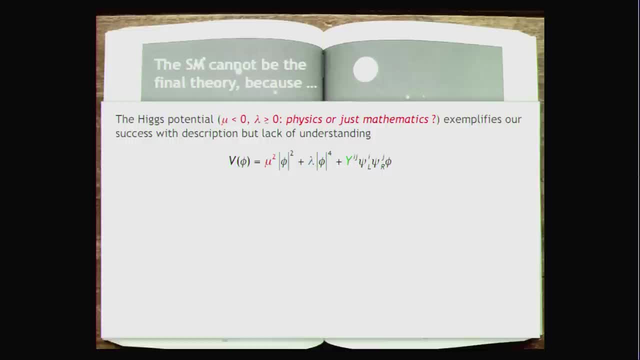 Or shouldn't we actually have a better theory which predicts this potential? It comes out of dynamic properties of this model that the potential has this form or another form. So first, the mass term has a huge problem. In fact, it receives. It receives radiative corrections of this type with top exchange, for example. 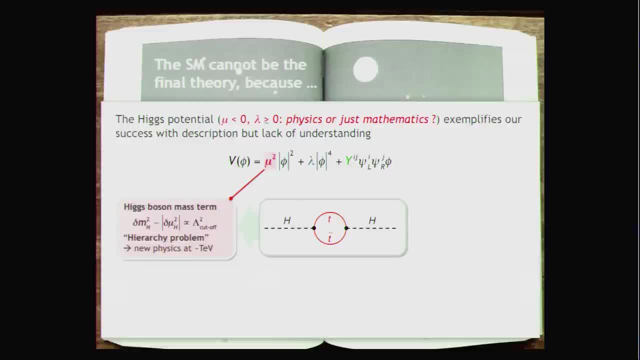 And if you go up in energy and you stop, you cut off the standard model, for example at grand unification or the Planck scale. at the Planck scale the mass of the Higgs would actually have these corrections become huge. 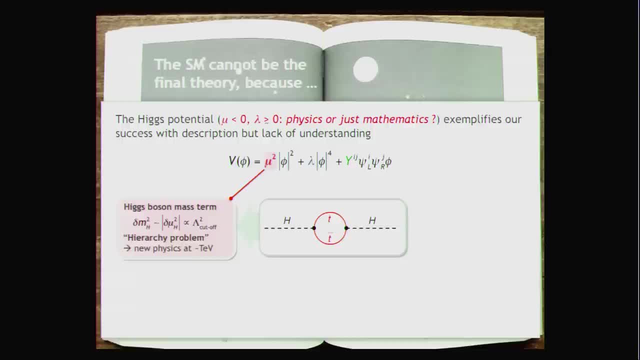 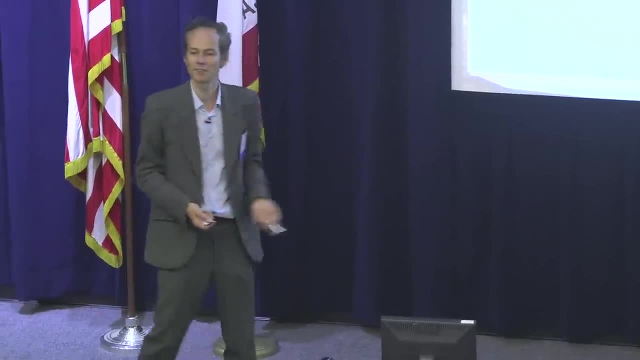 And the mass of the Higgs would have the mass of the Planck scale And so to have the Higgs mass so low means we need to have a cancellation- ridiculous cancellation- of two numbers of 10 to 19 GV to come up with 100 GV. 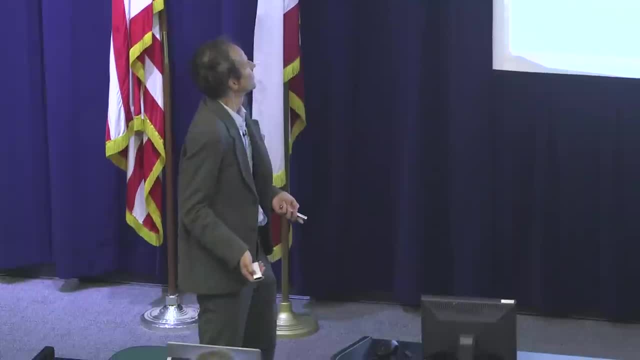 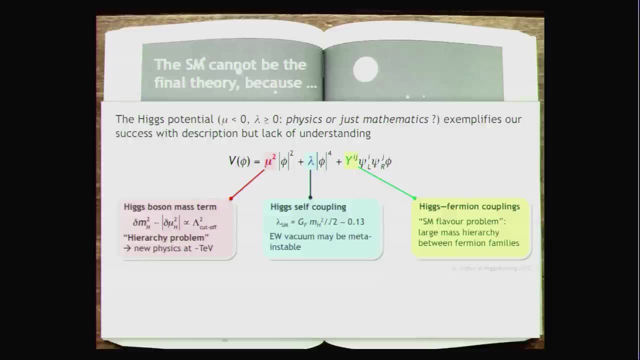 It is completely impossible. That cannot be the truth. So then, of course, We have to understand the lambda. whether we are in a stable or an emitter-stable universe, We have the same flavor problem. These couplings here give the fermion masses, but they are very, very different. 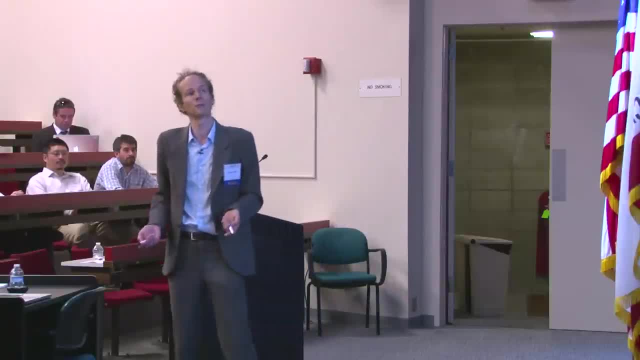 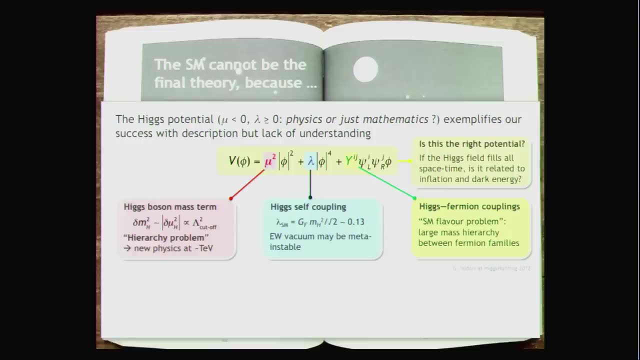 And we have no way, in the standard model, to understand where the hierarchy stems from. And then also, is this actually the right potential? And if the Higgs field indeed fills all space-time, is it related to inflation and dark energy? 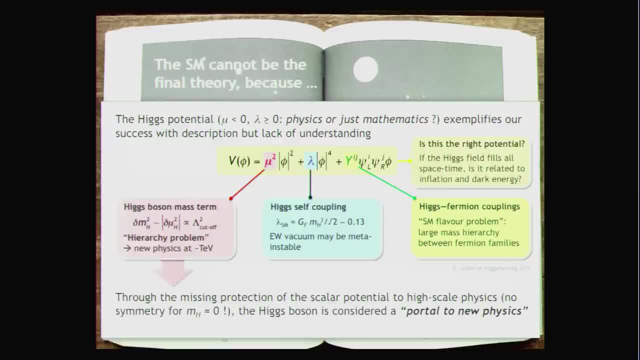 That's an interesting question. So getting back to this here, the missing protection of the scalar potential to high-scale physics. There is no symmetry. The Higgs mass is to zero. If you put the scalar, the quark mass is to zero. 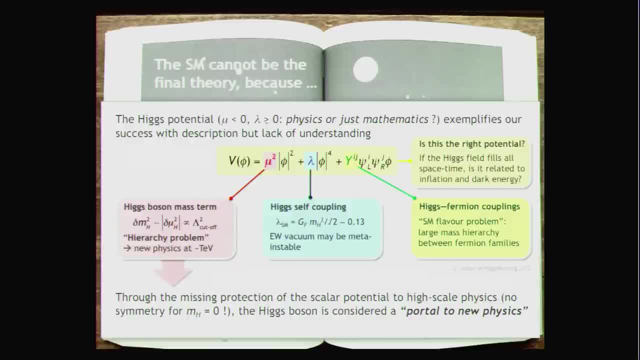 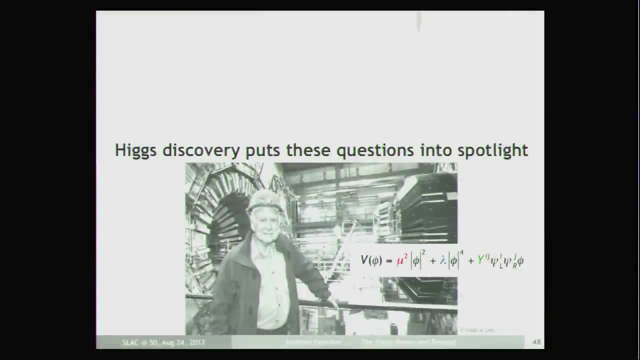 For example, we recover chiral symmetry, which is very interesting, which is naturally makes the quark mass light. It's not the case for the Higgs, And so the Higgs is considered the partner to new physics. So the Higgs discovery now, of course, puts these questions into the spotlight. 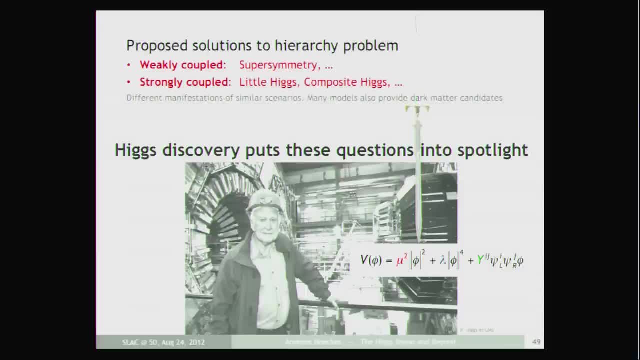 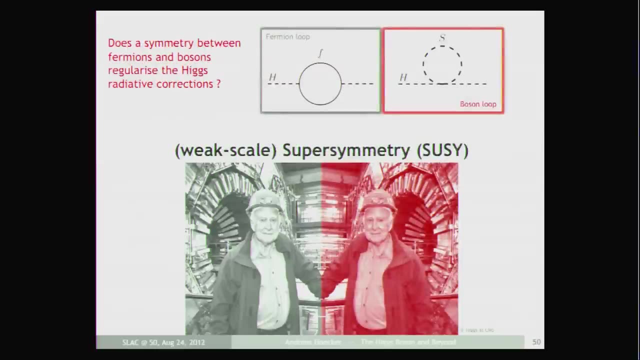 And theorists are incredibly creative in producing models which could evade these problems In particular, for example, weakly coupled solutions like supersymmetry, composite, Higgs, which are more complex, Or more strongly coupled solutions, And all these, of course, introduce new physics at the T scale, extra dimensions, for example. 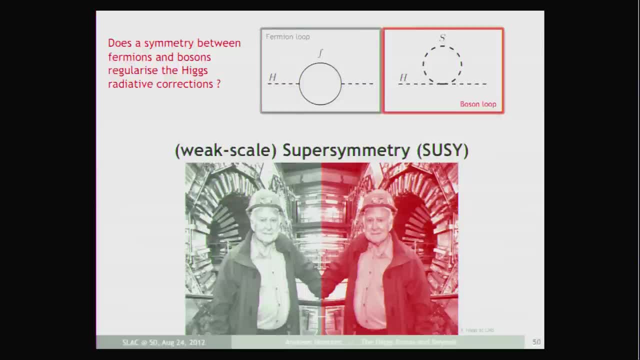 So, for example, does the symmetry between ferments and bosons regularize the Higgs radiative correction. So we have seen this correction here: If you have a top loop produces a huge amount, huge contribution to the Higgs mass. And then if you had the corresponding scalar loop here, it gives a negative sign and cancels. 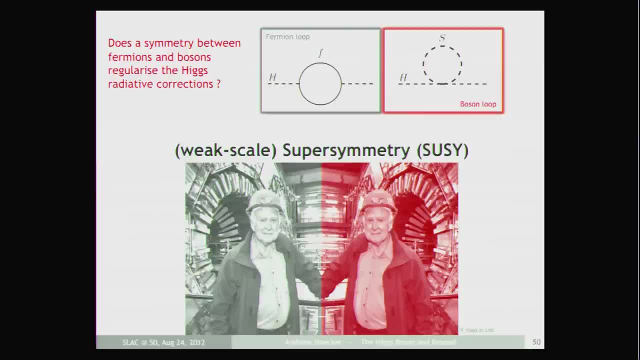 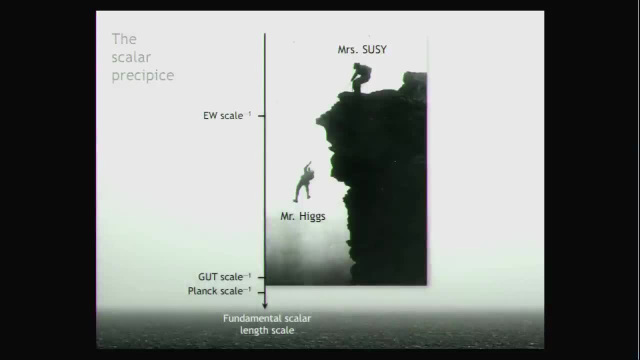 to all orders of perturbation theory. this contribution, That's very, very elegant. It's so elegant it must be true. We have to see So. that's weak-scale supersymmetry, and we can imagine this in our case. 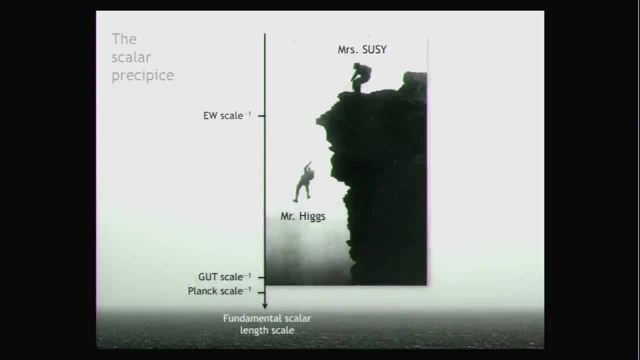 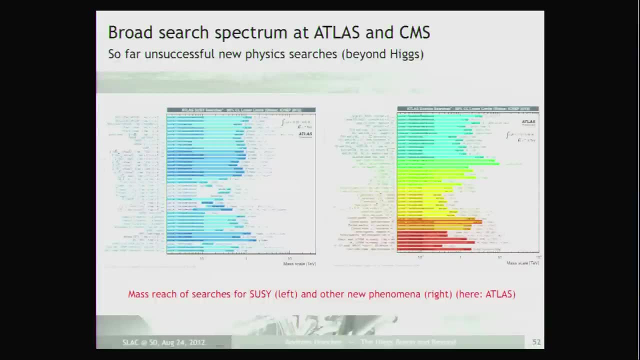 So Mr Higgs wants to fall into the scalar precipice, which is incredibly deep, And Mrs Susie is sitting here and holding it back at the electroweak scale. Now the Atlas and experiment have a huge amount of production, very, very productive. 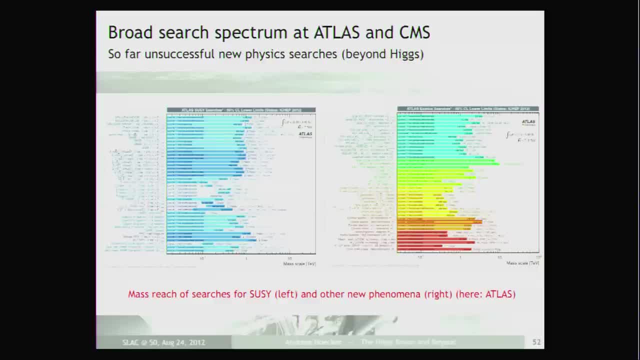 in searching for all these new physics models. All these physics models don't only produce Higgs partners, they also produce lots of new particles which can be strongly interacting, for example. These are all the limits in supersymmetry. These are all the limits in Atlas IV models beyond supersymmetry. 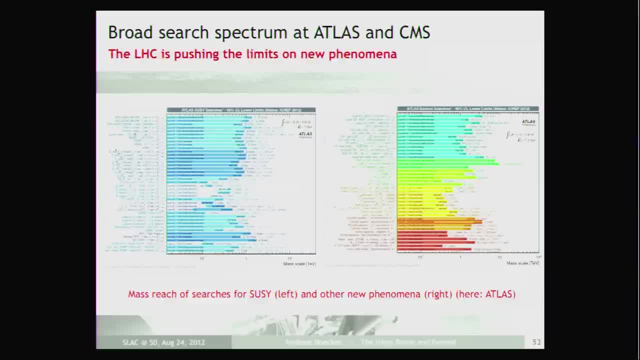 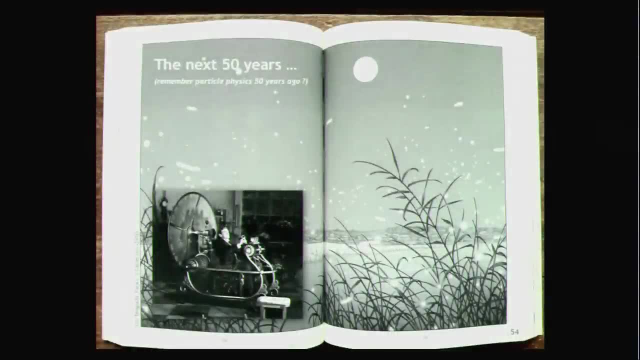 And you see we are reaching the TEV scale in these models. So clearly the LHC is pushing the limits on new phenomena here And I have to go to the next 50 years. So remember particle physics. 50 years ago There was no quarks, no CP violation, no standard model. 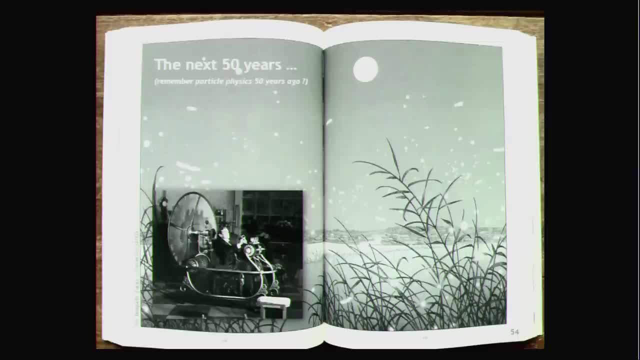 There was, I mean all these things. it's basically impossible. no Higgs mechanism, It's impossible. You can't predict what is going to happen 50 years from now. So I just wanted to go along a little bit. the options we have. 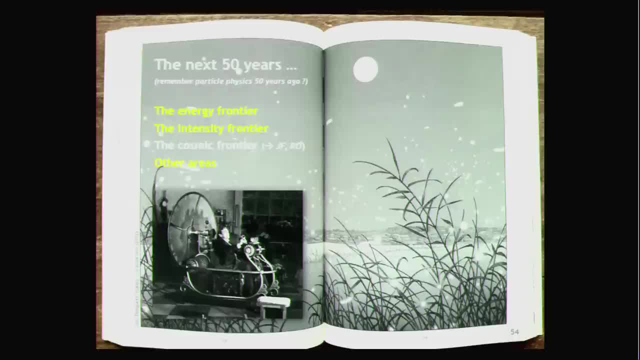 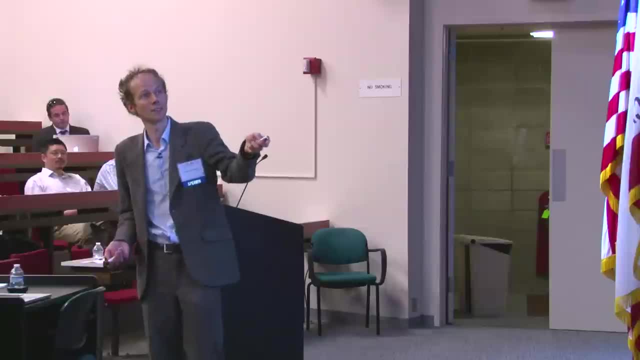 So we have the famous option of the energy frontier, the intensity frontier, a few other areas I would like to mention, Then also the cosmic frontier, which will be covered greatly by Jonathan Feng and Reni Ong later, And the introduction to future accelerators. I will assume you know what these accelerators? 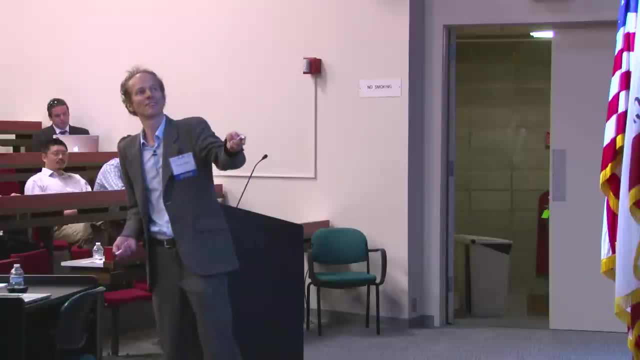 are, And so then, Frank will really put the details on these machines later today. So the high energy frontier: all we're doing will depend on what the LHC is. So we have the high energy frontier. All we're doing will depend on what the LHC is. 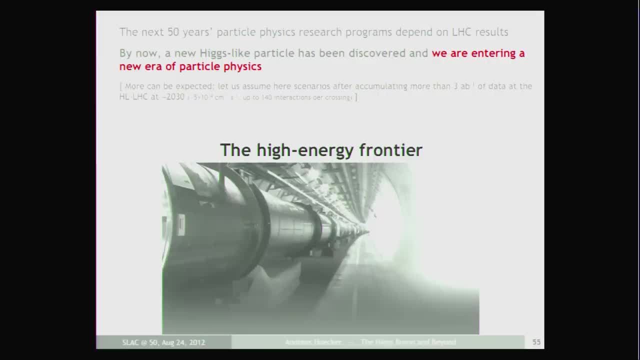 So we have the high energy frontier. All we're doing will depend on what the LHC is. All we're doing will depend on what the LHC is. All we're doing will depend on what the LHC brings us So far. we have a new particle which we have to study for sure. 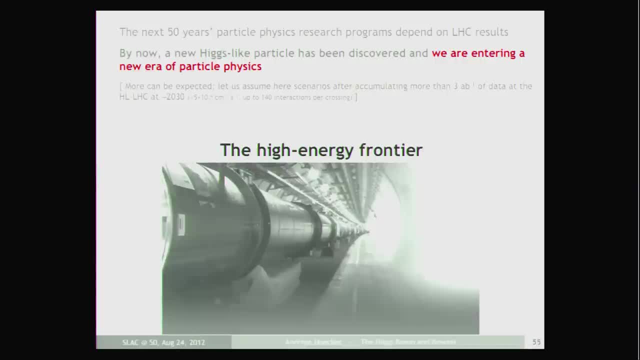 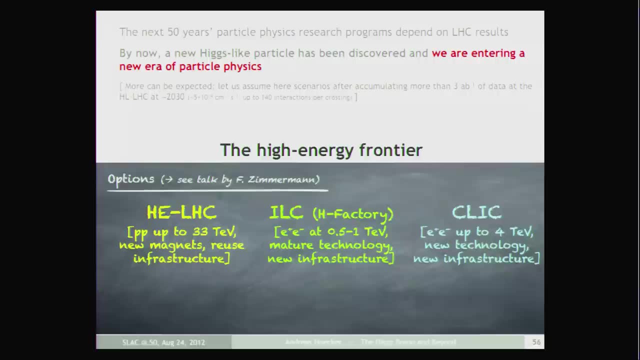 That's clear. But then the next, of course, depends on whether we find additional particles. So the options we have for this is we can double, or even more than double, the energy of the LHC by putting a larger, stronger magnet into the ring. 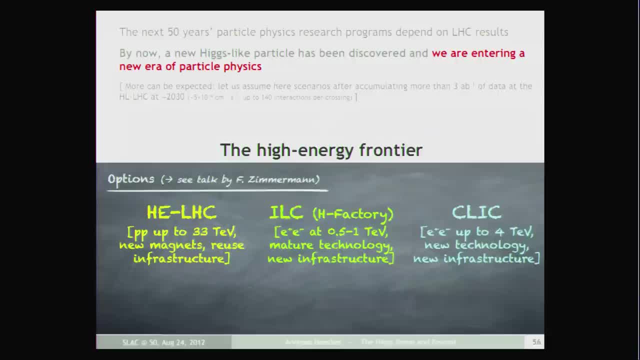 We can build a Higgs factory, which would be a linear collider, E plus, E minus, colliding to 500 GV or even having the possibility to go to 1 TeV. This is a mature technology We could basically start. 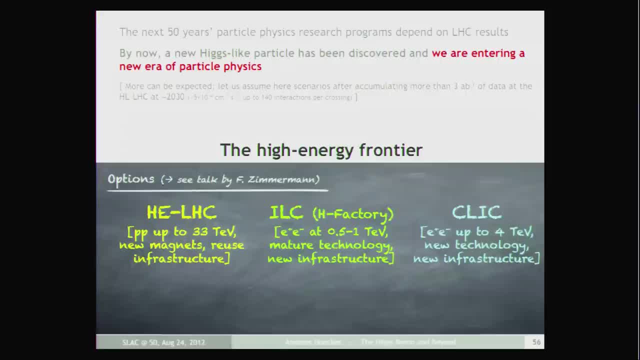 start the construction right away. And then there is Qlik, which allows to go to much higher energy, but it's new technologies which needs a little bit more R&D to be able to run it. And then there are very interesting additional projects, like a very large LHC, which needs, of course, a 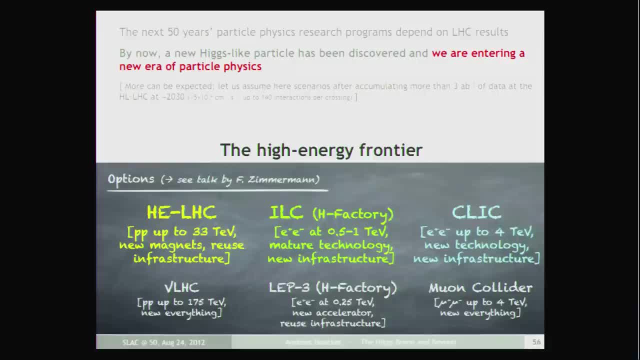 new tunnel. That's a big investment. Then LEP3, which has the idea, that's a relatively new project, which reuses the LHC tunnel to build there a stronger E plus E minus collider than LEP to be able to produce actually Higgs, so Higgs plus Z. 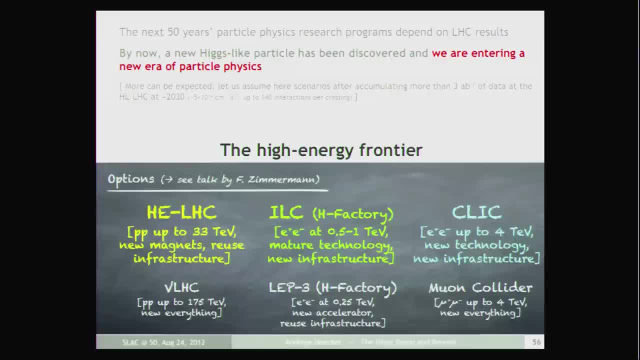 And then there is the very fascinating idea of a muon collider, which is new, everything. It is very, very challenging technology, But of course it has extremely interesting advantages because it's very, very compact and was supposed to be much cheaper than these huge solutions here. 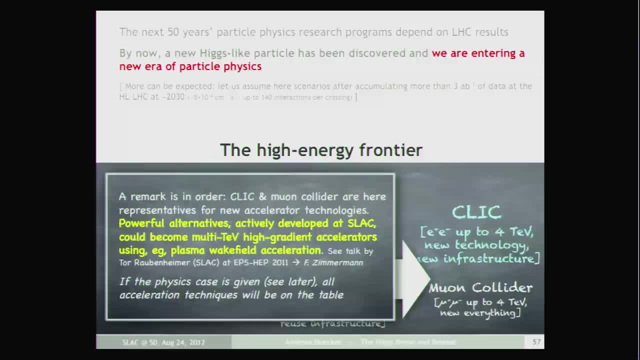 So I would like to make one point here. Qlik and muon colliders are basically here representatives of new accelerator technologies, And they are very powerful alternatives which are actively developed at SLAC, And I would really like to mention these very, very. 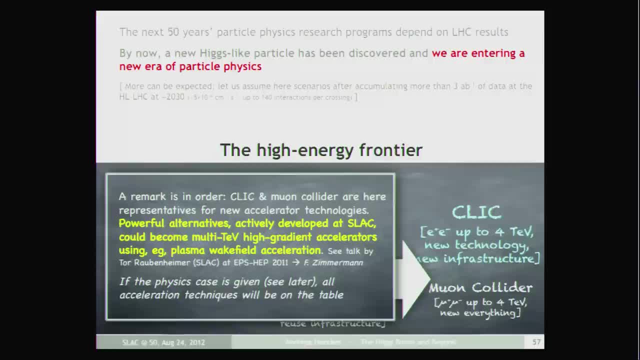 interesting high-gradient accelerators, for example, any kind of wakefield acceleration like plasma wakefield acceleration, And so there was a very interesting talk last year from Thor Robbenheimer at EPS, HEP, on this, And Frank will of course also go into the details of. 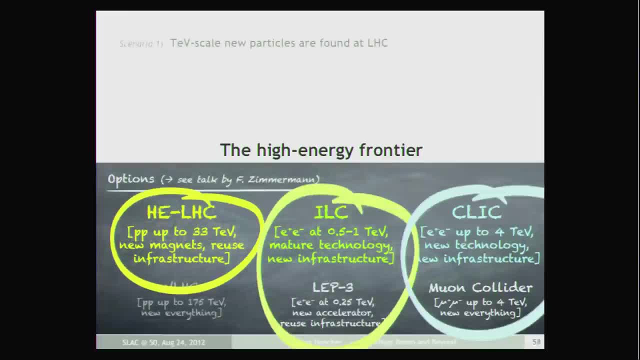 these possibilities, which are very, very fascinating. So let's assume we have observed lots of new physics at the LHC. We have the option to build everything. We want to build an ILC to measure the Higgs Qlik to measure with precision the heavy particles. 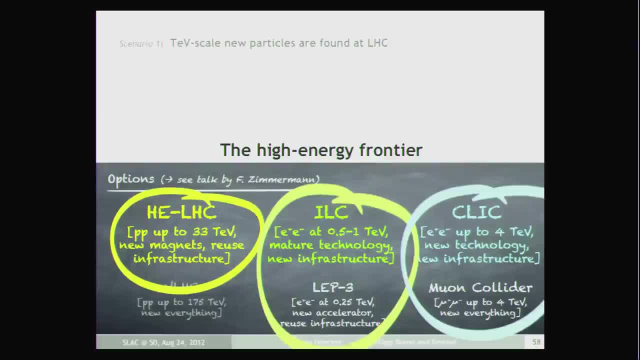 And also a high-energy LHC to go beyond what we've seen so far. That's basically an easy scenario. So we stay with the standard model Higgs. so far at the LHC, We don't observe any new phenomena at the LHC. 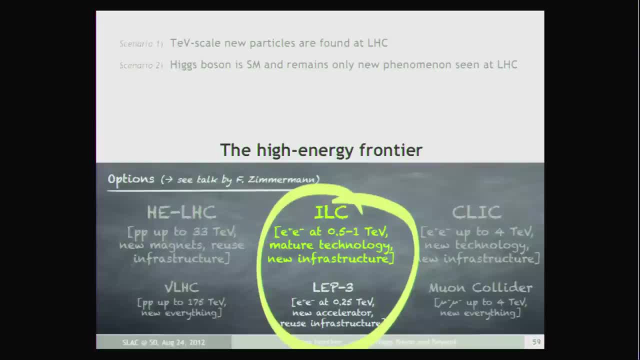 In that case we still need an E plus, E minus collider to measure to great precision the Higgs properties. And then, if we do not observe any new physics beyond the Higgs at the LHC, but we do observe physics at the 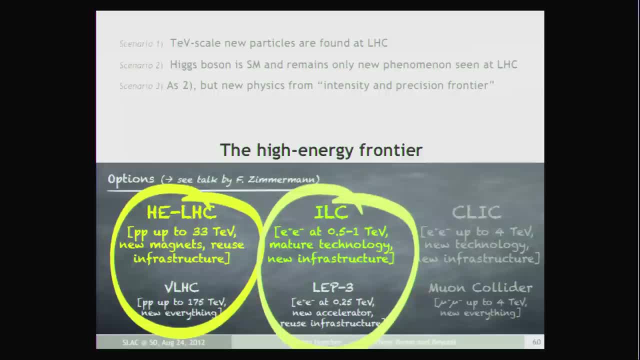 intensity, frontier, new physics, for example, charge lepton flavor variation. in that case we need to estimate what is the scale of this new physics And we would need a new high-energy collider to find this new physics. And we also need an ILC, a Higgs factory, RLF3, to be able. 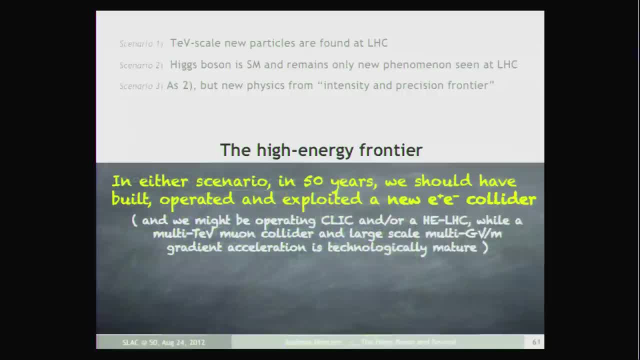 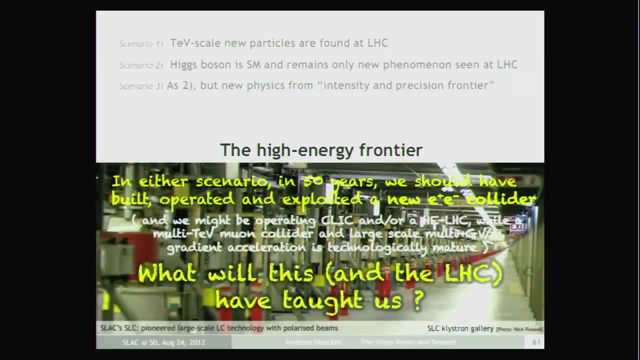 to measure precisely the Higgs properties. So in any case, in either scenario, in 50 years we should have built, operated and exploited a new E plus, E minus collider. So what will this have taught us? and the LHC together? 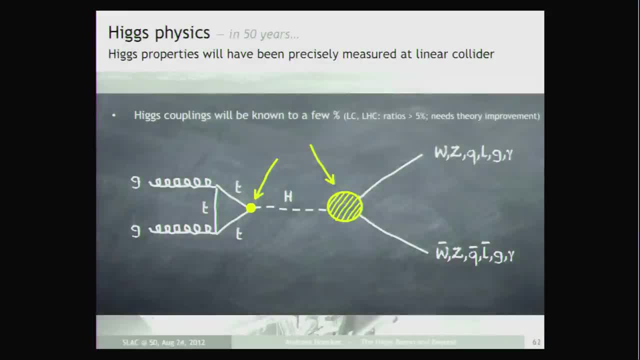 Of course the Higgs couplings here will have been measured to percent accuracy. We also need theory improvements here to be able to really exploit this fully. New heavy particles may couple to the Higgs and modify these couplings- an interesting scenario, of course. 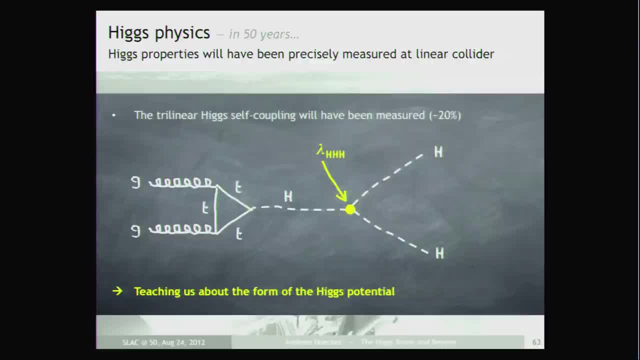 We have to measure the self-coupling of the Higgs, so the Higgs coupling going into two Higgs's. This gives us a factor of 1,000 reduction cross-section in the LHC. It's a very hard measurement. 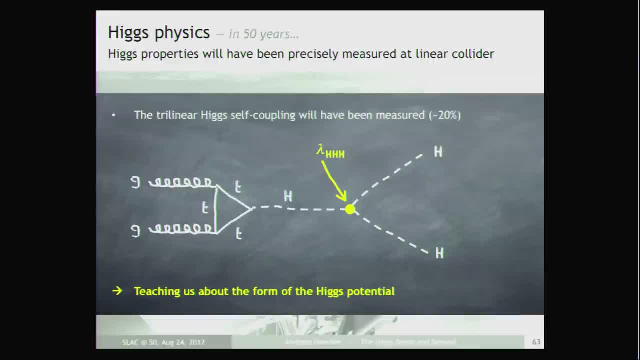 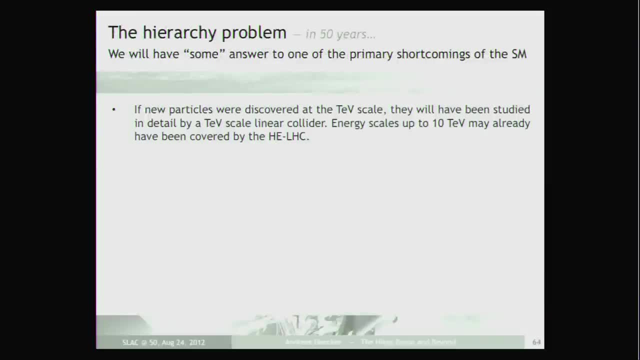 You need a lot of statistics for this, But of course this gives us directly access to the measurement of the Higgs potential. It's absolutely crucial to do this measurement, So if new particles were discovered at the TeV scale, they would have been studied in detail at the 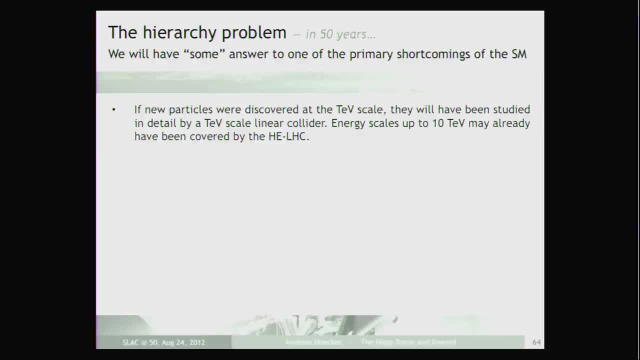 TeV linear collider And energies up to 10 TeV may already have been covered by the high-energy LHC. in 50 years from now, We will have learned and understood if the Higgs is fundamental regularized by new V couplings, for example. 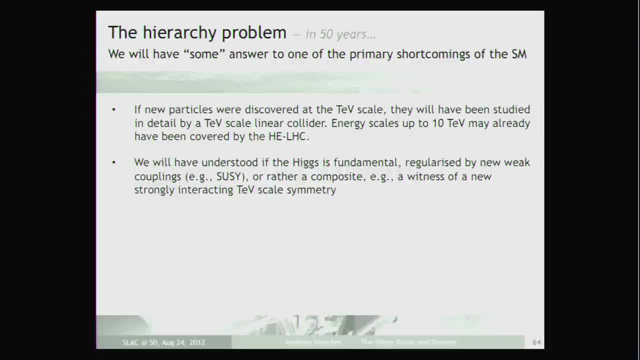 supersymmetry or other composite. we have an additional symmetry, at the TeV scale, for example, And the Higgs is then some kind of pseudo-Nambu-Goldstone boson. This, in any case, will be a revolution to our perception. 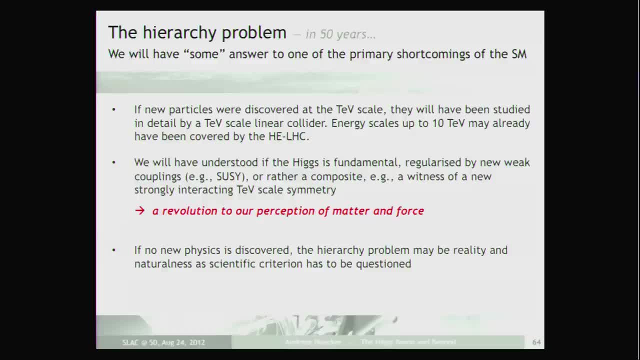 of matter and force. Now, if no new physics is discovered, the hierarchy problem may be reality, and naturalness as a scientific criterion has to be questioned In this case a revolution of thinking, physics, and possibly a hint to statistical choice of the universe's parameters. 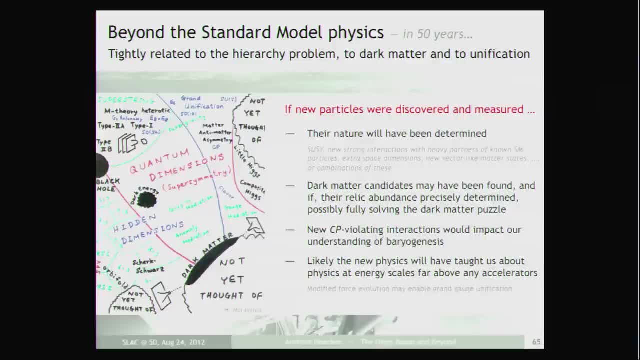 Now we also have to think about what will happen if we find new physics to all these beyond-the-standard models. And this is a picture of Hitoshi Murayama, who has put together the various models. And, of course, if we do see them, their nature will have. 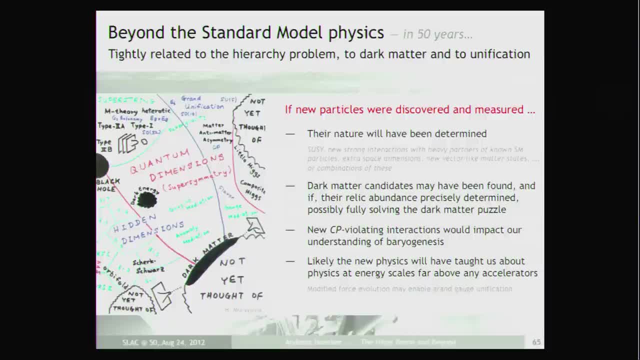 been determined at the linear collider Dark matter candidates may have been found and completely solved the dark matter puzzle. we currently have in the universe New CP violating interaction, so matter-anti-matter violating interaction would impact our understanding of baryogenesis, so the creation of matter in the universe. 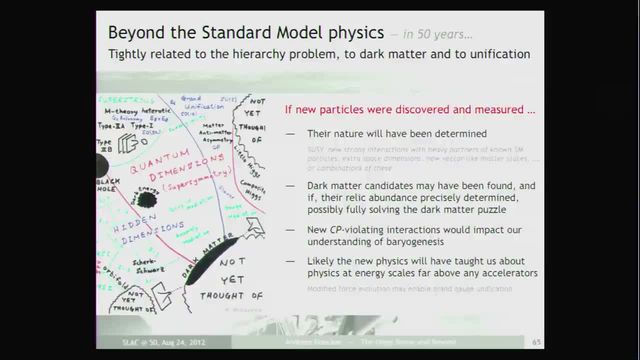 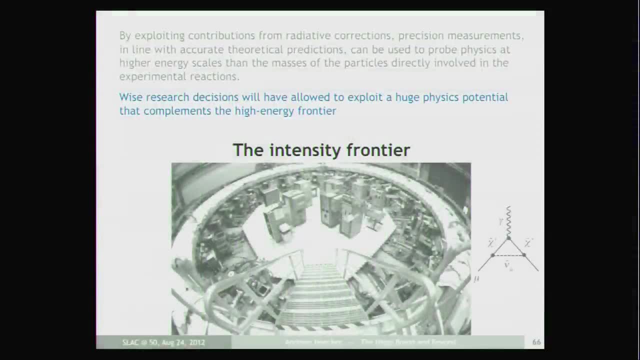 And likely the new physics will have taught us about the physics at energy scale far above any accelerators. Then I would like to briefly mention- also of course very important- the intensity frontier. Through Heisenberg's uncertainty relation we can. 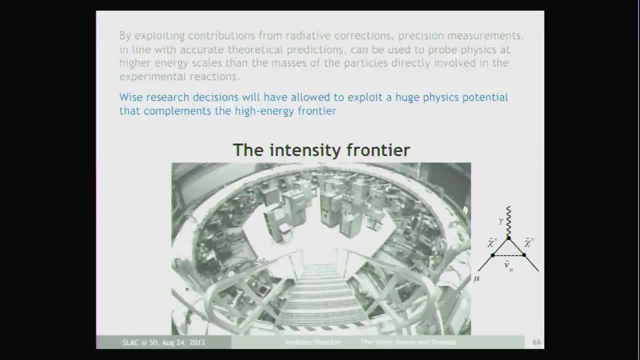 create particles which are much heavier than those we can directly create in our accelerators And we must exploit this. And wise research will have allowed to exploit a huge physics potential of this high intensity frontier. Now new techniques for the measurement of electric dipole. 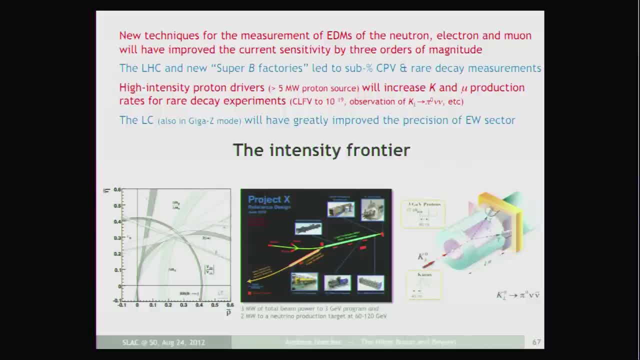 moments of neutrons, electrons and muons will have improved the current sensitivity by three orders of magnitude. That's absolutely astonishing and a real thing which can show us new physics in this area. The LHC and new B factories will lead to sub-percent CP violating and rare decay measurements. 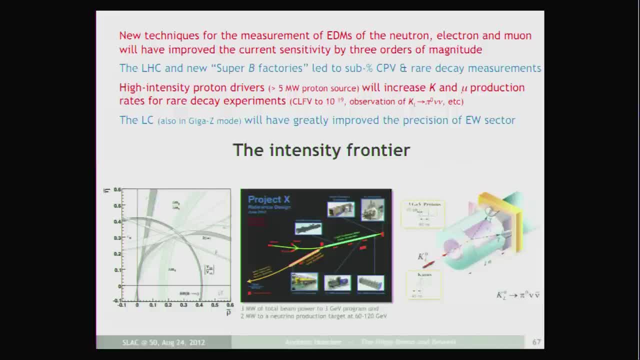 High intensity, The proton drivers. more than five megawatt proton source will create a huge amount of K and then muons to be able to study rare decays, For example. we can measure- that's really interesting- from mu to E conversion, the charge-electron flavor. 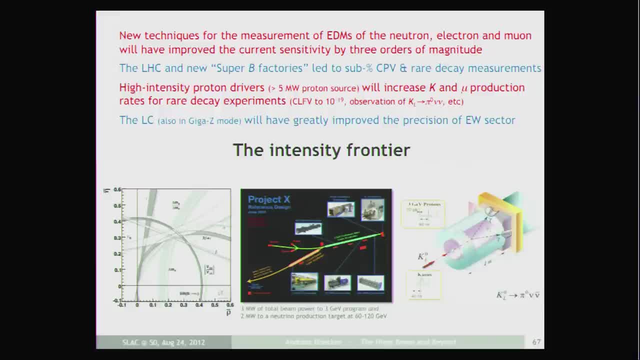 violation which is forbidden by extremely small in the standard model, not observably to 10 to minus 19,. with the absolutely true potential for discovery here. And also we can see, for example, this golden decay of K long to pi by 0 null bar, with a 10 to minus 11 branch. 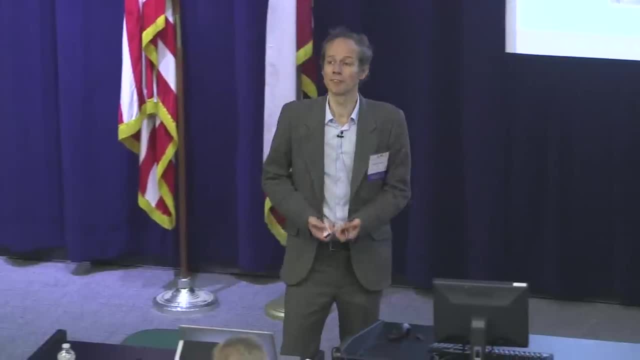 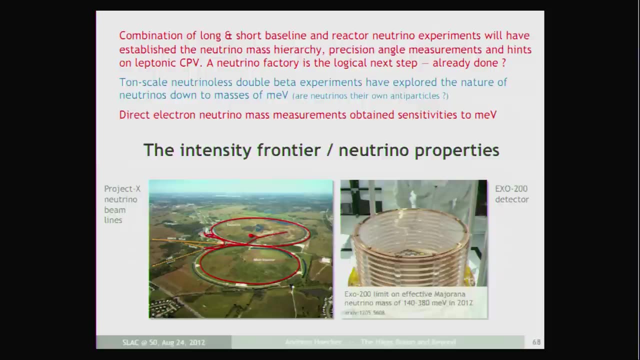 infraction. Of course, the linear collider will also then improve our precision. We can redo the electroweak fit and get lots of information about this. Then, of course, part of the intensity frontier is the neutrinos properties, And Fermilab has a very nice program. 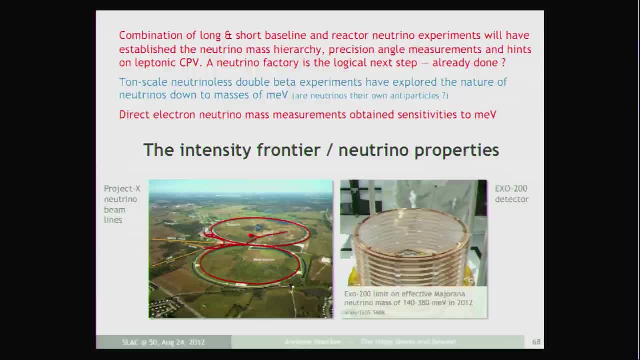 going through the various steps and ending up with a neutrino factory and then even going to a muon collider. That's really a very interesting program And the combination of long and short baseline and reactor neutrino experiments will have established the neutrino mass. 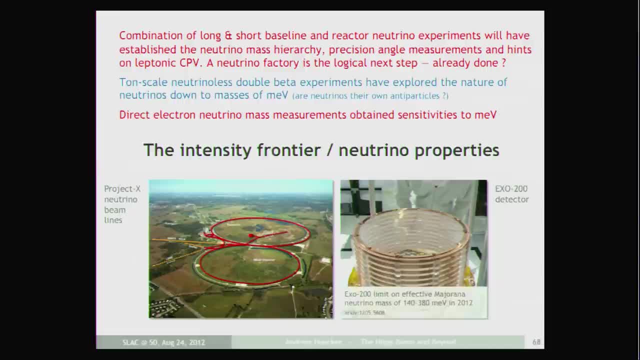 hierarchy, precision angle measurements and hints on leptonic CP violation, And then of course we can see that the neutrinos are systematically limited. So certainly the way to go is a neutrino factory is a logical next step, And maybe in 50 years I hope it's already done. 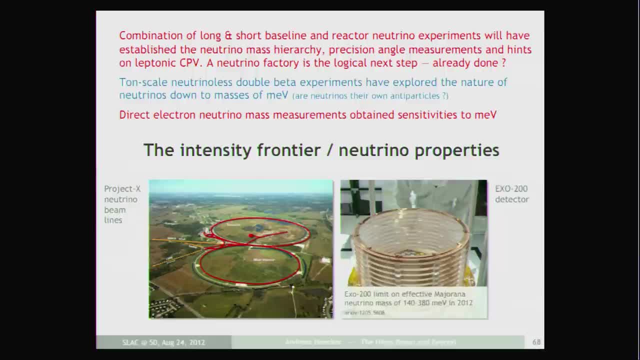 Tonscale neutrinos, as double beta decays, will have explored the nature of neutrinos. so, whether it's its own antiparticle or not, This is crucial to know whether we can use neutrinos to create leptogenesis and through leptogenesis, through. 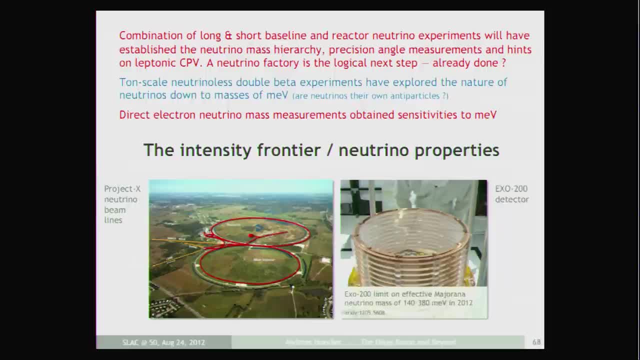 interesting processes produce bariogenesis. This is a very, very important thing, And for this we need to know whether neutrinos are Majorana particles or not, And we have also information on direct neutrino mass measurements. We will go up to milli-electron for these masses. 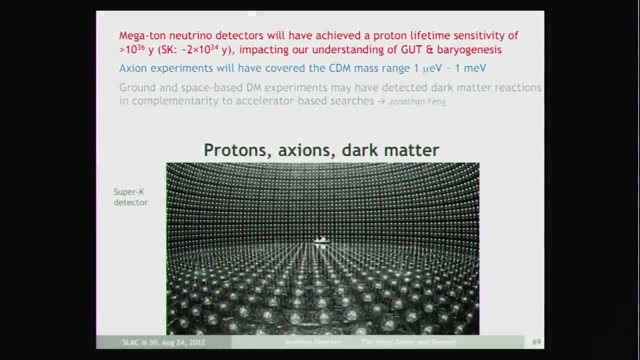 Finally, megaton neutrino detectors will have achieved a proton lifetime sensitivity larger than 10 to 36 years. Currently, we are from in Japan 2 times 10 to 34, impacting our understanding of unification. This is something I really want to emphasize. 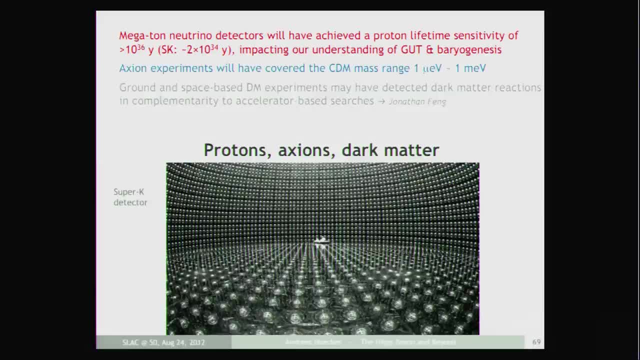 The fact that charges are quantized in protons- A proton is the same charge as the electrons. Our quark has 1 third of the charge of the electron- Must mean. Must mean that there is grand unification of electroweak and strong interactions. 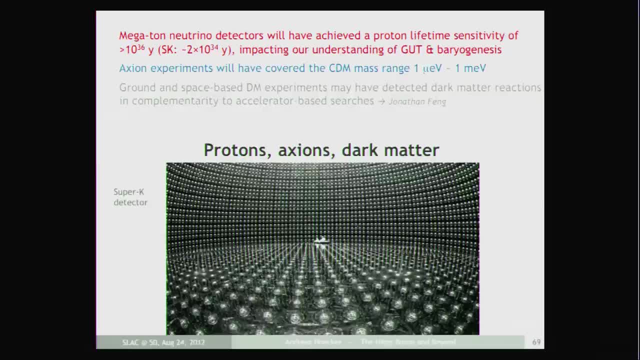 So we have to observe proton decay to be able to really. proton decay is a messenger of this grand unification. It's extremely important. Finally, axion experiments will have covered the cold dark matter range between 1 microelectron and 1 milli-electron. 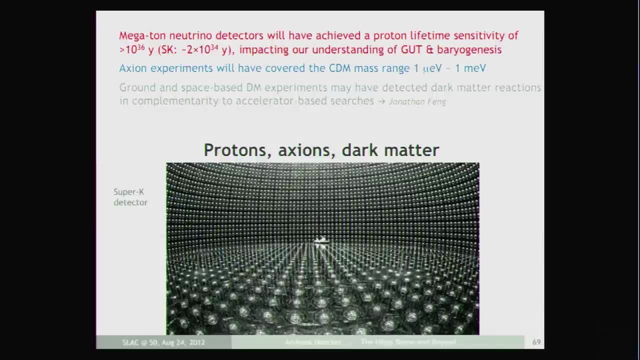 This is the most interesting range for axion to be able to be a cold dark matter candidate. And then there will be many, many experiments on direct detection of dark matter in space and on Earth, which will be discovered by Jonathan Fang later. Finally, the last point I have to mention, of course, theory. 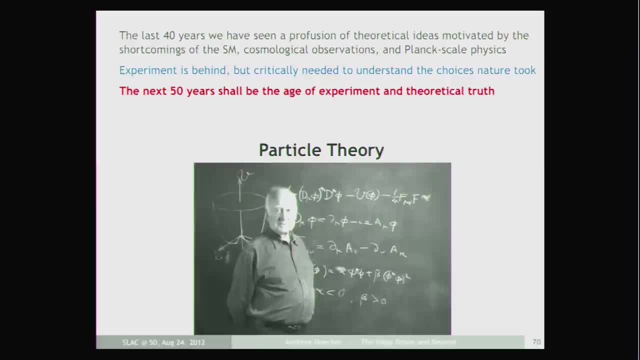 The last 40 years, we have seen a profusion of theoretical ideas motivated by the shortcomings of the standard model, by cosmological observations and by the Planck scale. physics Experiment is behind, far behind, but absolutely needed to understand the choices nature took. 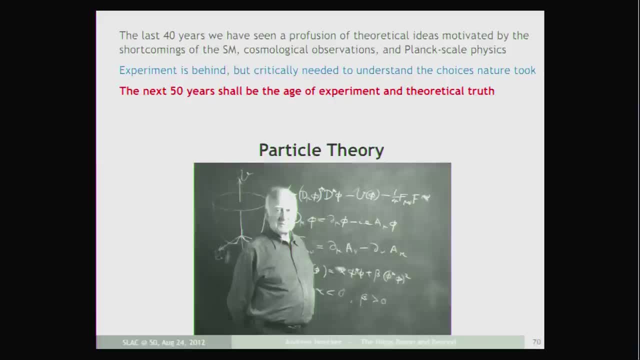 I have told you, super-stimulant is so elegant. it must be true. It could be that nature didn't choose it. So the next 50 years shall be the age of experiment and theoretical truth. And I would like to say I'm not going to be talking about the 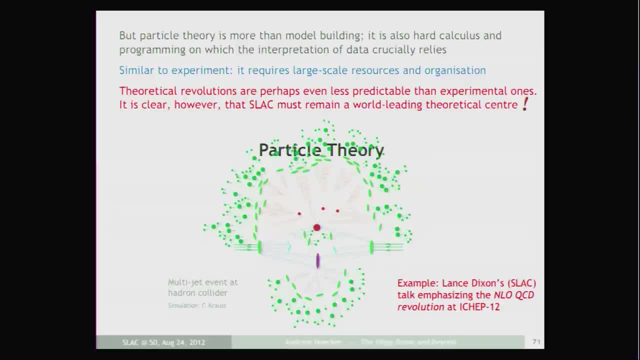 theory. I'd like to point out also that particle theory is more than just model building. It is also hard calculus and programming on which the interpretation of the data crucially relies. We cannot exploit, for example, the LHC without all the work. 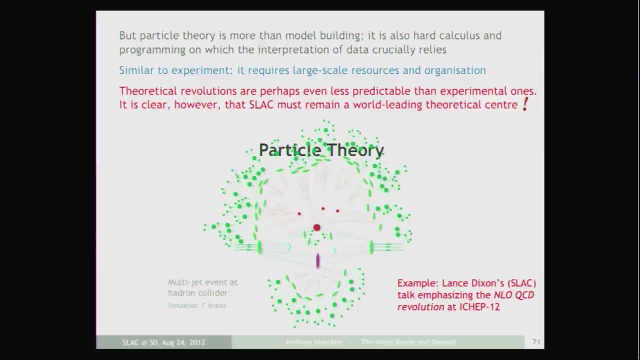 the theorists have done to do our predictions. There was a very, very nice talk by Lance Dixon on the NLO, next to leading all the QCD revolution at ICHEP, which you should look at And, of course, similar to experiment it requires. 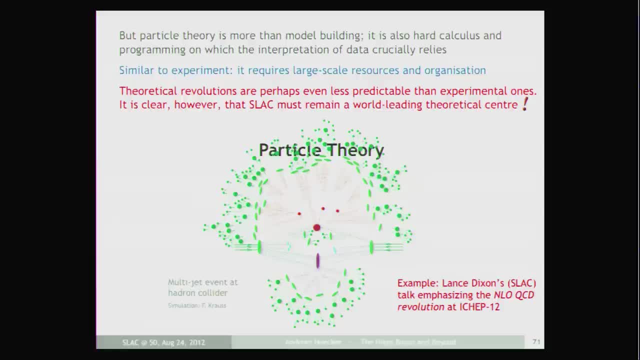 large-scale resources and organization. So theory in this way is getting more and more into also big organization, which is necessary to be able to do these calculations. So this is, for example, a proton-proton collision which you really have to calculate. 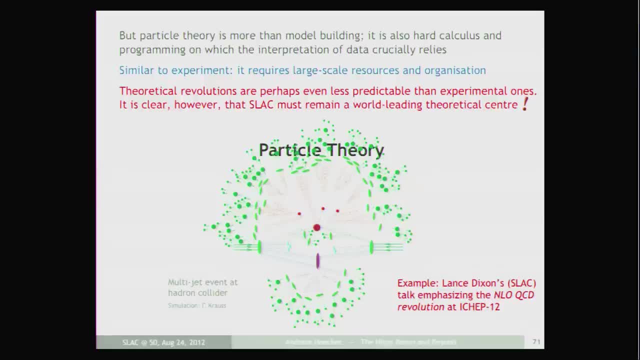 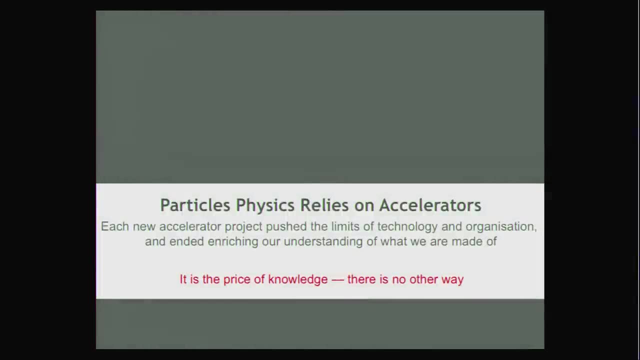 Theoretical revolutions are perhaps even less predictable than experimental ones. It's clear, however, that SLAC must remain a world-leading theoretical center, And although particle physics started by looking at the sky, at cosmic rays, and we get many, many ideas from cosmology and astrophysics, 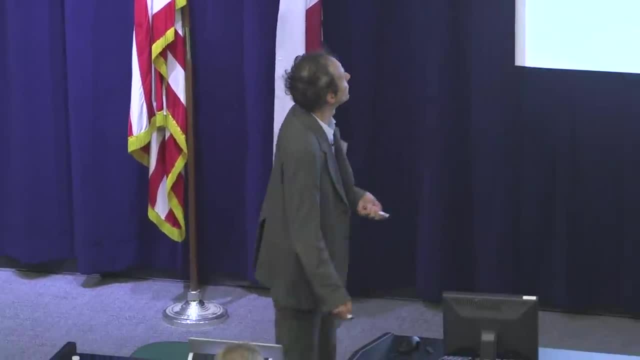 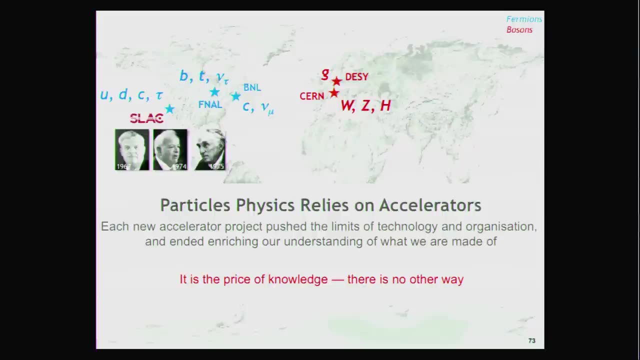 in the end, particle physics has to rely on accelerators And if you look back And the discoveries which were done, So this is for all the particles of the standard model. In particular, SLAC contributed, the UND quarks the Charm. 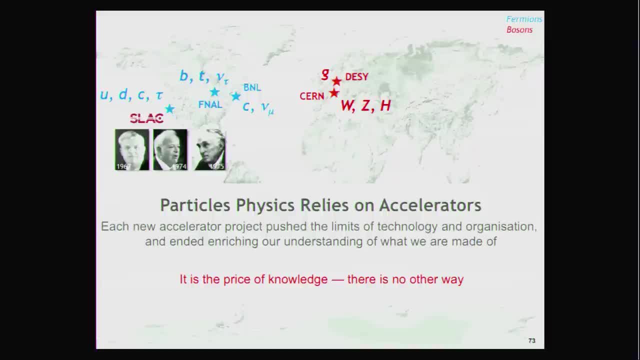 quarks and the Tau, with these eminent Nobel Prizes from there, And you see a nice asymmetry, which Young-Ki Kim also pointed out, between the material-oriented US and the interaction-oriented Europe. Certainly, each new accelerator project pushed the limits of technology and organization. 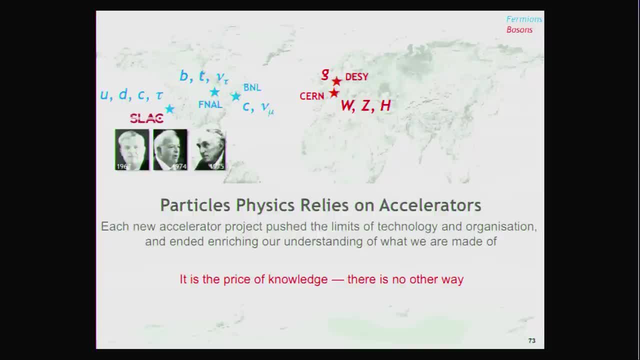 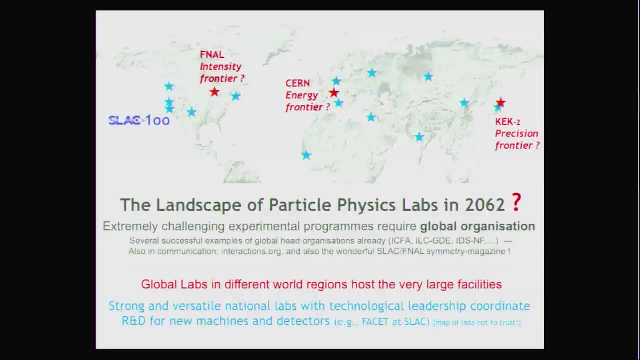 It ended enriching our understanding of what we were made of. It's the price of knowledge. There's absolutely no other way to get there. So if we want to try to build a landscape of particle physics labs in 2062, I'm going far too much what I actually should do. 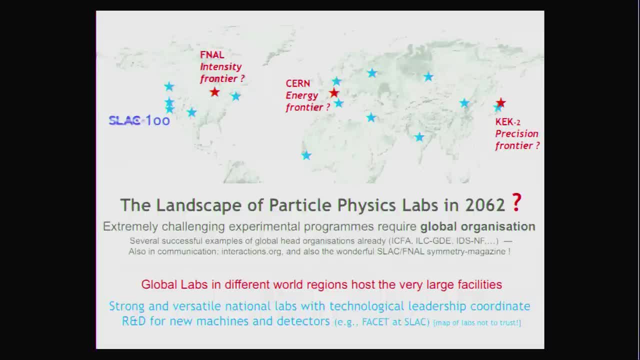 because I really have my nose in the data. But if we do this, we have an extremely challenging experimental program which requires global organization. We have several successful examples of global head organization, like ICVA, the global design effort. also the Nucino factory efforts. 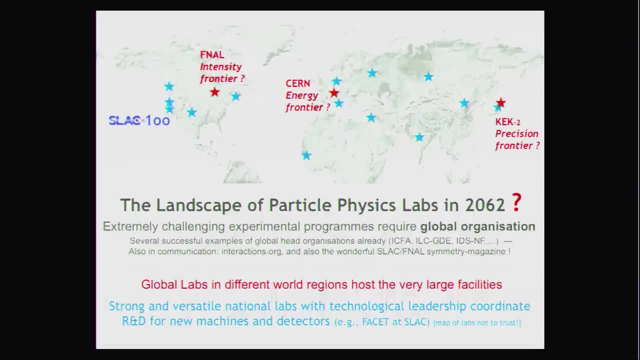 And also in communication. we have interactions like- I'm sure every particle physicist is subscribed to this very important source of information- Then the wonderful SLAC, FNAL Symmetry Magazine. And so we will have in 2062, probably, or hopefully. 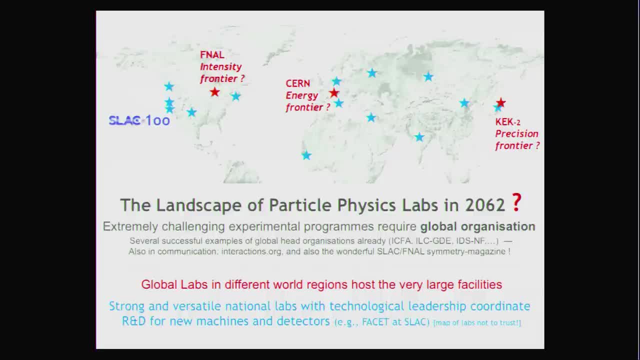 global labs in all the different world regions hosting the very large facilities, For example, intensity frontier at FNAL, at Sun, the energy frontier and Japan, a new site, the precision frontier plus or minus, for example. All the labs currently have various programs. 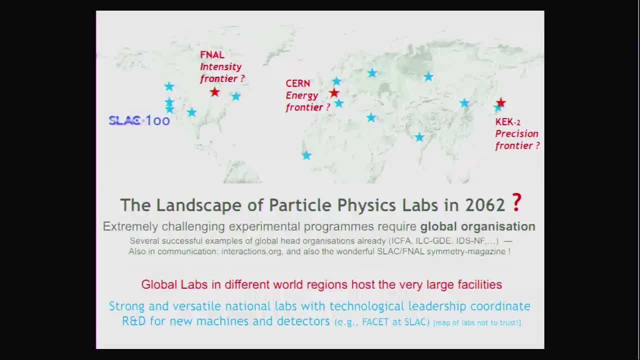 It could be the other way around, But this would be the best form of organization. We have to have in every region a huge lab which could make these facilities, And then we need strong and versatile national labs with technological leadership that coordinate the research and development for new machines and detectors. 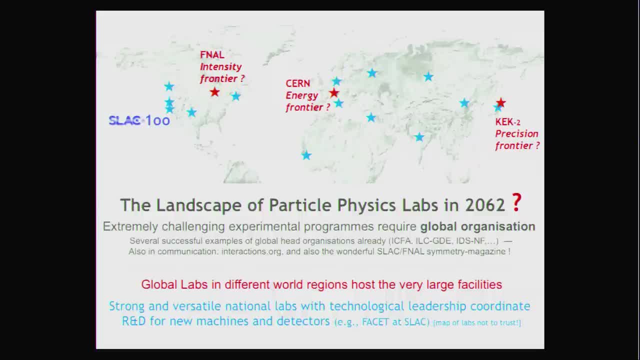 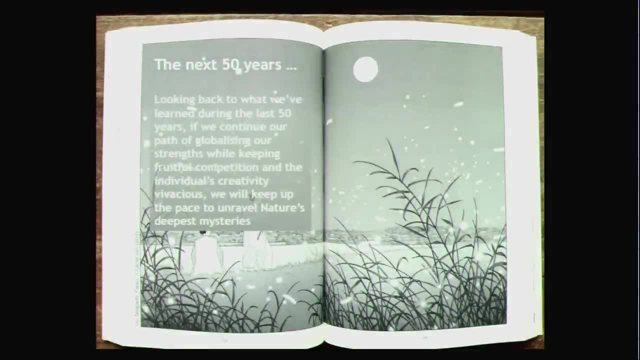 And faceted. SLAC is a very, very nice example of this, of course. So I will finalize here: The next 50 years. if we look back to what we've learned during the last 50 years, if we continue our path of globalizing our strength. 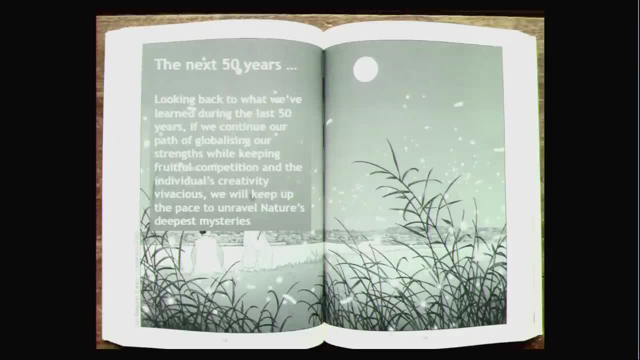 and keep fruitful communities. We will keep up the pace to unravel nature's deepest mystery And in 50 years from now there will be new particle physics. We will have emerged with new symmetries, new particles, new interactions that have extended the standard model. 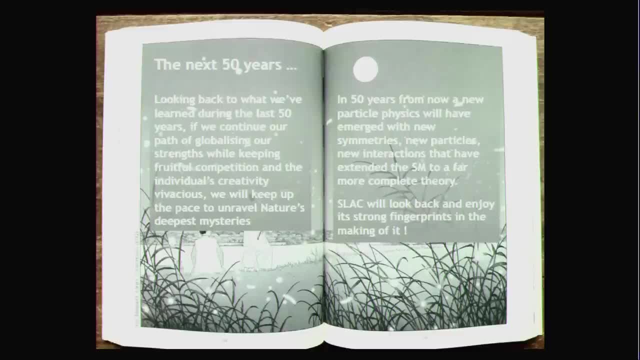 to a far more complete theory, And SLAC, in 50 years, will look back and enjoy its strong fingerprints on the making of it, as it does now on the making of the standard model, And I would like to congratulate SLAC for this achievement. 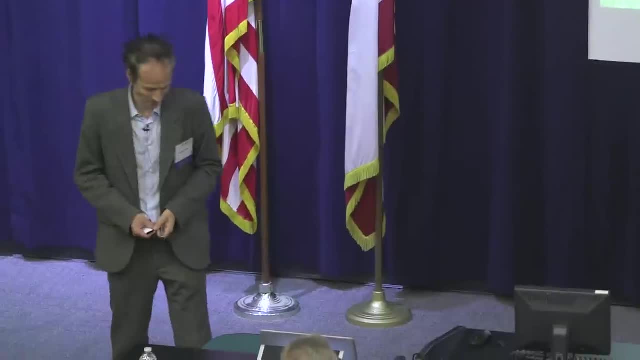 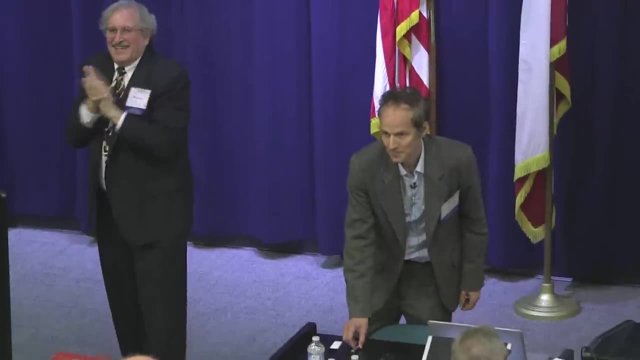 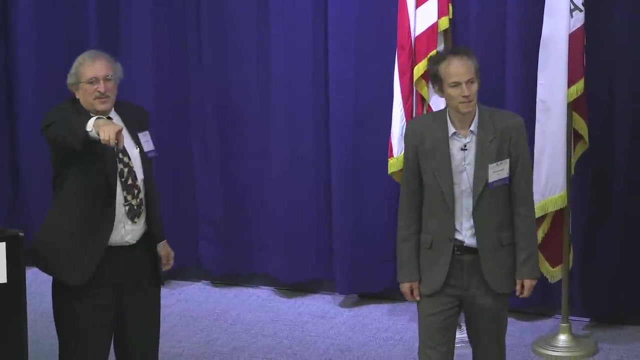 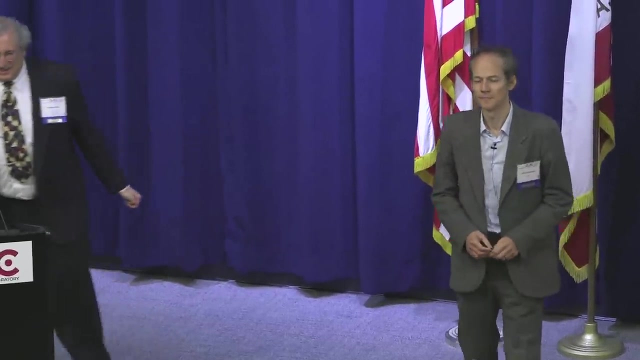 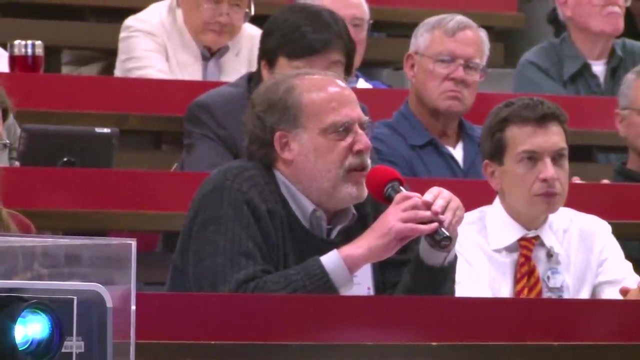 Thank you, Thank you, So we have time for a few questions. Please wait for the microphone. Excuse me. Most of the public presentations on July 4th and following referred to this. This is the discovery of a Higgs-like boson. 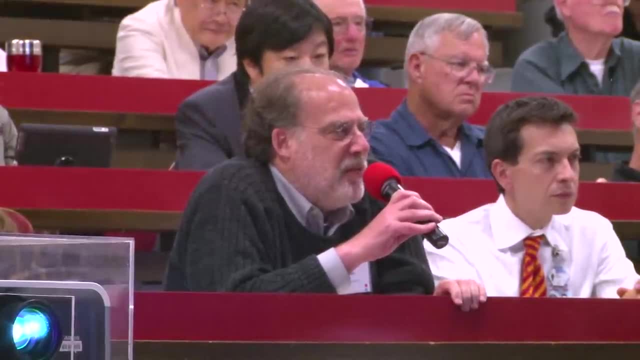 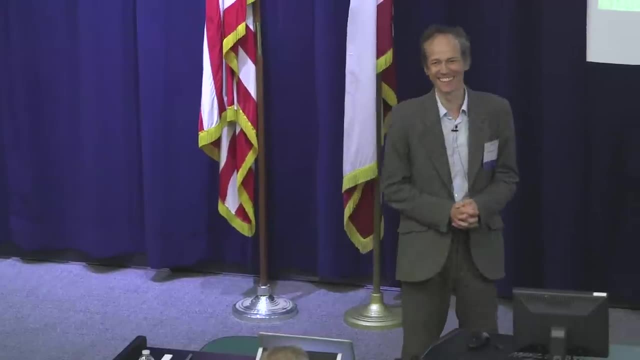 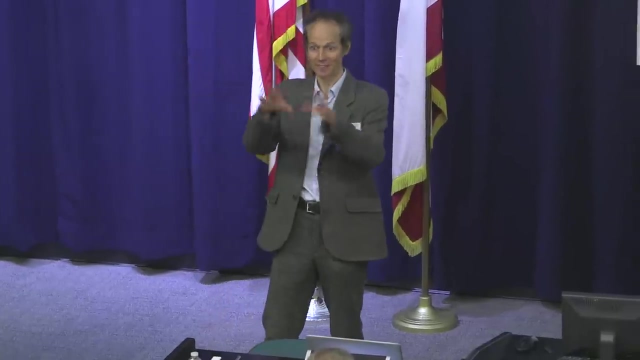 You've repeatedly referred to it as the discovery of the Higgs boson. Is there reason for your lack of caution? No, I think it is true. We should be prudent. So far, we have a boson which has, within the large uncertainties we have, 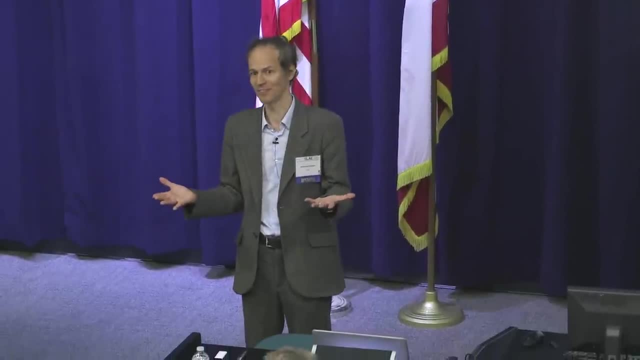 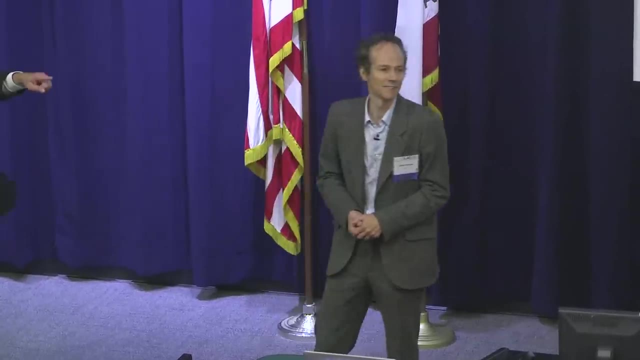 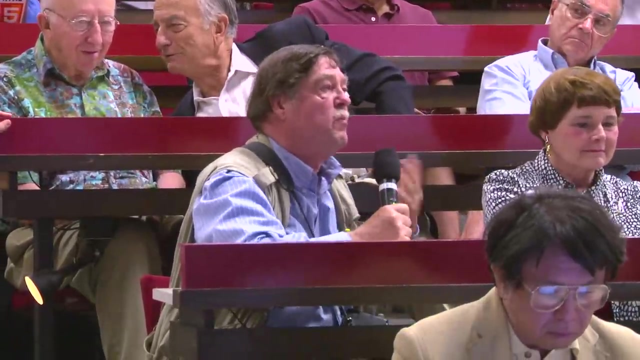 all the properties, it must have to be a real Higgs boson. So that's everything we can say for the moment. Thank you, Thank you, Thank you. Earlier, in your talk you likened the Higgs mechanism to superconductivity. 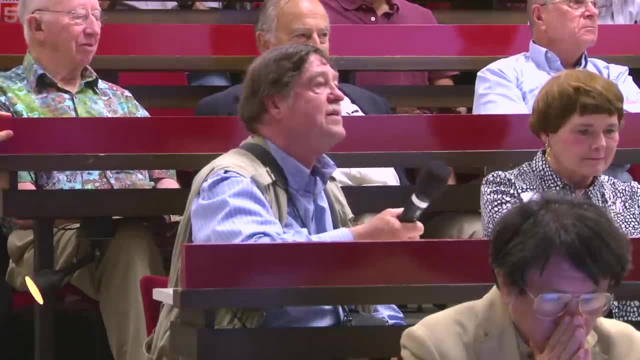 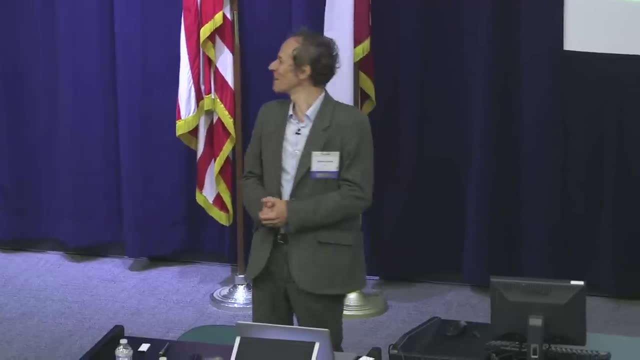 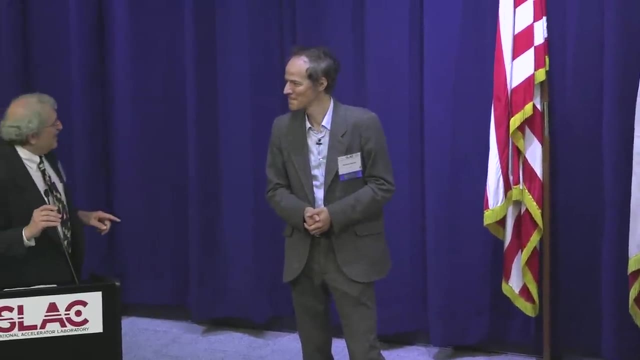 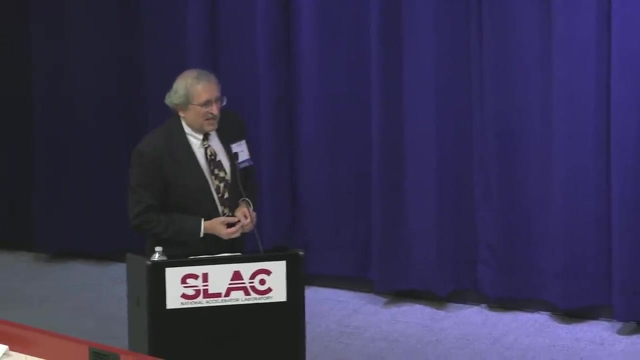 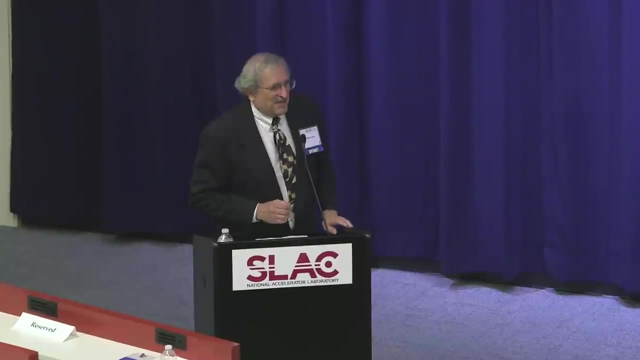 Could you expand on that a little bit? Is there a theorist who could maybe do this? If you turn this on, mathematically the Meissner effect in superconductivity is the same thing as what we call the Higgs mechanism in elementary particle physics. I can expand on that offline. 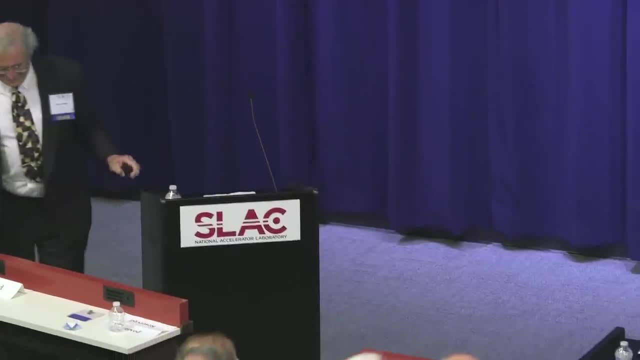 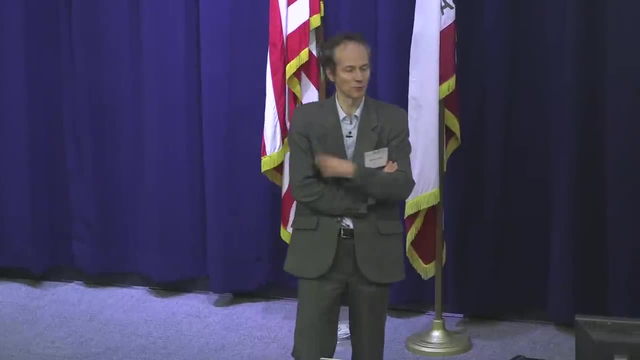 if you like, but that's the connection. Yeah, it's called the Anderson-Higgs mechanism And it's really, I mean, the original idea of the spontaneous symmetry wagon, really from Nambu- also came from superconductivity through the creation of the Cooper-Pairs. 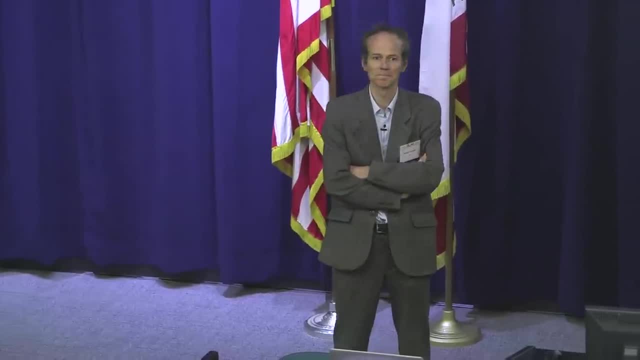 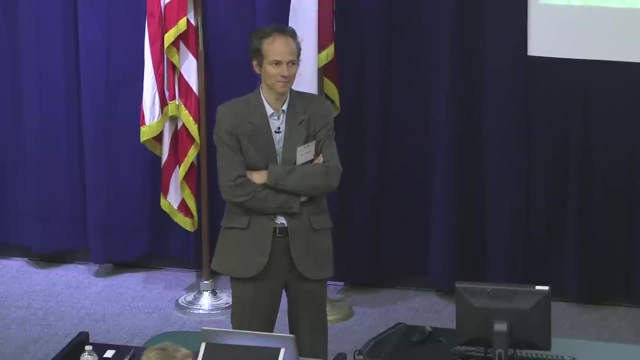 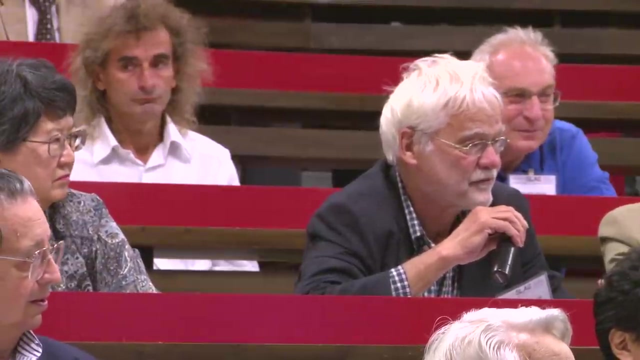 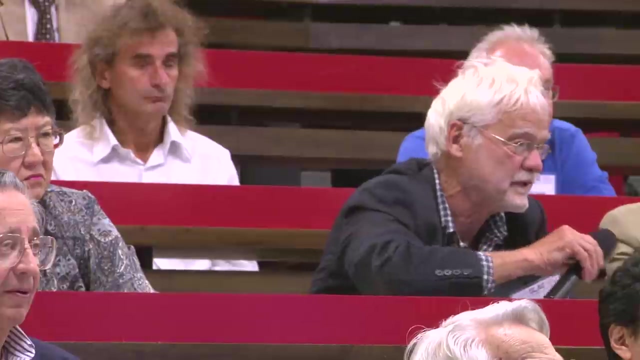 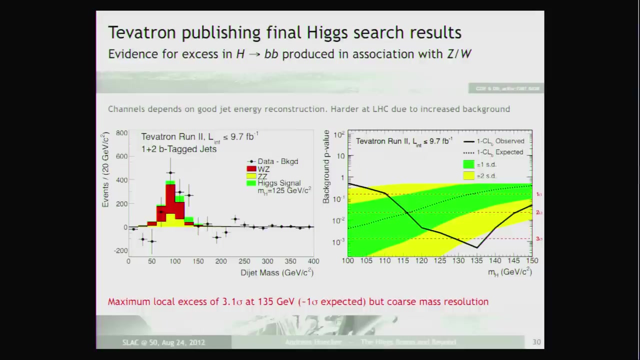 I wonder if you could show again the Tevatron data. It sort of was in a flash and I couldn't really see the error. There's a lot of evidence there. Maybe you should discuss it a little bit. So this is a subtracted plot which you see here. So all contribution from background. 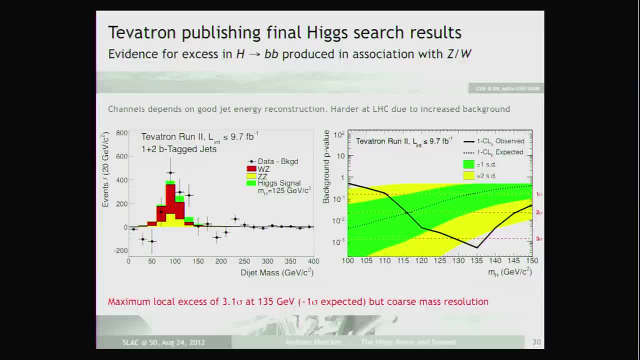 are subtracted. This is the die-jet mass. So you look into the creation of the Higgs to BB bar plus association of the W or Z- In this case I think it's the W- And you plot the invariant mass of the BB And you subtract all the backgrounds apart from W. 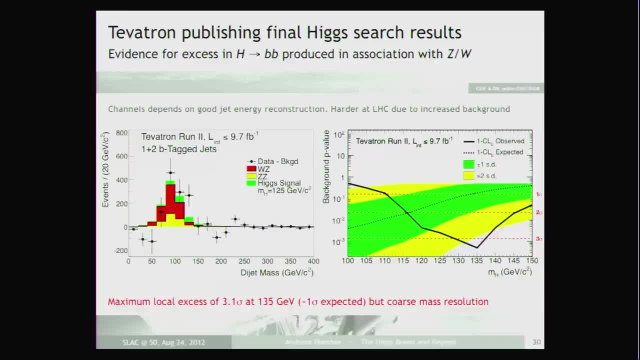 Z and Z, Z, And so there is a little excess here in this area. But what actually is done at the end is a full multivariate analysis which creates. So this is just a projection of all the information which goes in there, But the real result is a full multivariate. 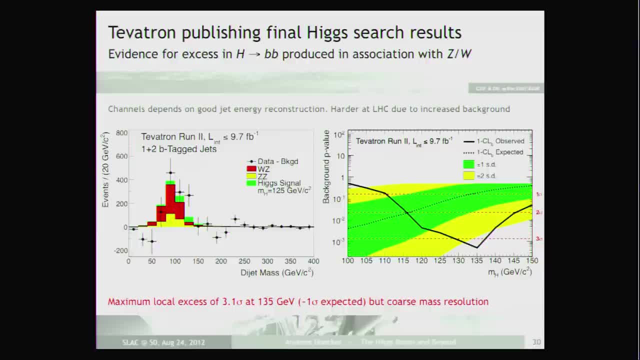 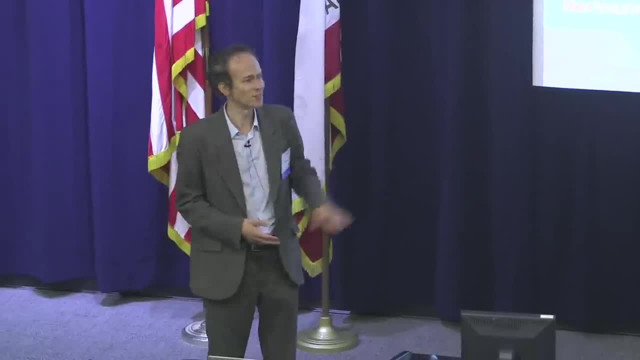 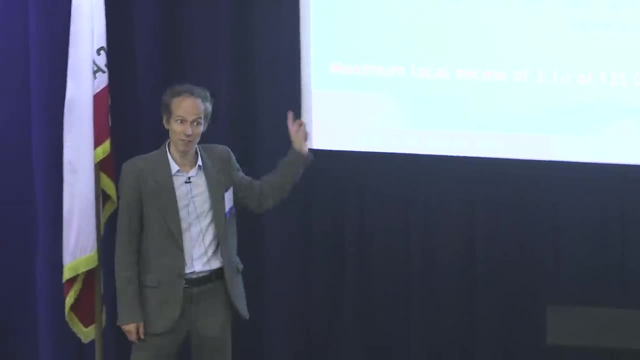 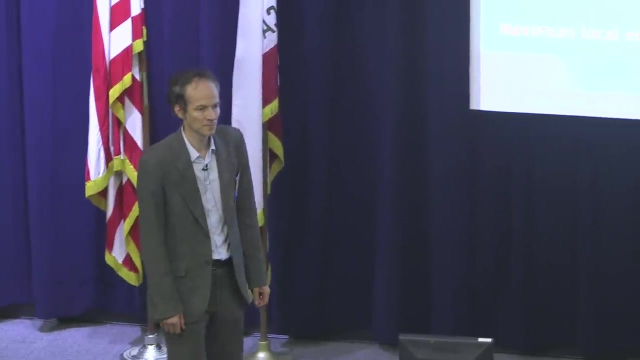 analysis which has a stronger discrimination than this one, than just the mass. So it's really very difficult to conclude from this on the actual power the teratron analysis has. It is much more than only this plot. Okay, One last question, Just a small comment with respect to this question. over here I noticed the Atlas paper.